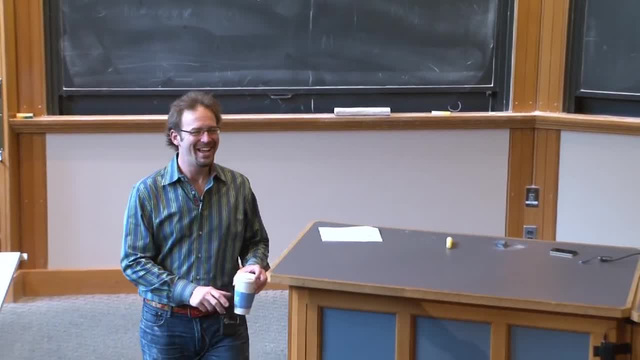 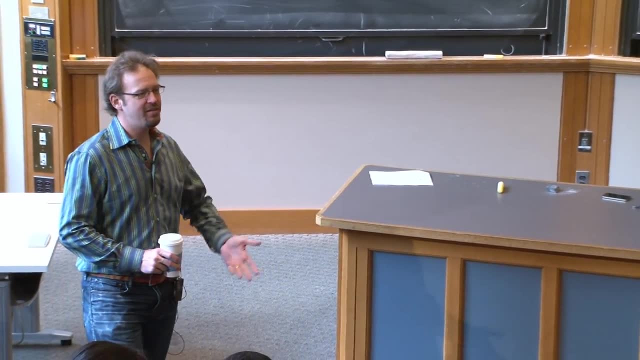 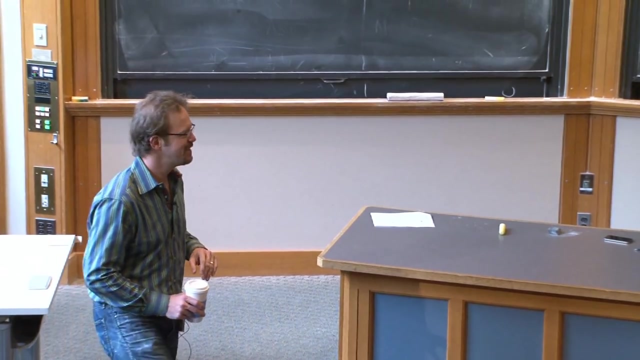 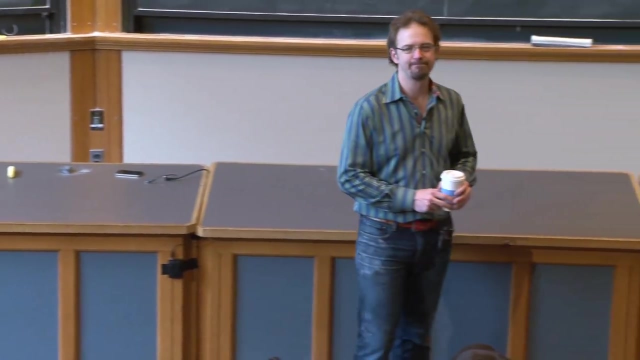 Hi everyone. Spring has regressed, So we're going to have a guest at the end of lecture today, which should be kind of entertaining, just as a warning if you see someone come in. So questions before we get started. No questions about anything at all. 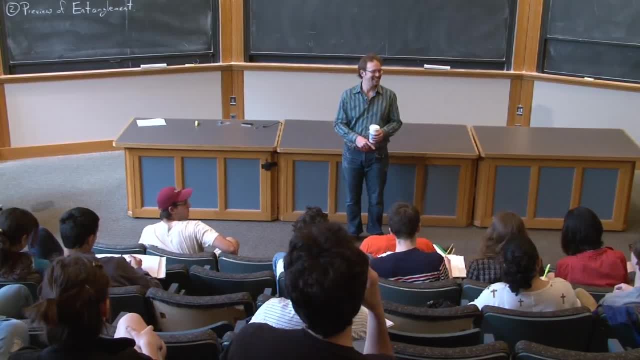 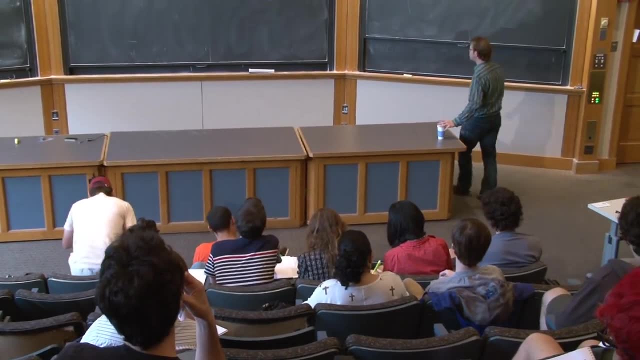 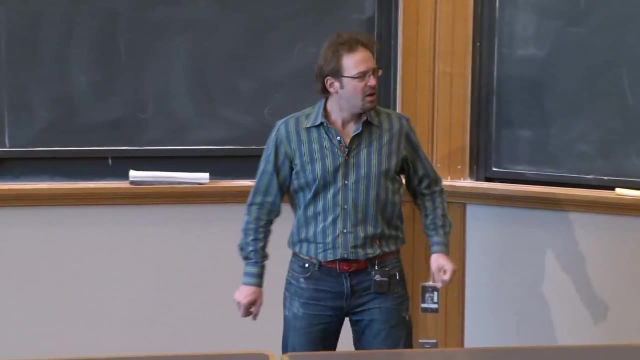 Max, Nothing. Yeah, Can you explain the physical significance of the crystal momentum? Yeah, OK, Let me go over that. That's a good question. So the question is: what again, is the significance of the crystal momentum? So let me answer that in a slightly backward way. 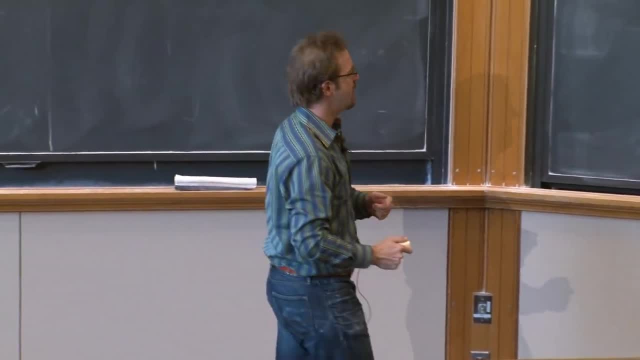 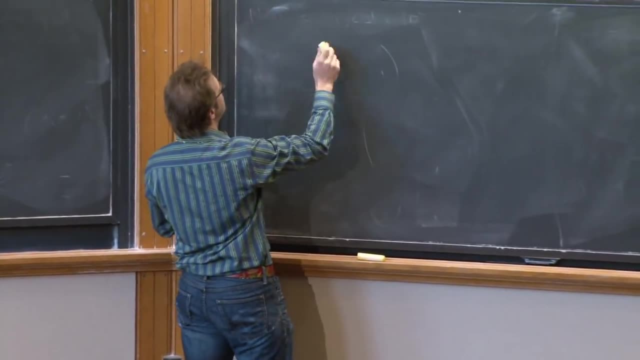 So this is a form of the explanation I haven't given you. It's going to be a slightly different one. Let's step back and think about the momentum and ask what the momentum is. Now. you guys showed on a problem set the following fact: 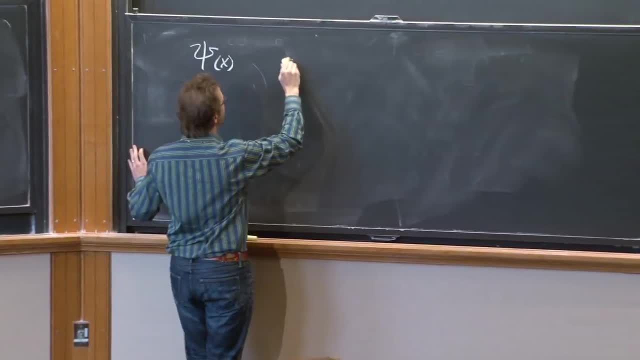 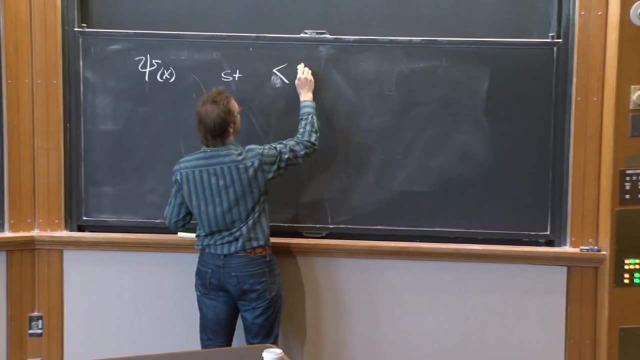 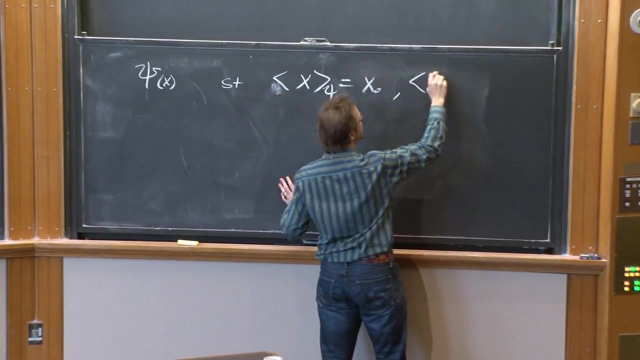 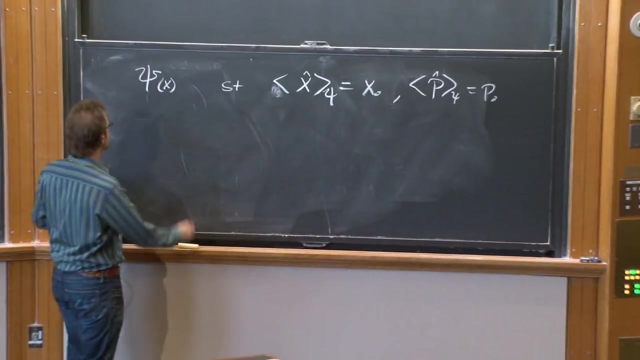 that if you have a wave function psi of x such that the expectation value in the state psi of x in the state psi is equal to x0, and the expectation value of p in the state psi is p0, hat hat. then if you want to change that, 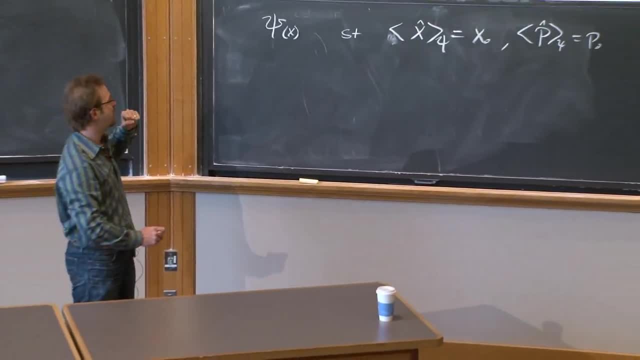 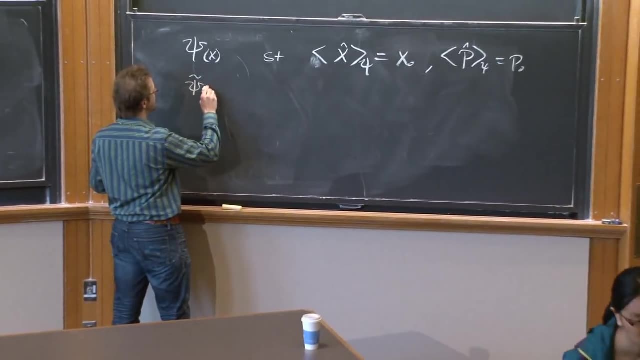 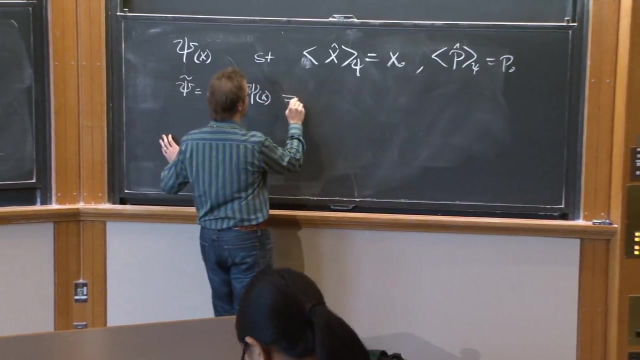 If you want to change the momentum, increase the momentum by h bar k. the way to do that is to take psi and build a new wave function. psi tilde is equal to e, to the ikx psi of x And then the expectation value of x. 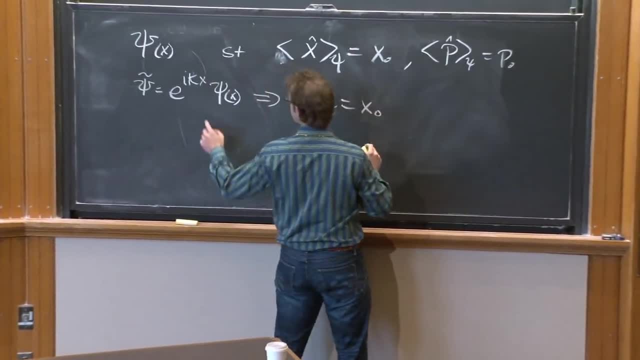 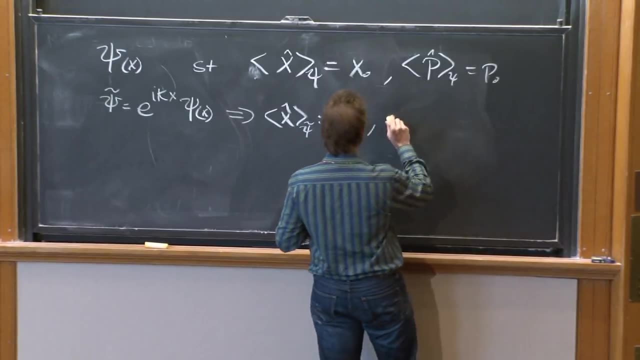 is the same psi tilde still equal to x0, because this phase goes away from the wave function as a complex conjugate when you take the inner product, But the expectation value of the momentum is shifted in the state psi tilde. 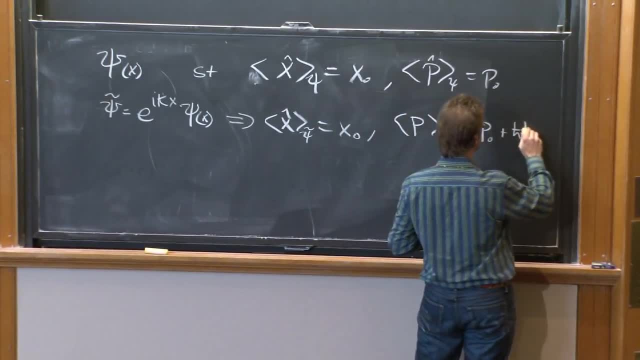 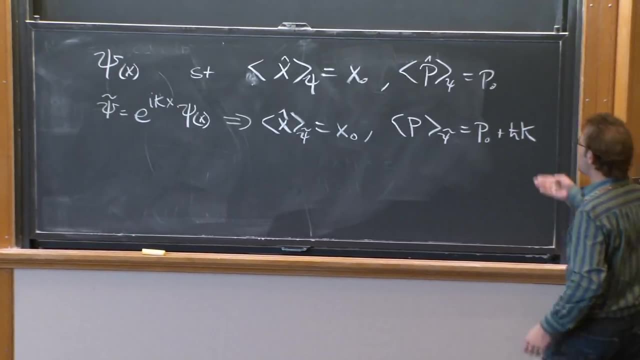 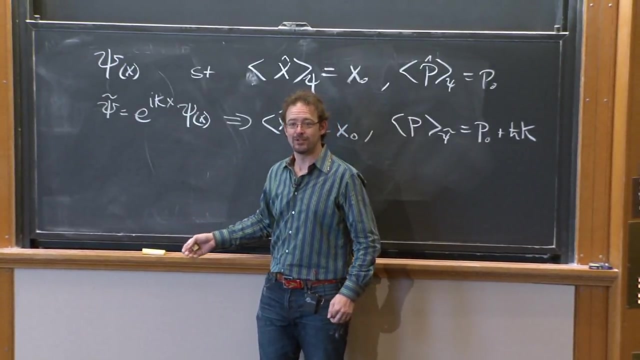 is shifted by h bar k, p0 plus h bar k. So all the intuition you have about momentum you can translate into intuition about the spatial variation of the phase of the wave function. Yeah, I have another question. Oh, OK, good, 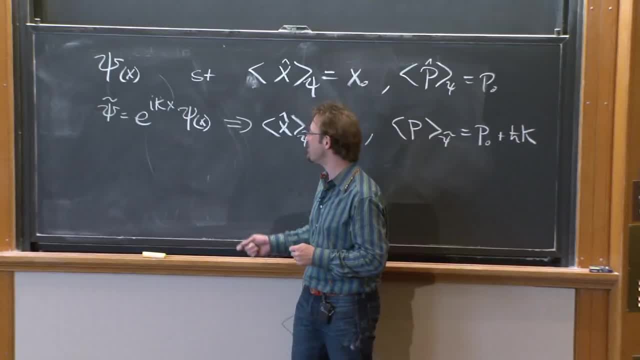 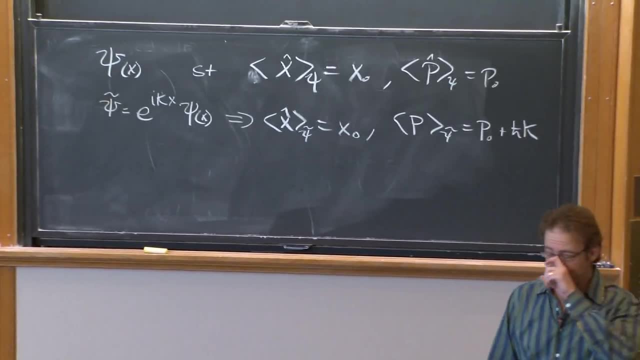 OK, good, good, good. So we have a sneaky recitation structure today. So, Um, So the information about the momentum can be encoded in the spatial variation of the phase of the wave function, So another way to answer the question then. 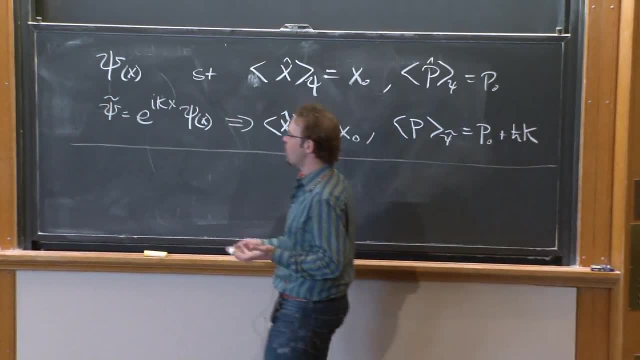 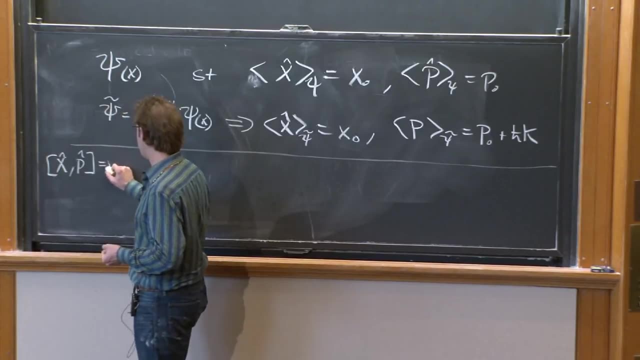 of what is momentum apart from it's the thing that. So what are ways to answer the question? what is momentum? You could ask. well, what is momentum? It's the thing that commutes with x by ih bar. That's one way to answer it. 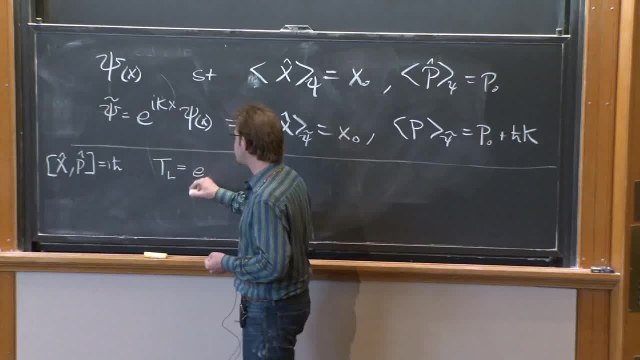 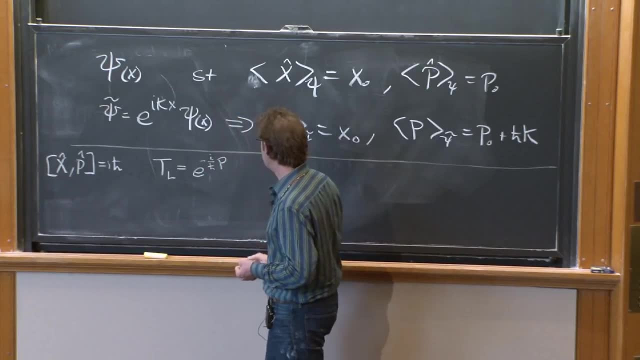 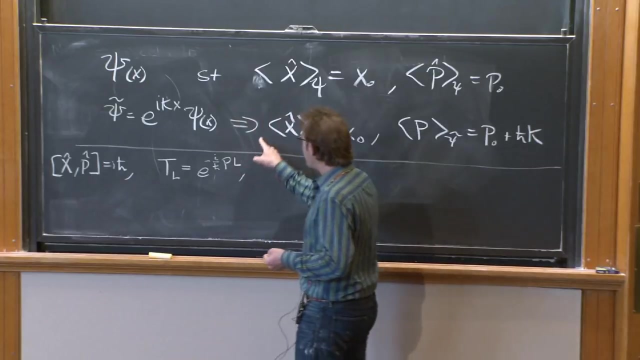 Another way to answer it is to say that translations by L can be expressed in terms of momentum, as e to the minus i upon h, bar h, bar p, L. OK, So these are both ways of describing what the momentum is, But another way of talking about the momentum. 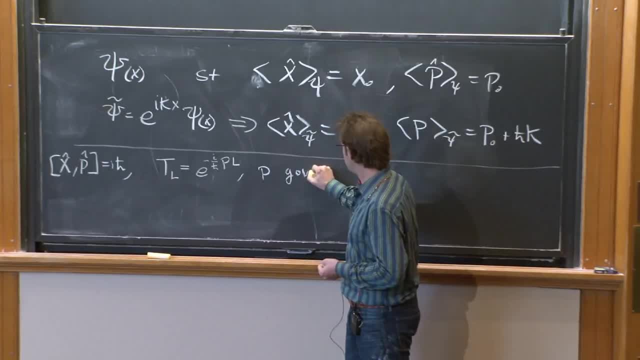 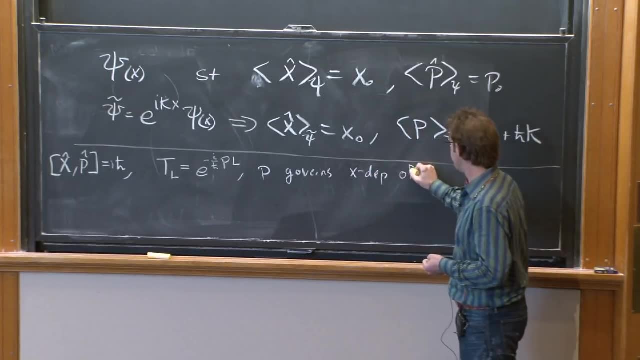 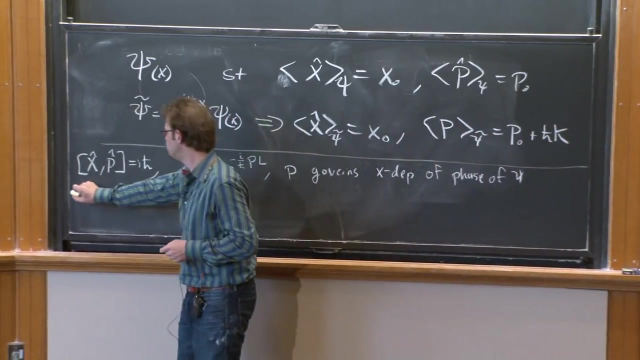 is the momentum. p governs the spatial variation, the x dependence of the phase of the wave function of psi. OK, So these are all ways of talking about what the momentum is. So now let's turn this around and let's 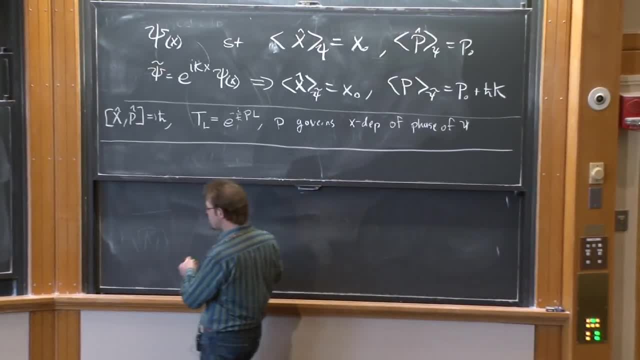 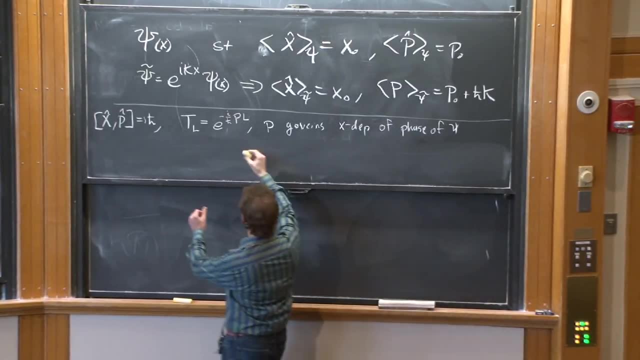 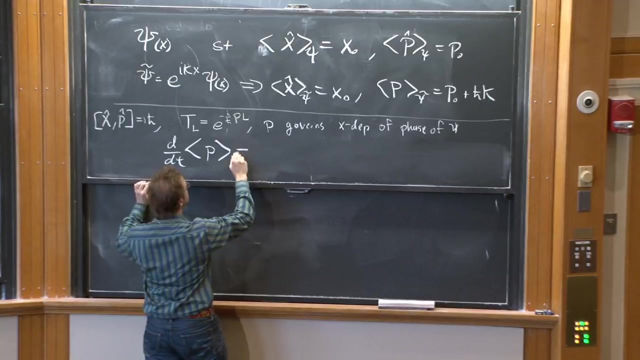 ask about the crystal momentum. Oh, and one last thing, a last defining property of the momentum, a central property from the Schrodinger equation, is that the time variation d, dt of p is equal to the expectation value of minus d. 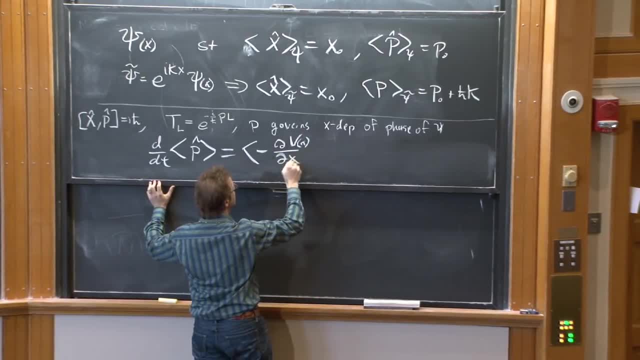 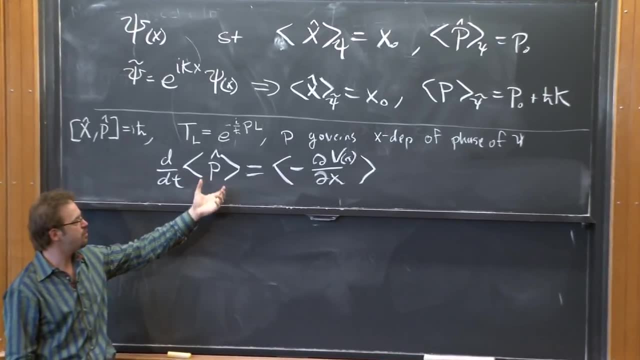 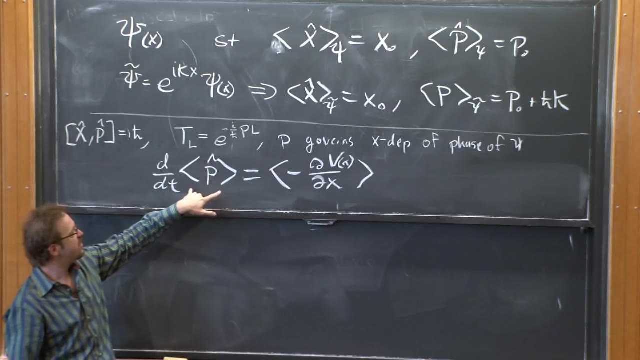 the potential of x, dx, also known as the force Right. So this is the Ehrenfest's theorem statement that the classical equation of motion, p, dot, is equal to minus, dv, dx or minus is equal to the force. Ehrenfest's theorem tells us that the classical equations 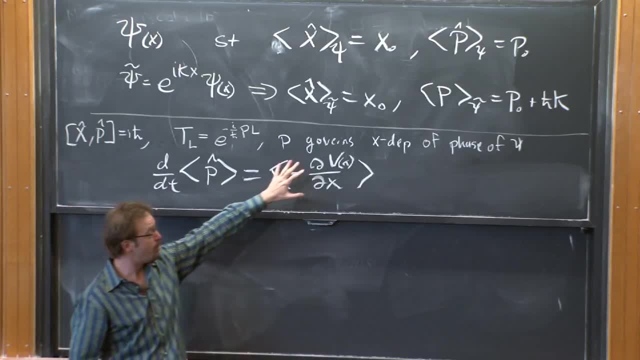 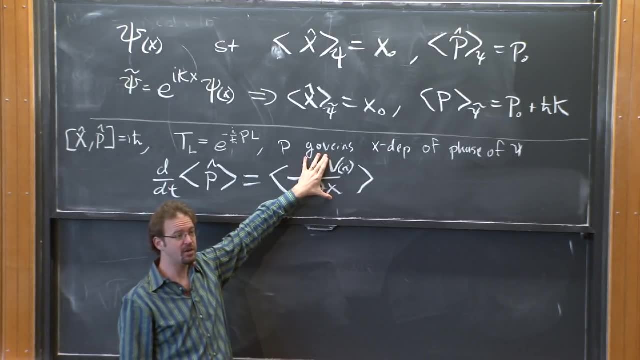 of motion are realized as expectation values And equivalently, if there's no potential, if the potential is constant, this tells us that the momentum expectation value is time, independent Right, A familiar fact. So these are all true, lovely and things about the. 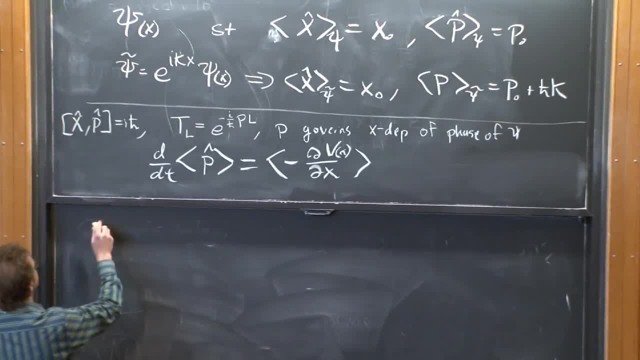 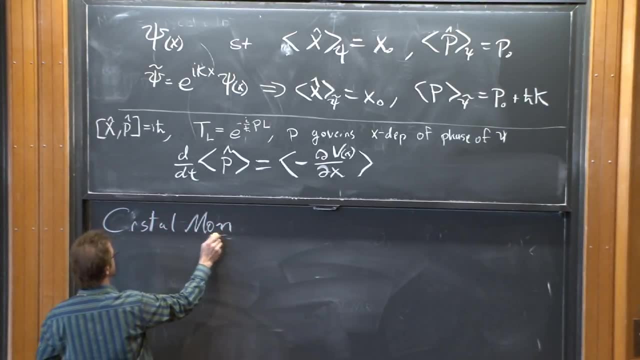 momentum. So let's turn all of these facts around into the crystal momentum. So let's talk about crystal momentum, which was the question. what is the crystal momentum? So the crystal momentum is defined from the beginning from the following property: If we have a potential v of x, which 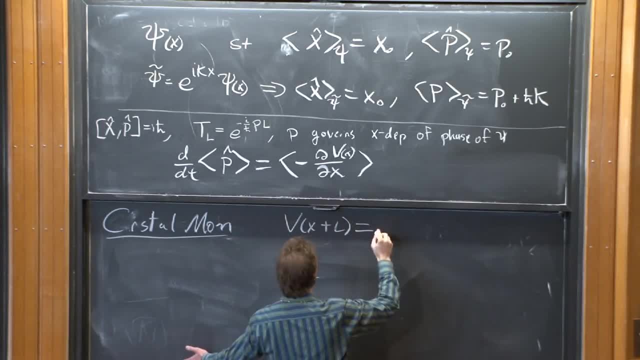 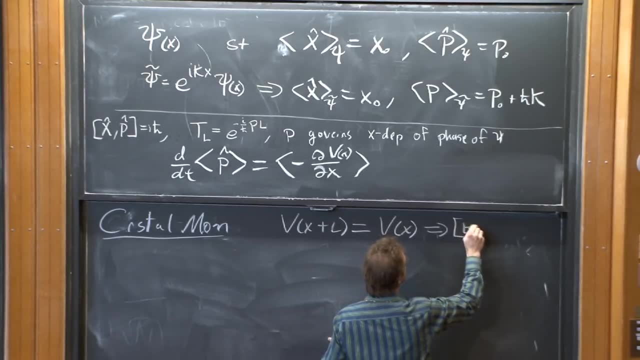 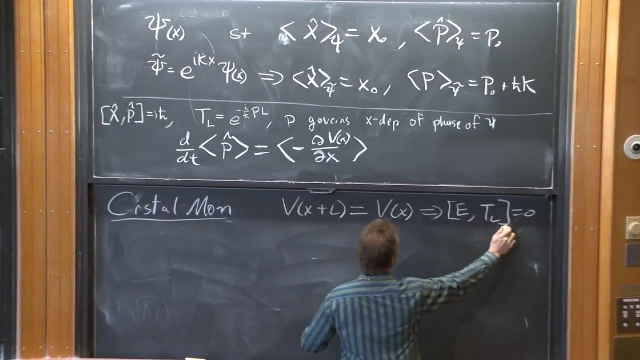 is invariant. under shifting by one lattice, spacing by some L, this is v of x. then this tells us that the energy operator is invariant if we shift by L. if we translate by, L equals 0. And from this fact we deduced via block or a la bloc: 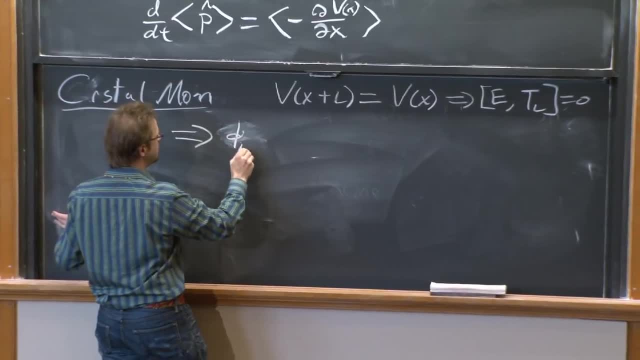 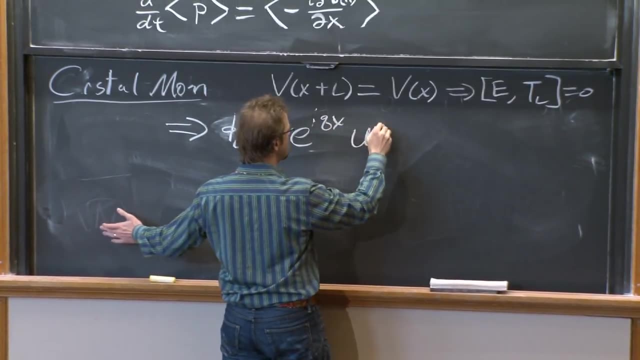 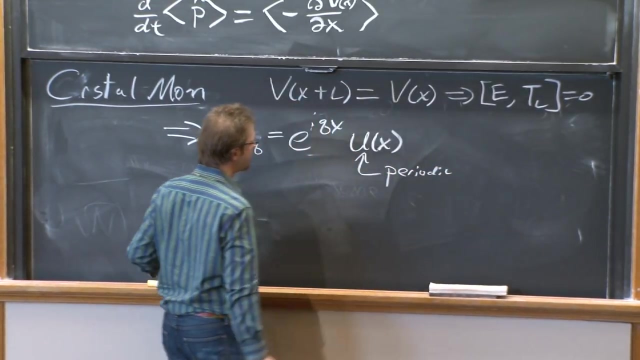 that the wave functions, or really the energy eigenfunctions, can be written in the form: eq is equal to e, to the iqx u of x, where u we're going to take to be a periodic function. So what does this parameter q do? 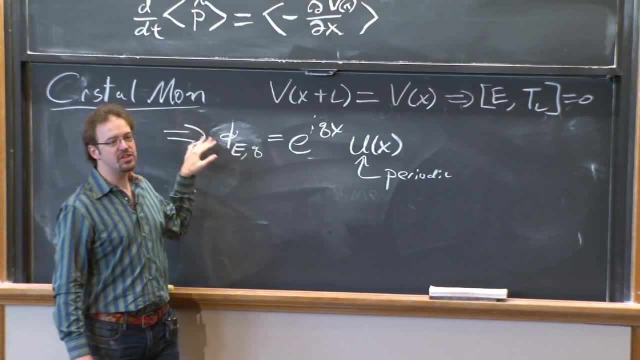 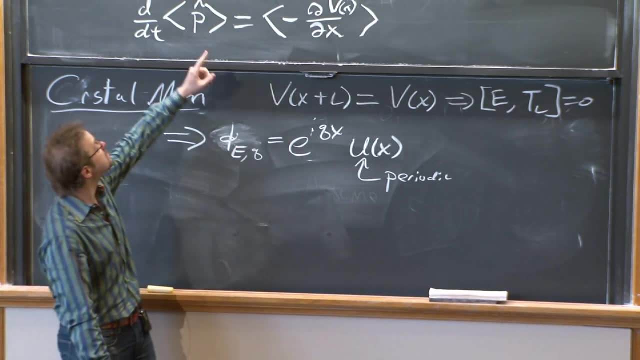 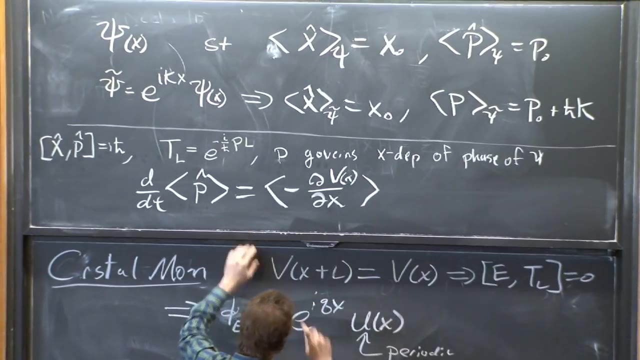 What does it do? What it's doing? q is governing the spatial variation of the phase of the wave function: Cool. So, in precisely this sense, in precisely this sense that the momentum governs the space of the wave function. here, in the case of a periodic potential, 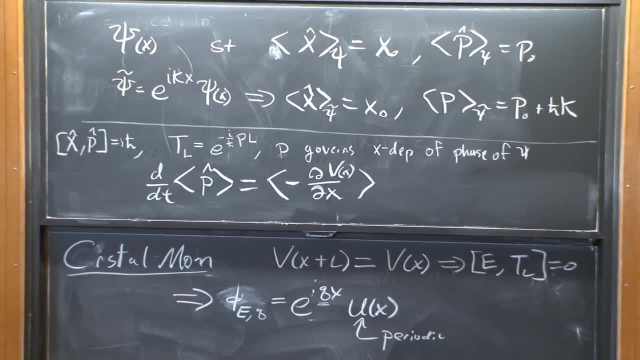 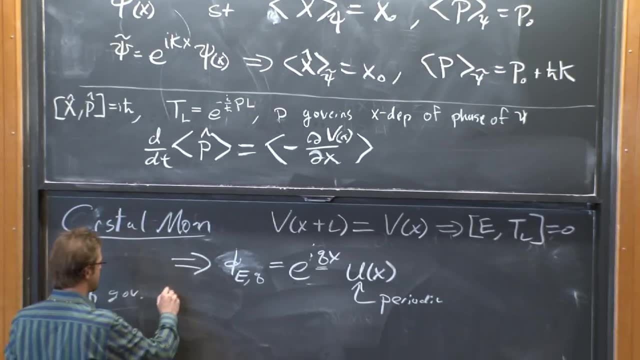 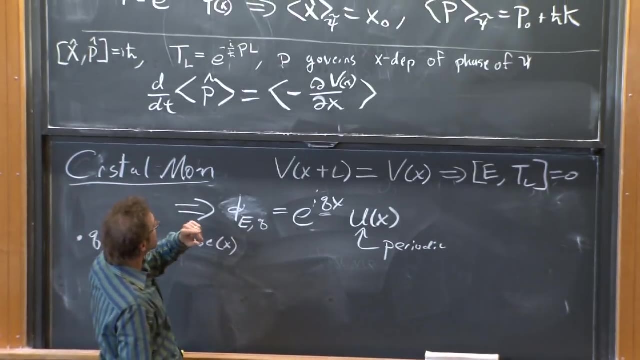 the crystal momentum, q is governing the spatial variation of the phase of the wave function. So q is the thing that governs the phase. So it's the function of x, It's the function of x. Well, what about another fact about the crystal momentum? 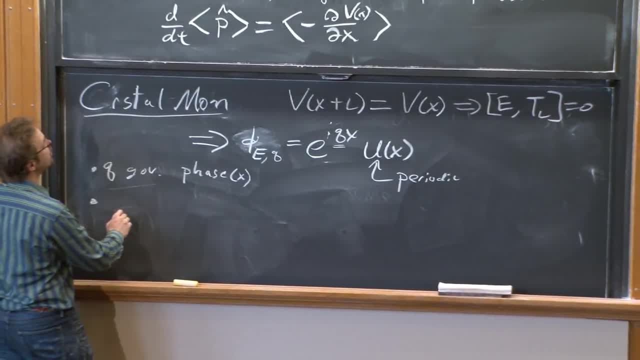 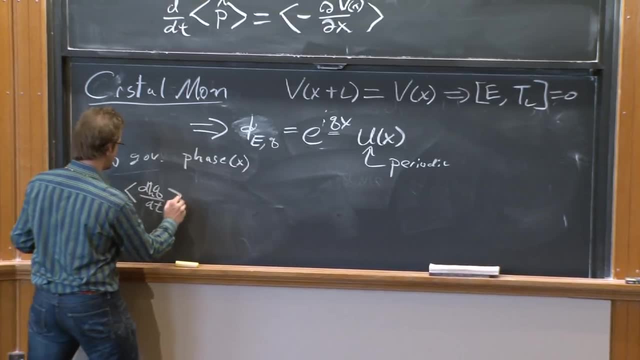 which you show in your problem set is that if you impose an external force, dq, dt and really d, h bar q, dt is equal to d dt of the expectation. It's equal to d dt of the expectation that q is equal to d dt. 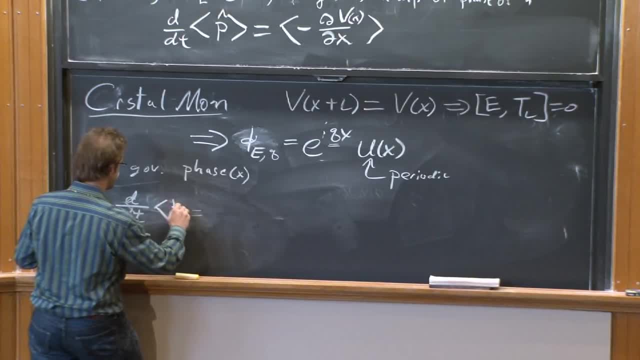 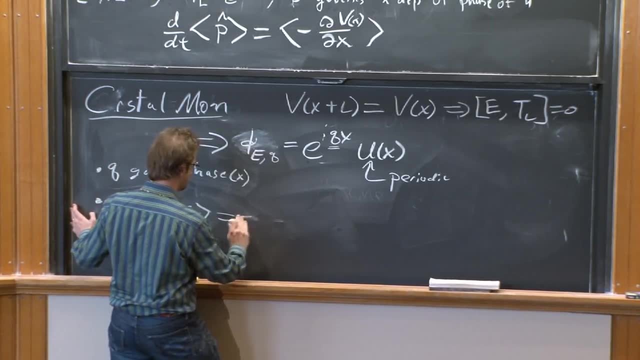 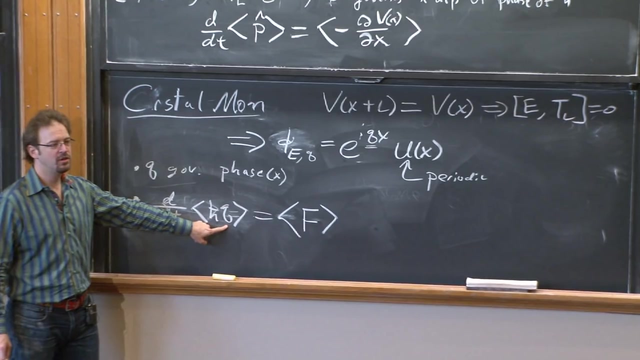 So what does this mean? It's equal to d dt expectation value of h bar q is equal to minus the expectation value of the force. I'll just write So again, this is a quantity, and this was assuming that we had a sharply peaked wave packet. 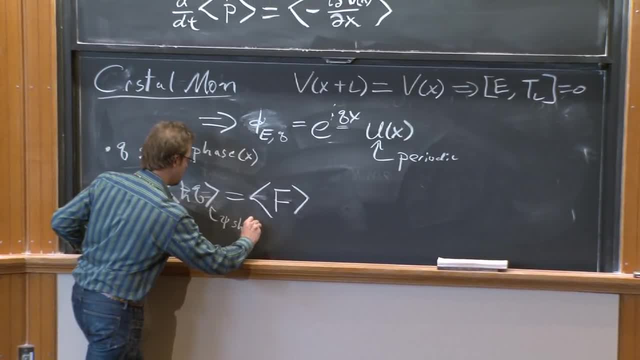 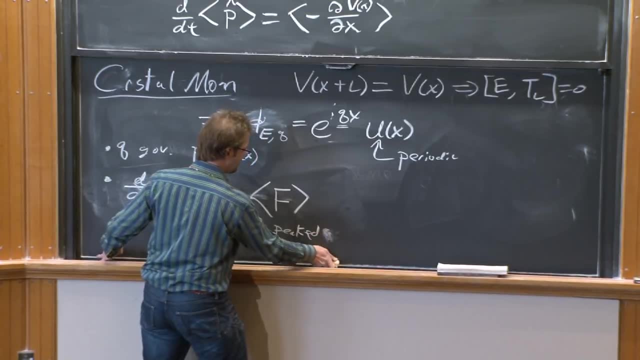 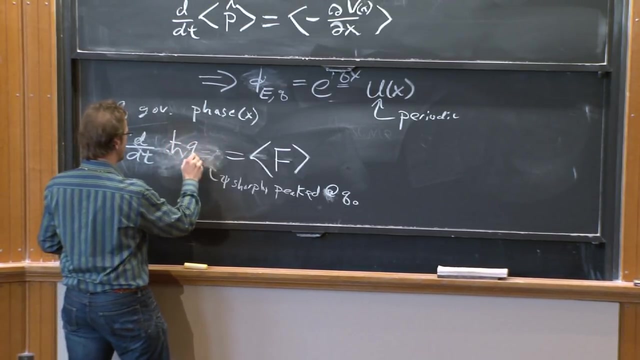 So this is for a wave packet sharply peaked at q0. And so then let me just write this as h bar q0.. So the central value of your wave packet. so this is what you show on the problem set that the central value of your wave packet, the peak 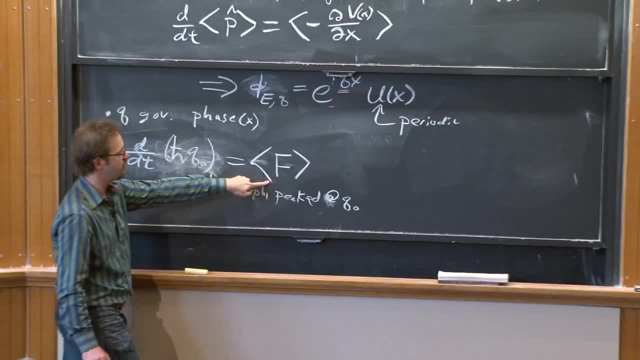 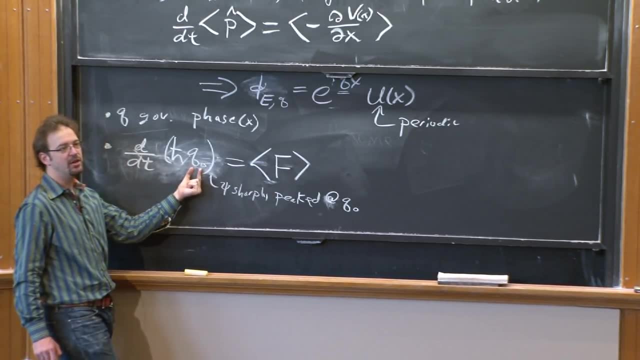 of your wave packet varies in time according to the external force, And so, in particular, if the force is 0, if we turn on no external driving force, your wave packet maintains its crystal momentum. It's time independent, So the crystal momentum is something. 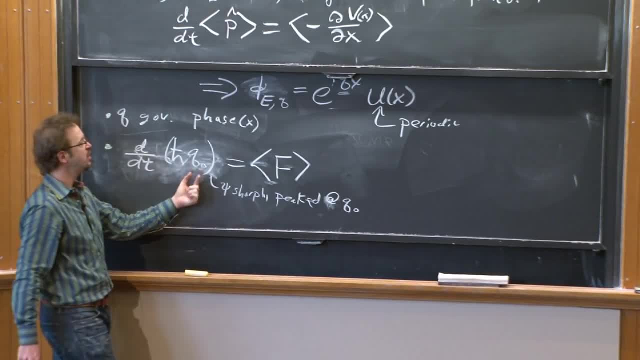 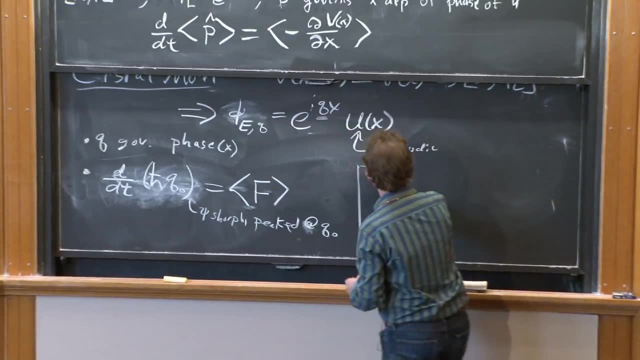 that's time, independent unless an external force is applied. just like this, Just like the momentum, And it's something that governs the phase of the wave function. just like the momentum. However, it's different in a crucial way: It is not the eigenvalue. 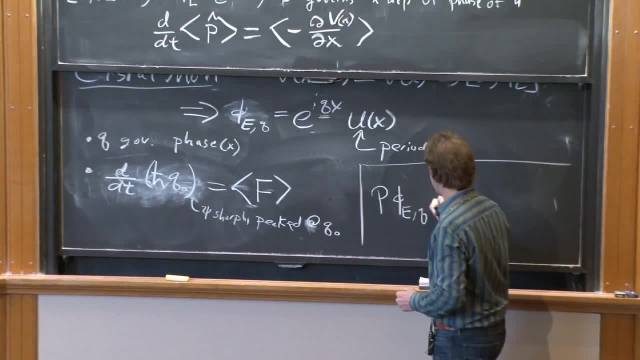 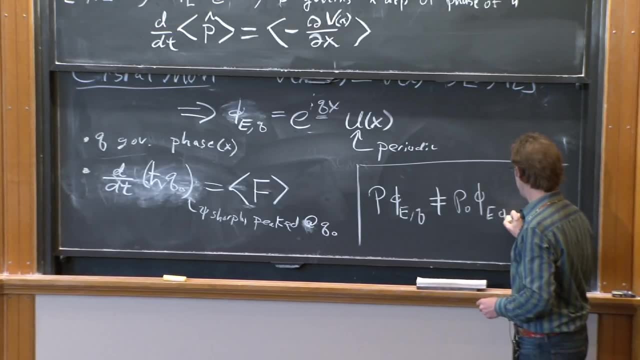 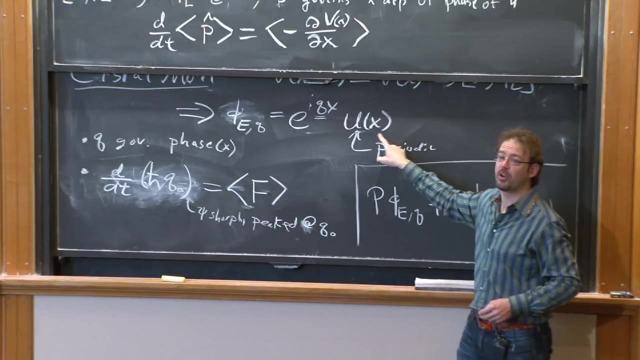 p on phi sub eq is not equal to a constant p0 times phi sub eq, Because when we act with p or we act with a derivative, we pick up a term from here which gives us a constant, But we also have this overall periodic piece. 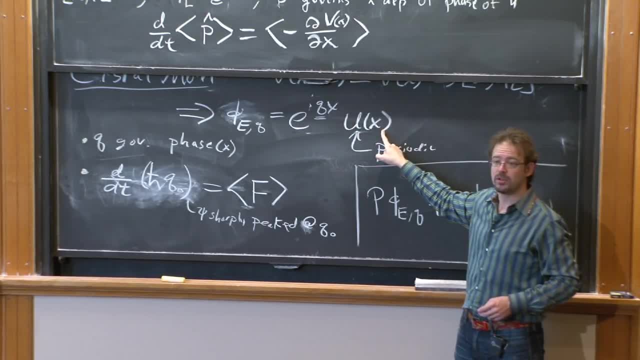 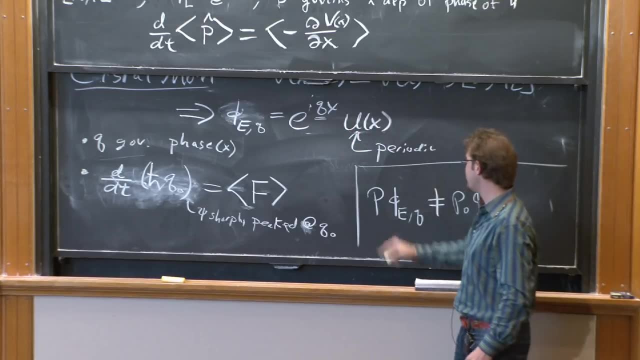 And its spatial variation. The spatial variation is generically non-zero, And if the potential is non-trivial, it's always non-constant. So when the momentum operator hits this guy, it will generically not give us 0. Then we'll get two terms and we will not. 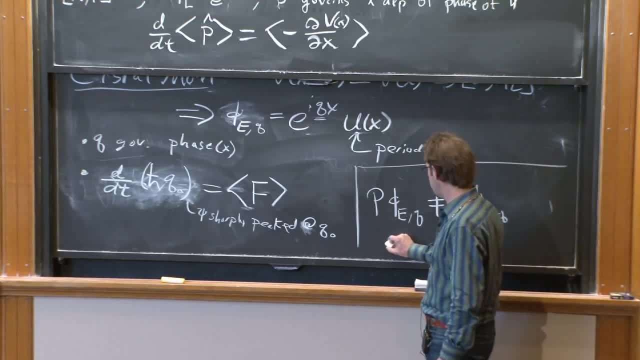 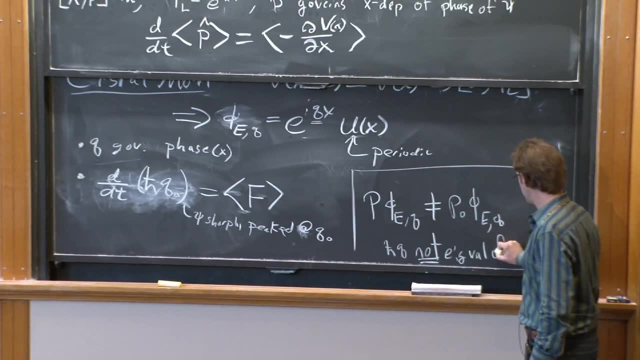 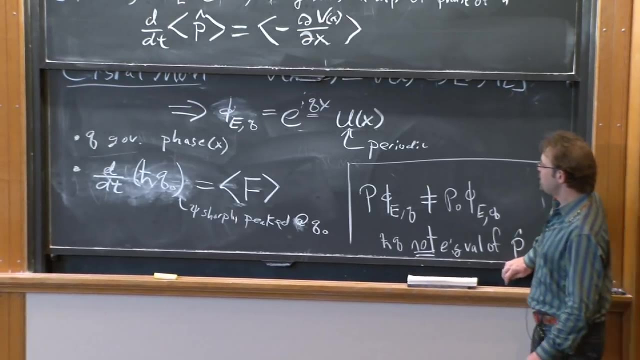 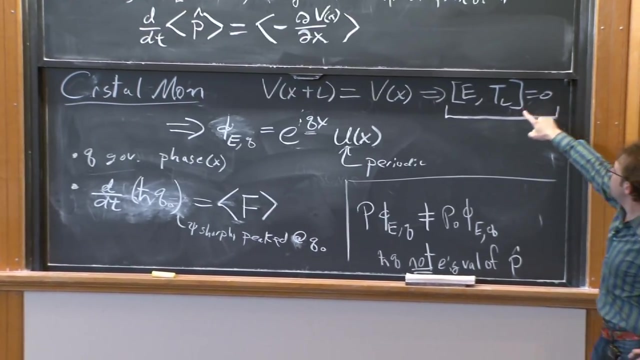 get an eigenvalue equation. So q is not the eigenvalue h bar q is not the eigenvalue of p. And what's the last important property of q that's different from the momentum? It comes from the commutator, which tells us that the thing that's conserved 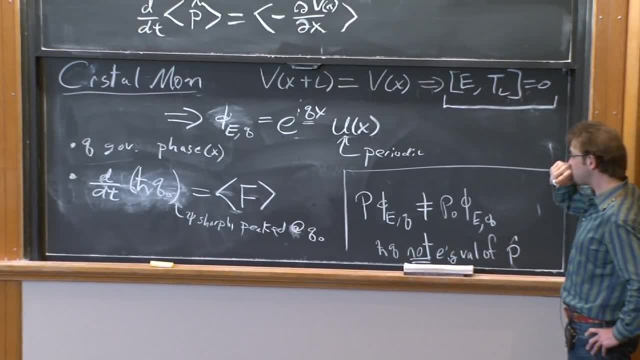 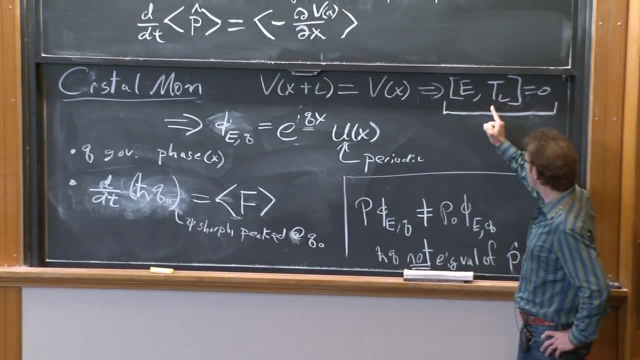 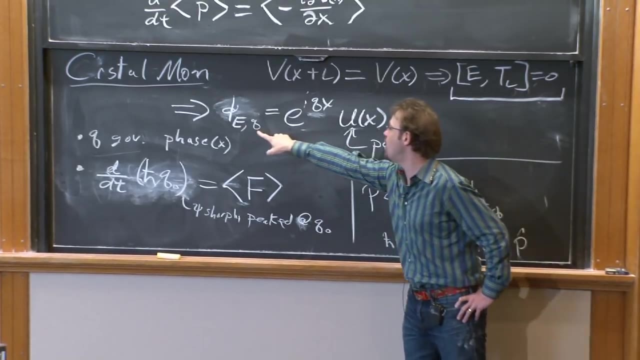 is the expectation value of tl is really the precise statement And, in particular, what this tells us is that the eigenvalue of our wave function, under translations by l, is a quantum function. So it's a quantum function. So it's a quantum function. 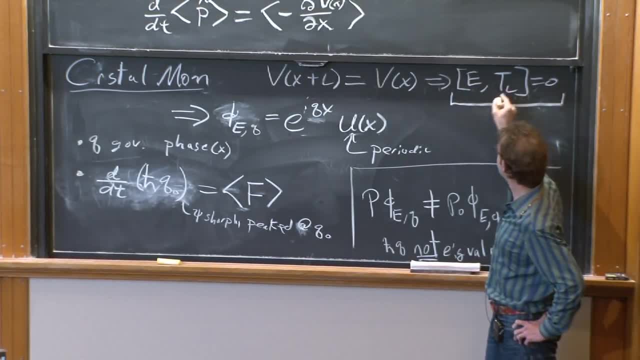 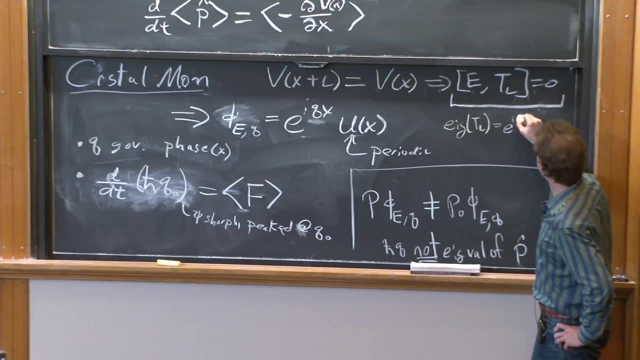 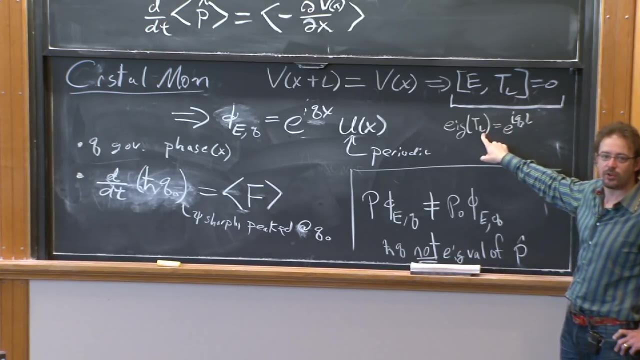 So it's a quantum function. It's a quantity that can be determined simultaneously with knowing the energy. However, the eigenvalue of t sub l on this state is equal to e to the iql, which means that q is only defined for determining the eigenvalue up. 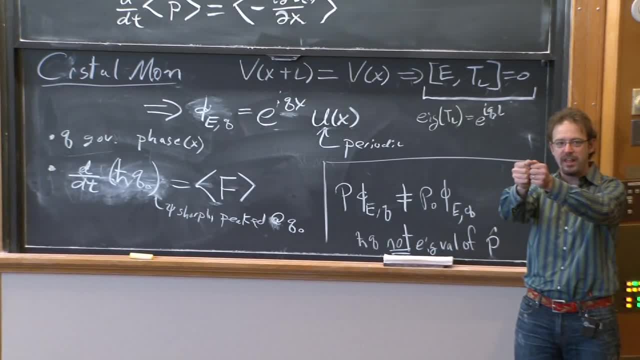 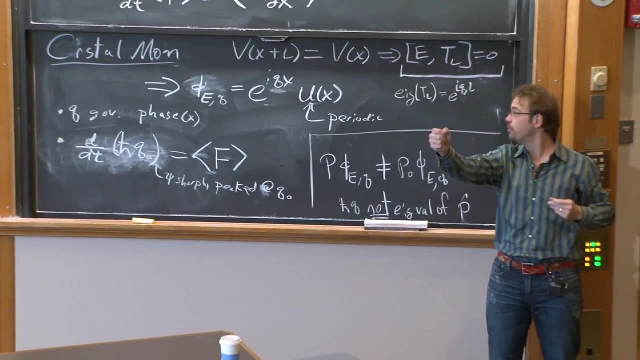 to 2 pi over l. If you have q, which is 0, and you increase it to pi over l, that value- pi over l- is effectively the same as the value minus pi over l, because it leads to the same. 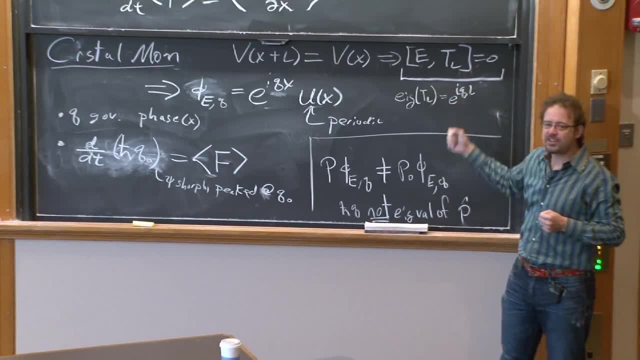 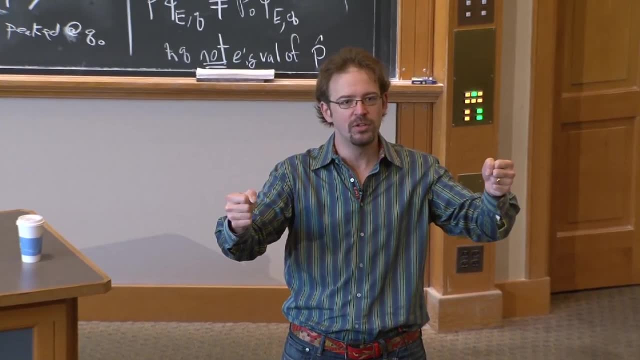 It leads to the same eigenvalue. But that's really strange because that means that q itself it's not strictly conserved, It's conserved mod 2, pi over l When you have momentum conservation. momentum is strictly conserved if there's no force. 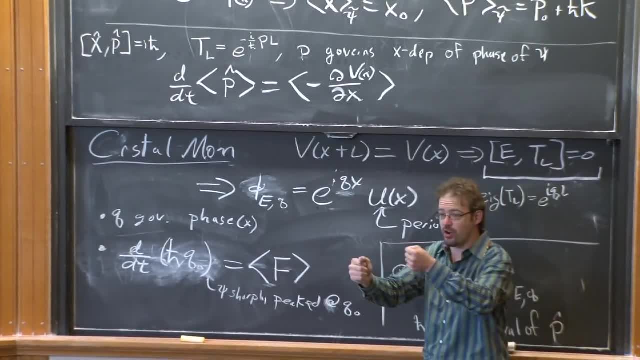 And even if there is a force, it's increasing control by the force. As you turn on a force, it just constantly increases. For the crystal momentum that's not the case. You turn on a force, it increases according to the conservation law. 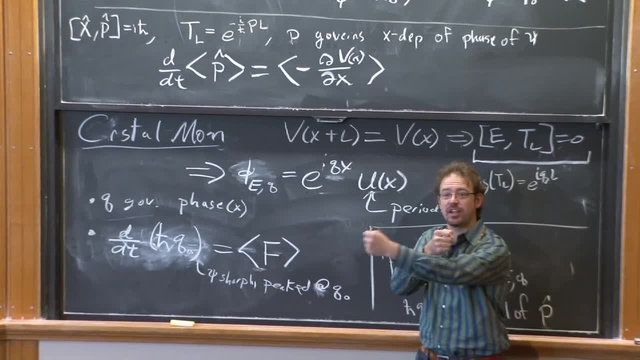 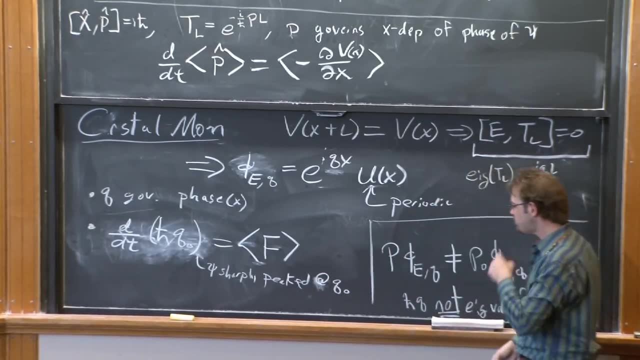 But It's not increasing constantly. It's periodic, It's periodically defined, So it increases and then it ends up at a smaller value. It increases and ends up at a smaller value, So it carries many of the same properties. It governs the phase. 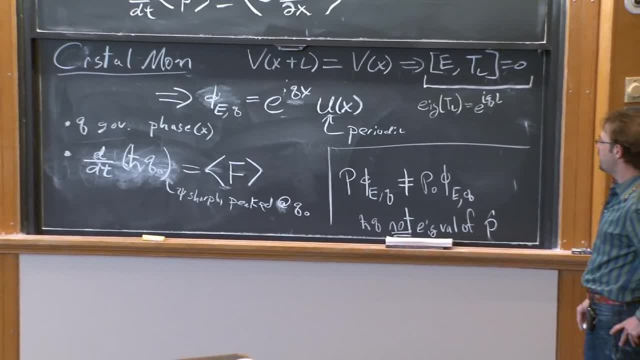 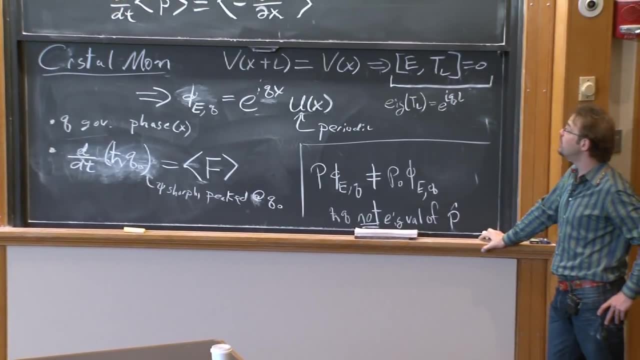 It's time independent unless there's an external force applied. It's the eigenvalue controls the eigenvalue of an operator that commutes with the energy when you have a periodic potential, in the same way that the momentum commutes with the energy when 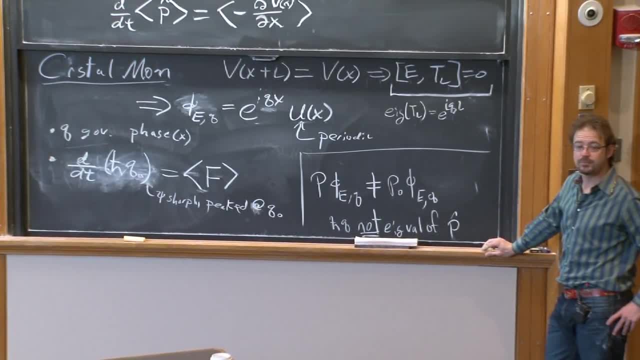 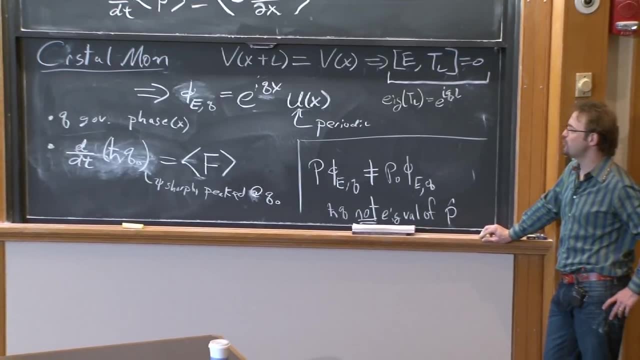 you have no external force. when you have a constant, It's the eigenvalue of the potential. Did that help? Good, OK. So developing an intuition for the crystal momentum, I think, is best done by just playing with examples, And you'll do that more in a course on solids. 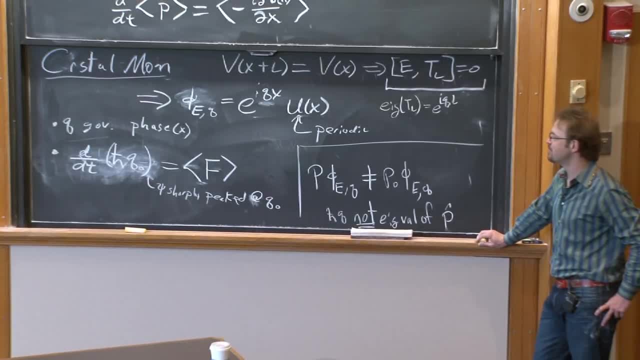 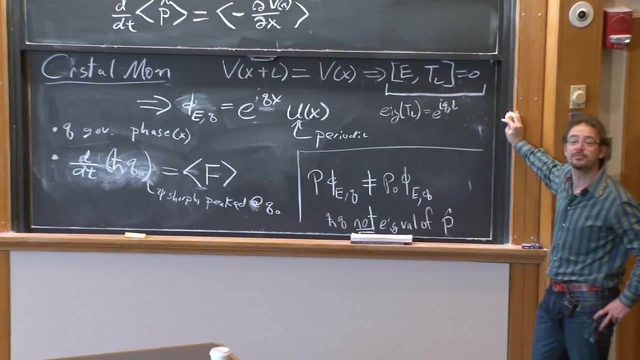 which I encourage you all to take, because it's really beautiful stuff. But for our purposes, this is going to be the full set of ideas we'll need for: Yeah, Can you get something in lightning off of the Ah Yeah. 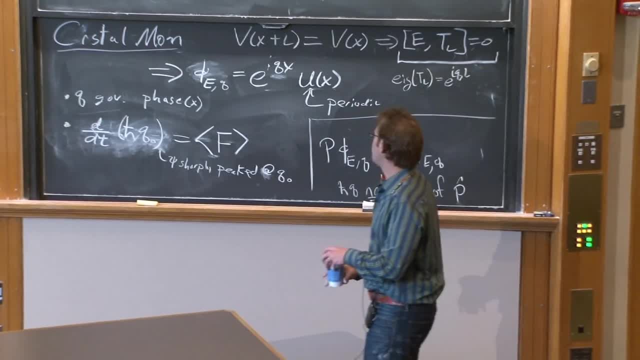 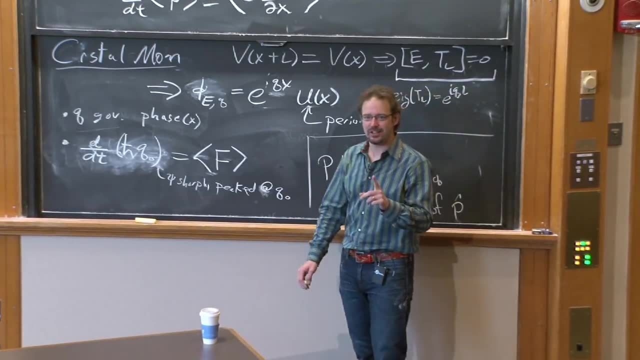 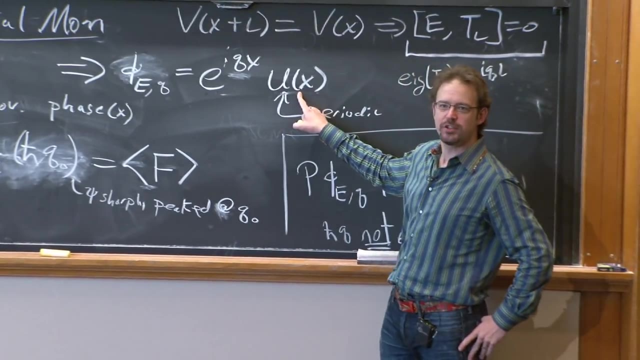 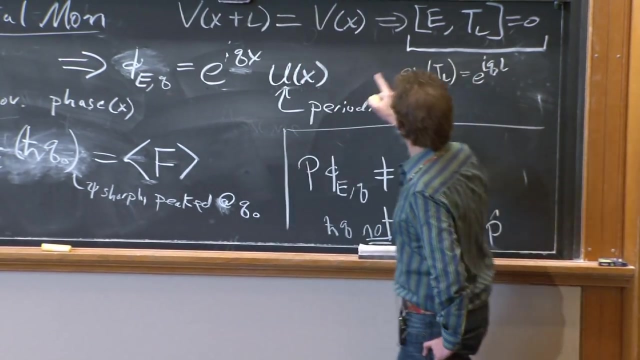 Yeah, Yeah, Yeah, Good, So, thank you. So this involves a slight subtlety which I've been glossing over in the entire story here, which is the following: So is u of x a real function? Well, when we started out asking what? 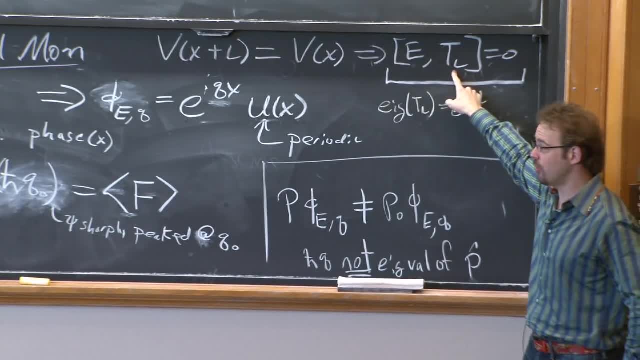 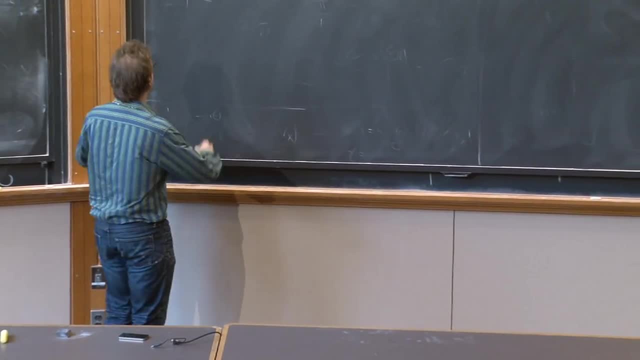 are the eigenfunctions of the translate by L operator. all we showed Was that, and I'm going to do this on a separate board, just to make it clear. Tell me if this turns off because it kept bumping. OK, cool. 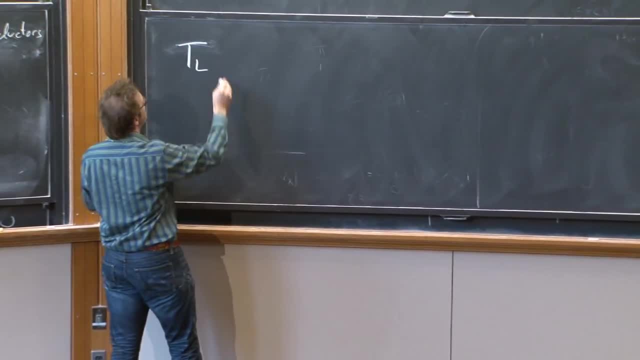 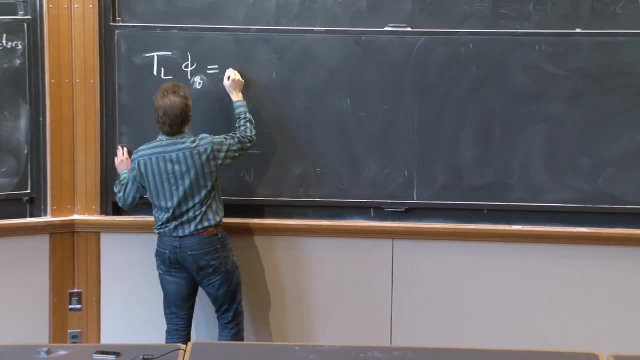 So when we started with translate by L and we constructed its eigenfunctions, we said that translate by L q, phi- I'll just say phi sub q is equal to some phase And this is unitary, so its eigenvalue must be an actual phase. e to the i alpha of phi sub q of x. 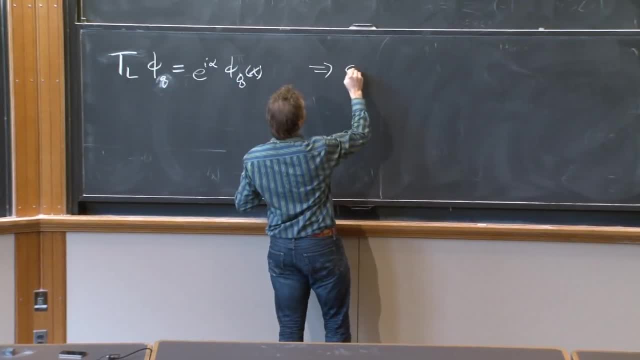 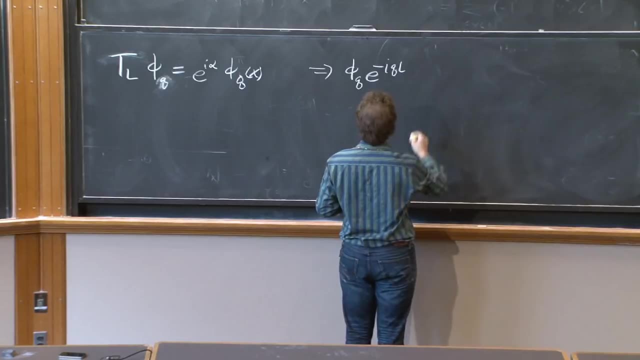 And let's just suppose that this is true. Then this tells us that phi sub q times e to the minus 1.5.. OK, e to the minus iql equals u. So I'm just going to use this to define a new function: u sub q. 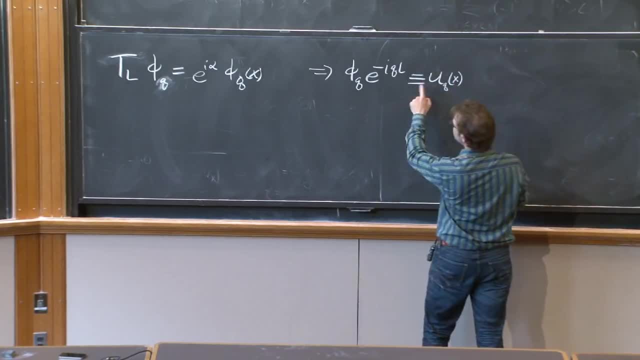 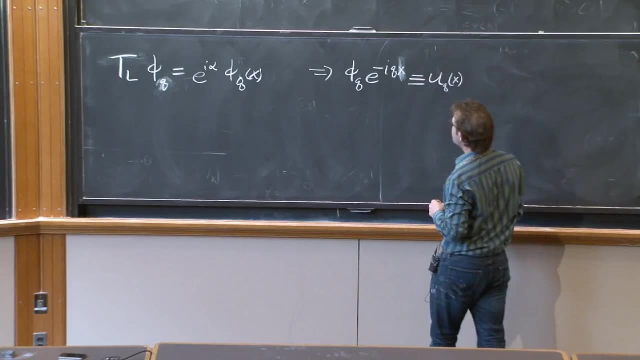 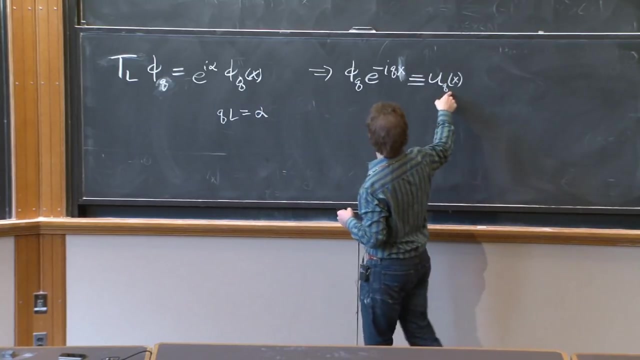 Or just u I'll u sub q, fine x. So this defines a new function: u sub q. I take an eigenfunction, I multiply it by some phase, Sorry, e to the minus iqx. If we choose ql to be equal to alpha, then acting on u sub q. 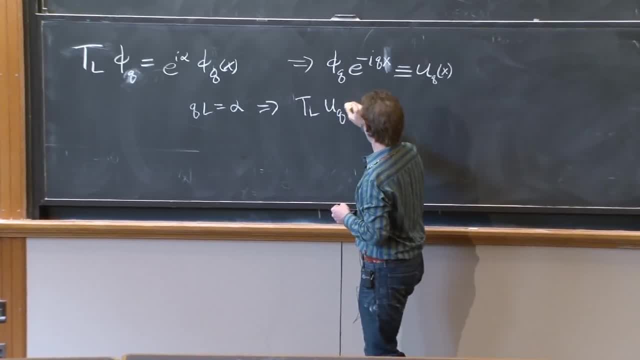 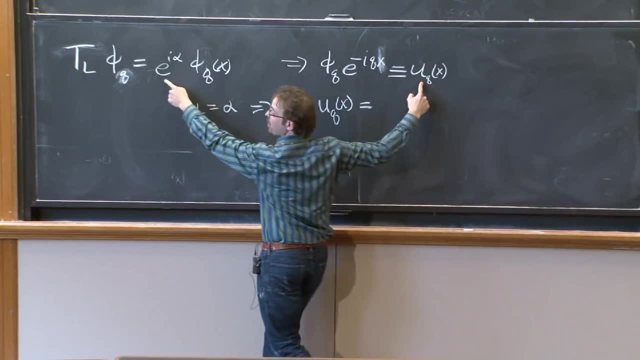 by translate by L on u sub q of x is equal to well, if we act on phi sub q with translate by L, what happens with phi sub q? We pick up a phase e to the i alpha. What happens to e to the minus iqx? 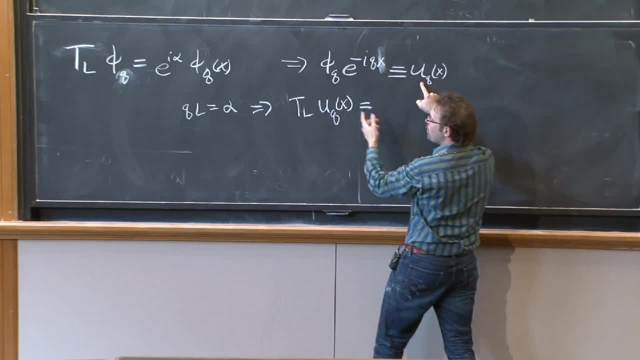 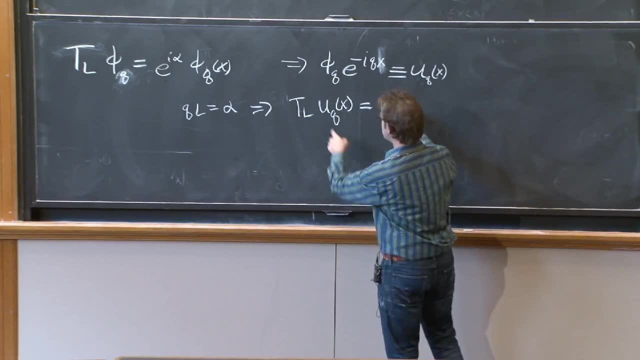 x goes to x plus l, We pick up a phase e to the minus iql. So if ql is equal to alpha, those two phases cancel and we just get u back. u sub q of x, But translate by L of u sub q by definition is equal to u sub q of x plus l. 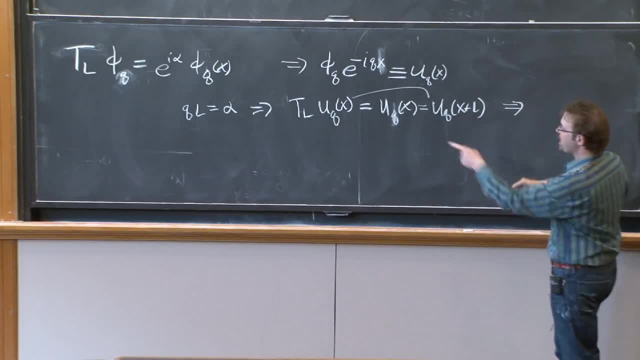 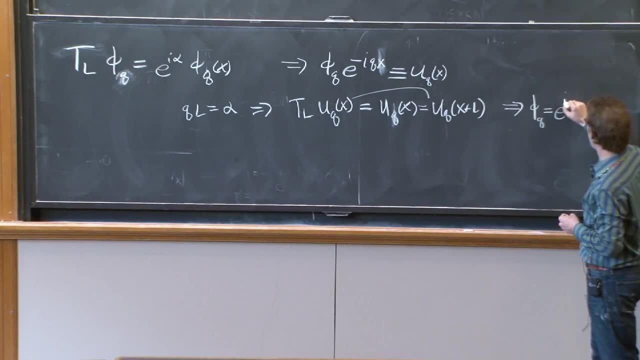 So what we've determined is that if we pick ql is equal to alpha, then phi sub q. phi can now be labeled by its eigenvalue. q can be written in the form e to the iqx: u sub q of x, where this is periodic. 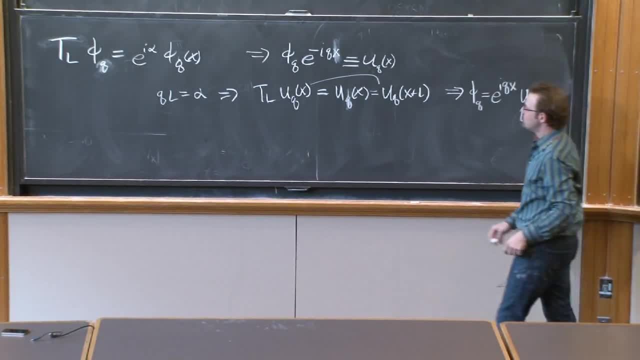 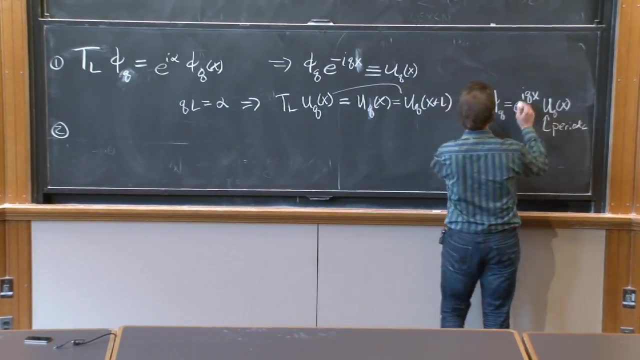 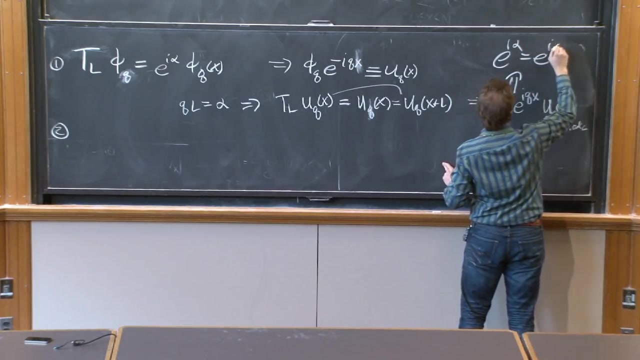 Everybody agree with that. OK, so that's step one. Step two is to say: well, look E to the i p? U, Since the eigenvalue of this guy under t sub l e to the i q alpha is equal to e to the i q l. 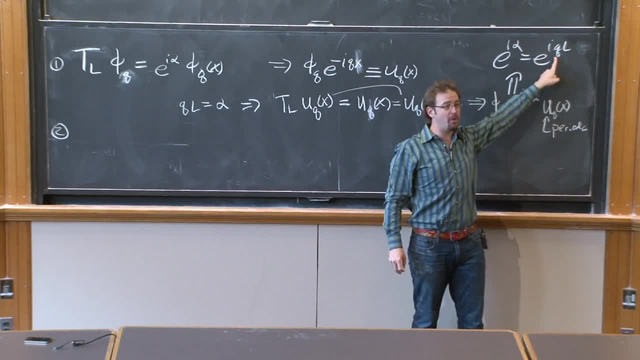 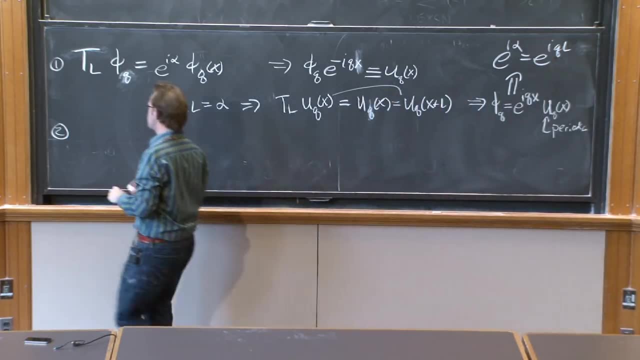 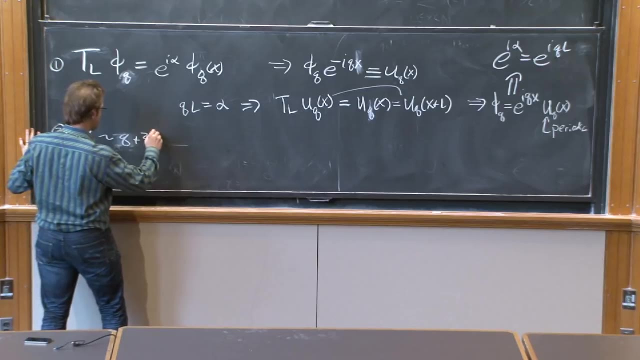 Since this is periodic, under shifts of q by 2 pi upon l, I can just choose to define q up to 2 pi over l. So q I will take to be equivalent to q plus 2 pi over l, And the reason I'm going to do that. 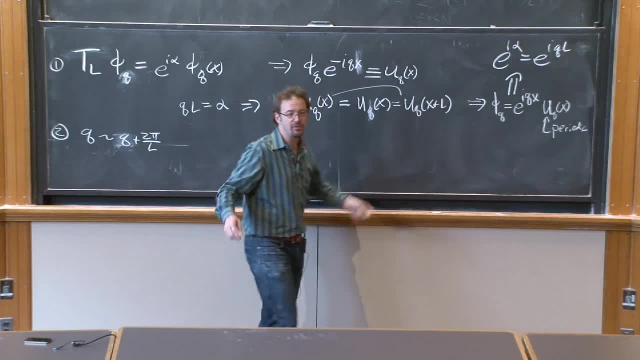 is because it gives the same eigenvalue, And if I want to label things by eigenvalues, it's redundant to give multiple values to the same eigenvalue. Now, there's a subtlety here, though, And the subtlety here is this: 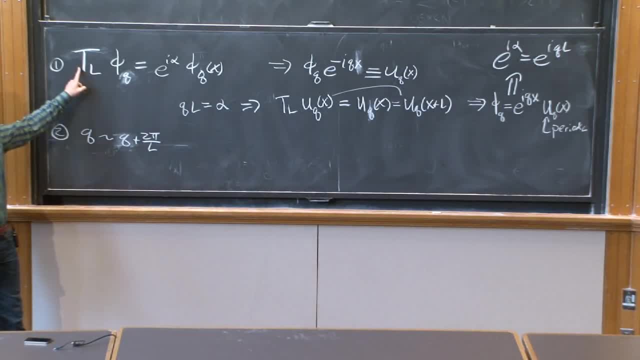 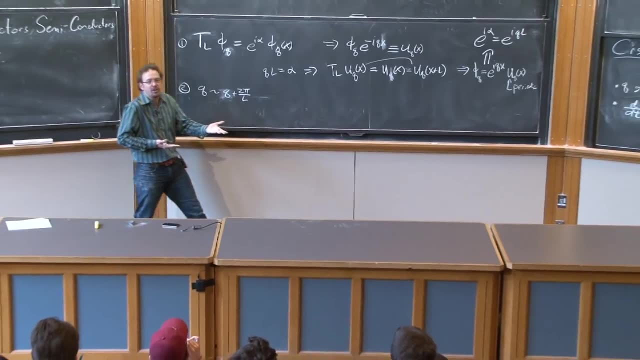 Suppose we have a free particle. Does a free particle respect translation by l? So if we have a free particle, the potential is 0. That constant function is also periodic under shifts by l, Because it's just 0. So it's stupidly periodic. 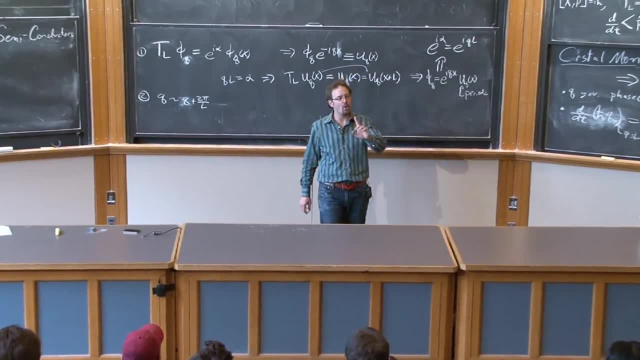 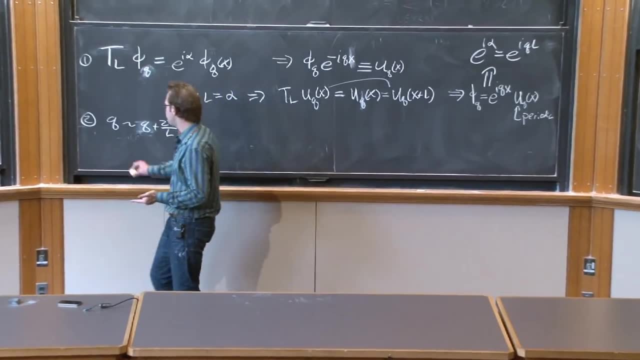 But it's periodic nonetheless. So now I'm going to ask the following question: What are the common eigenfunctions of the energy and translate by l for the free particle? We did this last time. So the common eigenfunctions of translate by l and the energy. 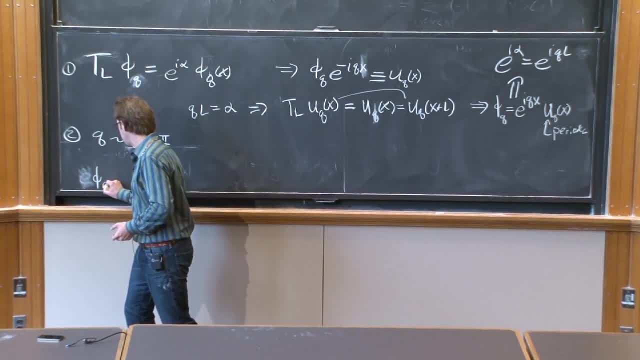 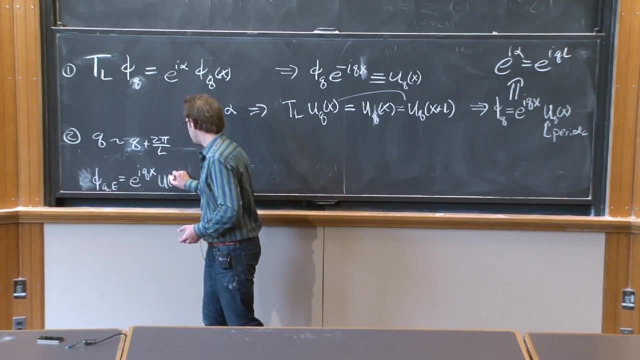 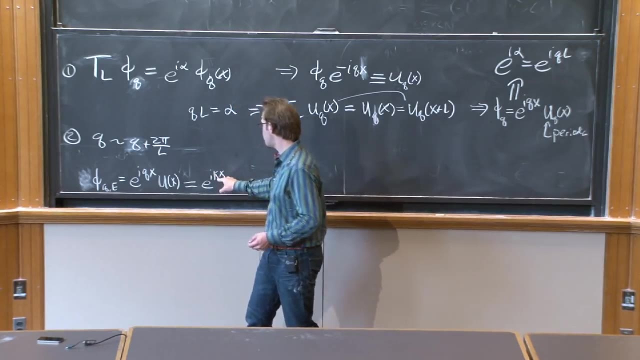 are the wave functions. phi sub q comma e are equal to e to the i, q, x times. some function u of x on general grounds. But we know what these eigenfunctions are. They're just e to the i k, x, where k squared upon 2m. 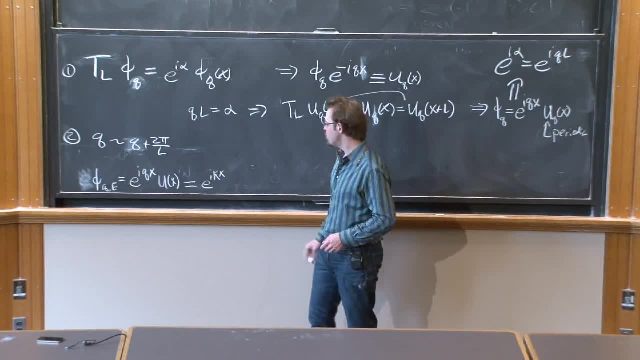 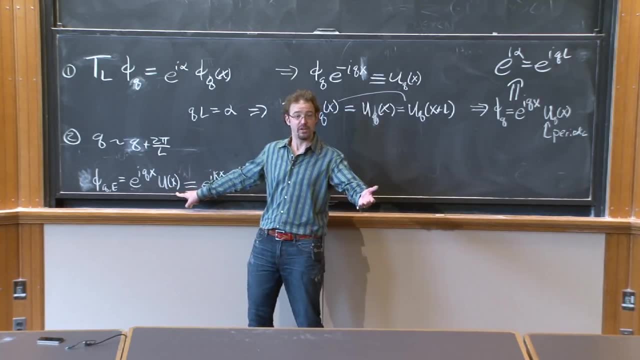 is equal to e. h bar squared k squared upon 2m is equal to e. So we know that these are the correct eigenfunctions, But we're writing them in the form e to the i, q, x, u. Now you say that's fine. 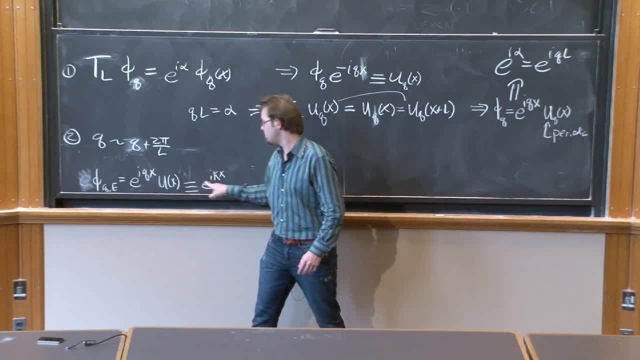 There's nothing wrong with this. We just say u is constant and q is equal to k, Then these functions are of this form, But they're of this form, with e to the i, q, x being e to the i, k, x and u of x being constant. 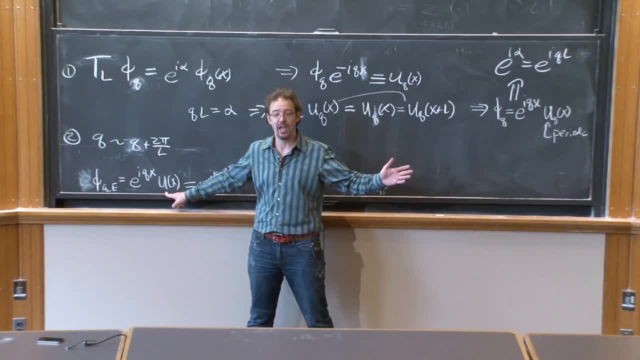 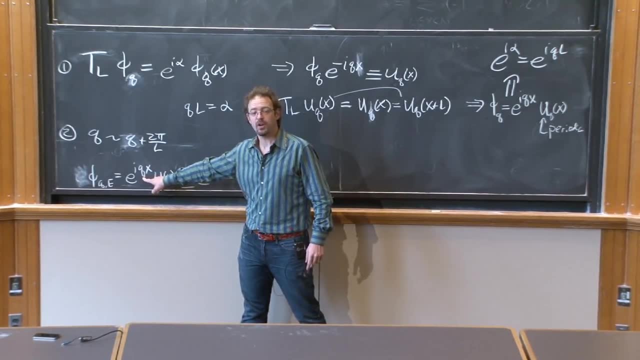 There's nothing wrong with that. Does everyone agree? Perfectly consistent? However, I thought we said that q is periodic by 2 pi. If q is periodic by 2 pi, then that would seem to imply that k is periodic by 2 pi. 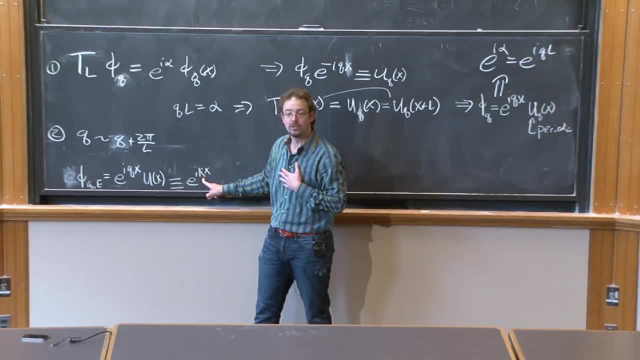 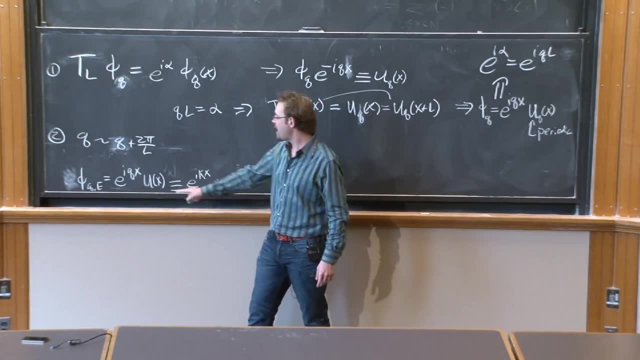 But we know that's not true because any k is allowed for a free particle. So if we want to think about q as periodic by 2 pi upon l, then we cannot require that u is real, because it must be the phase that makes this up. 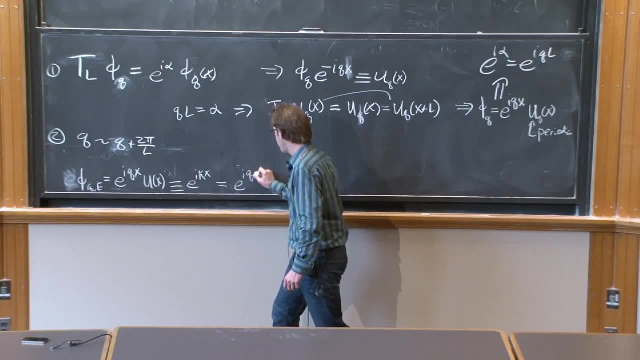 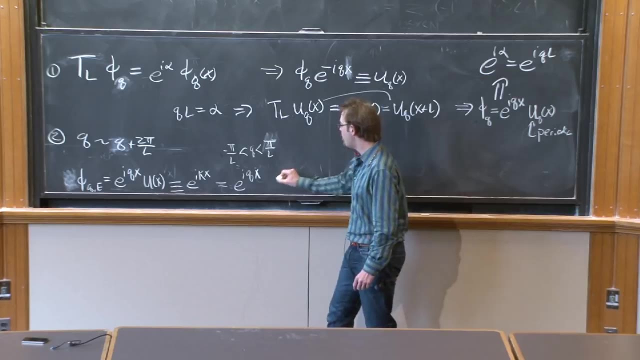 It must be, So I can always write this as e to the i, q, x, where q is less than 2 pi upon l, Or, sorry, q is between 2 pi or pi upon l and minus pi upon l, So that it's defined only after this periodic thing. 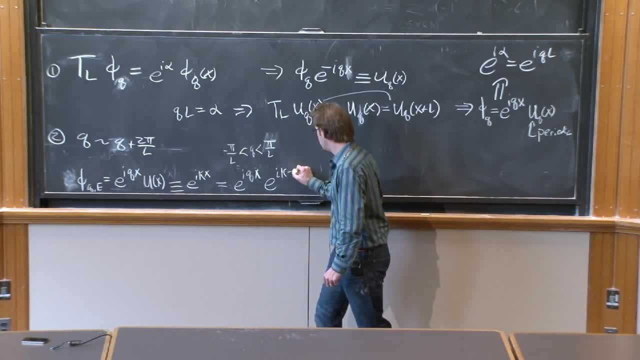 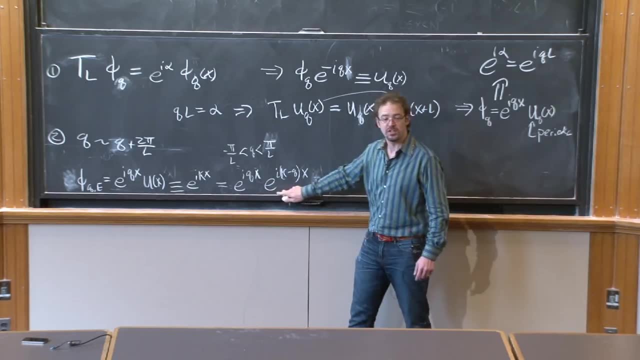 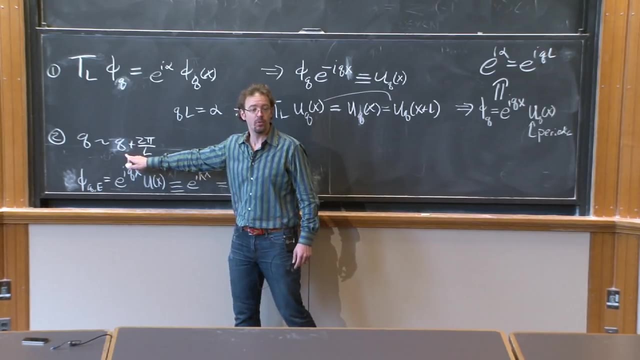 But times some additional phase e to the i k minus q x. So this is trivially equal to e to the i k x. But now u is not a real function. On the other hand, if we hadn't imposed the requirement that q is periodic, we wouldn't have needed to make u real. 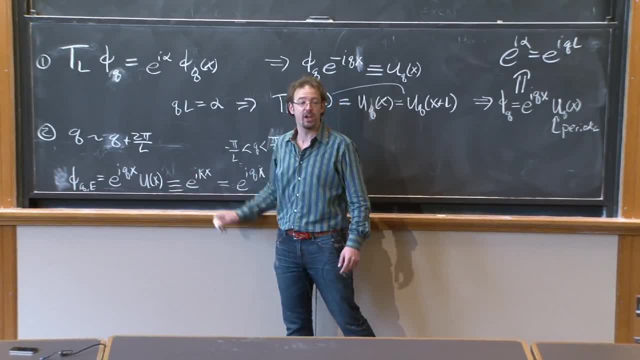 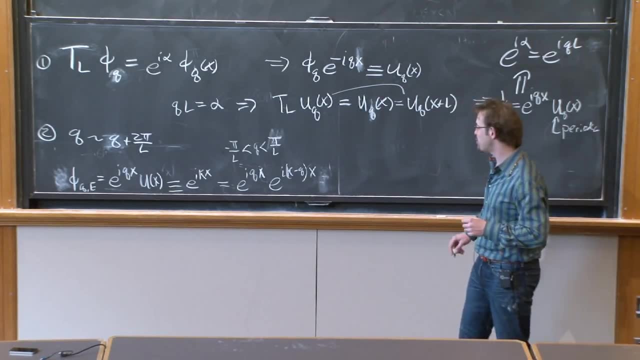 We could have just taken q to be equal to k for any value, k, And then u would be constant, U would be real. So this is important for answering the excellent question that our fearless recitation instructor provoked me to answer, which is that we'll. 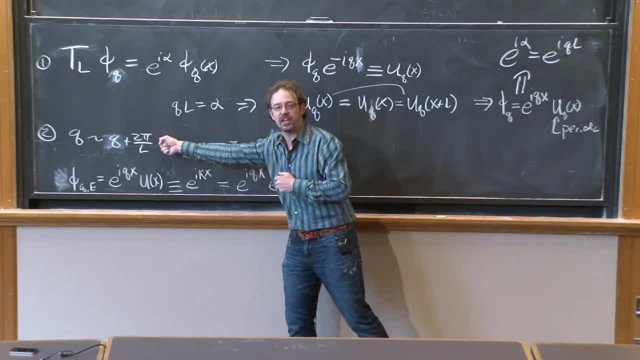 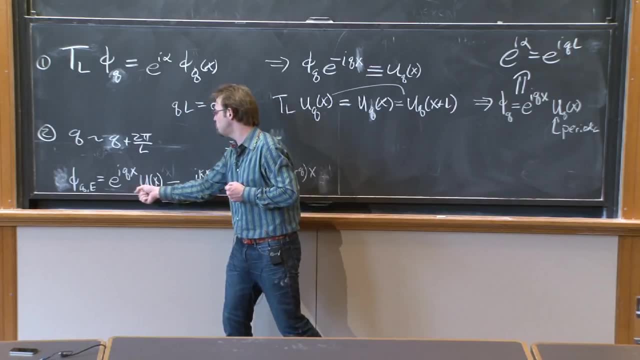 come back to the question in just a second, But I want to emphasize this: That if we're going to take q to be defined only up to shifts by 2 pi over l, it's important that we allow u to be not real. 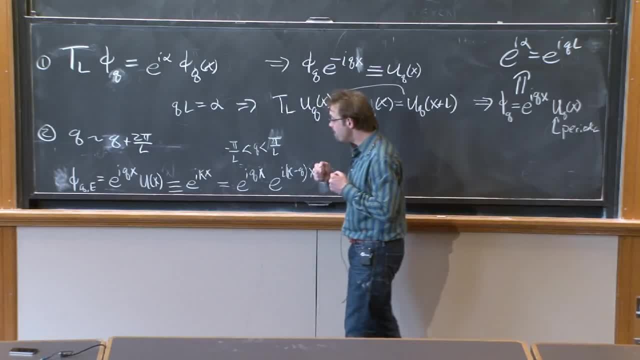 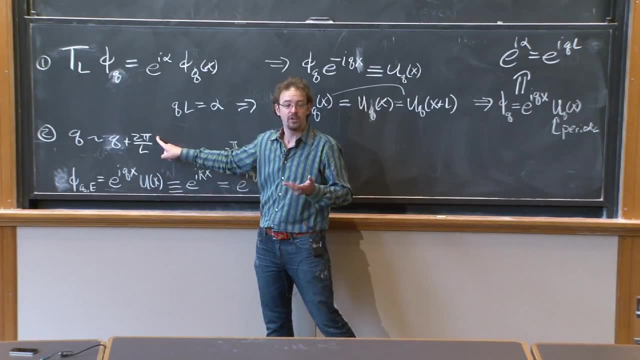 It must be able to be an overall phase. But if we want u to be always real, we can do that. We just can't impose this periodicity. Different values of q mean different wave functions, And this is really what's going on when you see those plots. 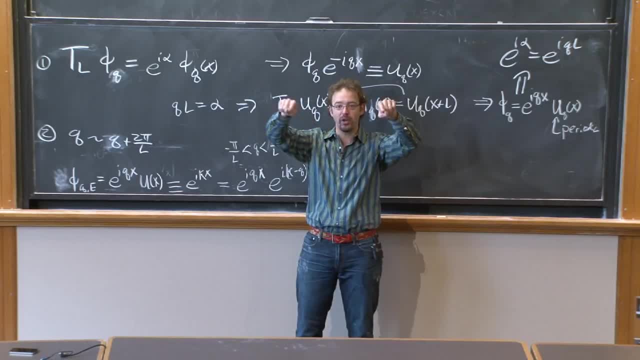 Sometimes you see the plots as parabolas. The bands are represented by parabolas with wiggles, And sometimes they're folded up, And that's the difference. The difference is that when you fold them up, you're imposing this periodicity. 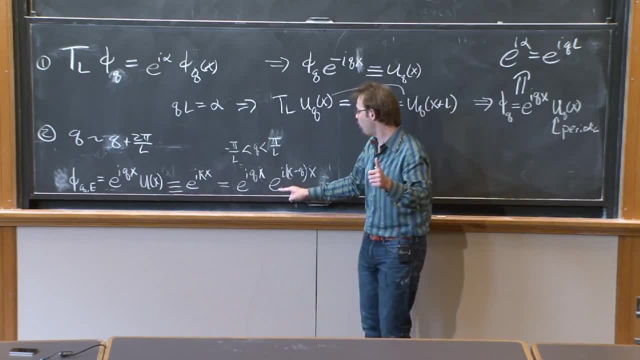 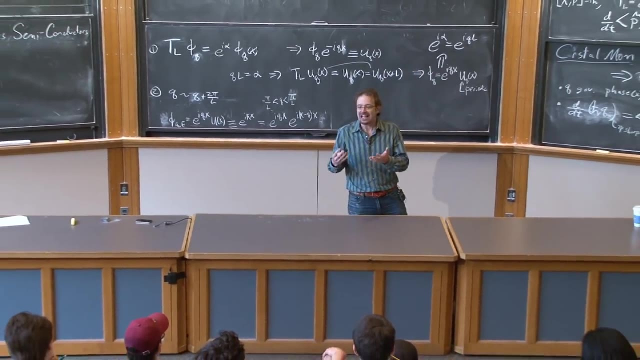 And you're labeling the eigenfunctions by q and the overall amount of the number of k, effectively of k phases that you're subtracting off. Yeah, So is this an arbitrary choice? Yeah, I mean, how to say It's exactly akin to a choice of variables. 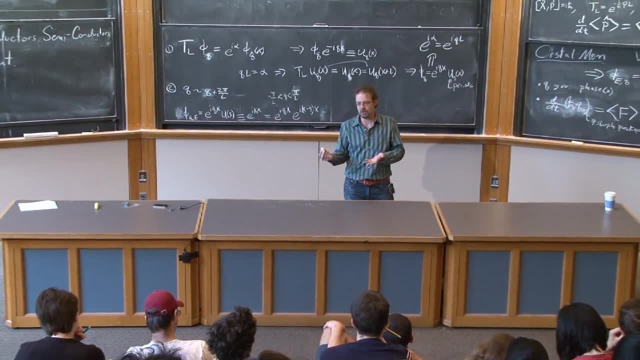 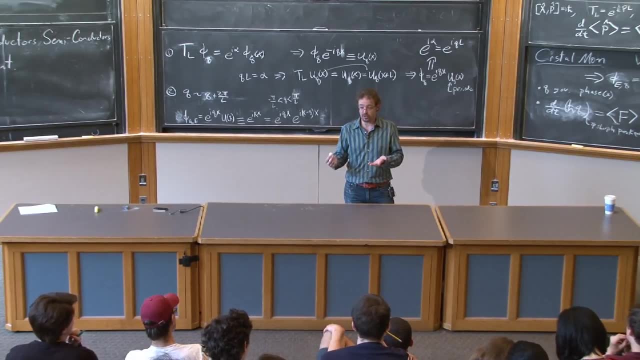 In describing the position of this particle. should we use Cartesian coordinates or should we use spherical coordinates? Well, it can't possibly matter, And so you'd better make sure, in any description of your system, that changing your coordinates doesn't change your results. 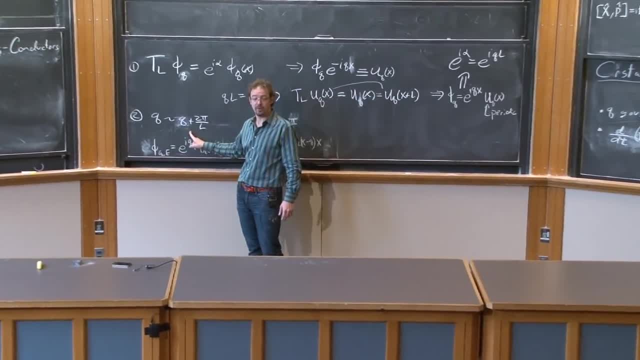 And here that's exactly what's going on. Do we want to define our variable to be periodic by 2 pi upon l? Well, OK then, But u can't be real. Or we could take q to be not periodic by 2 pi l. 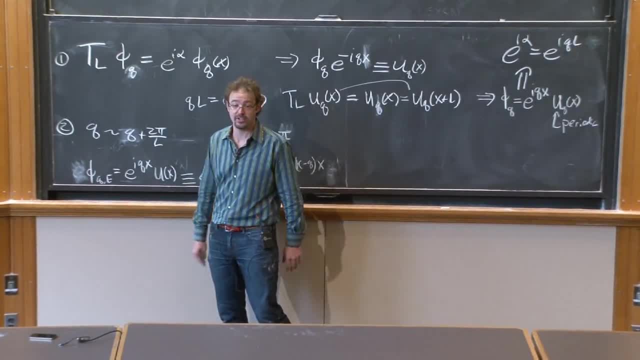 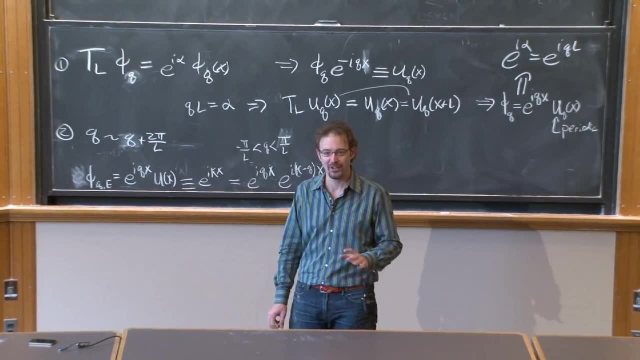 and impose that u is real. It's just a choice of variables, But it can't possibly give different answers. The point is, this is a subtle little distinction that we gloss over and is glossed over, into my knowledge, Every book on intro quantum mechanics. 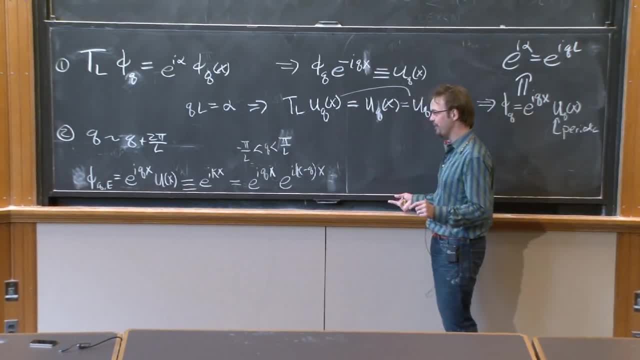 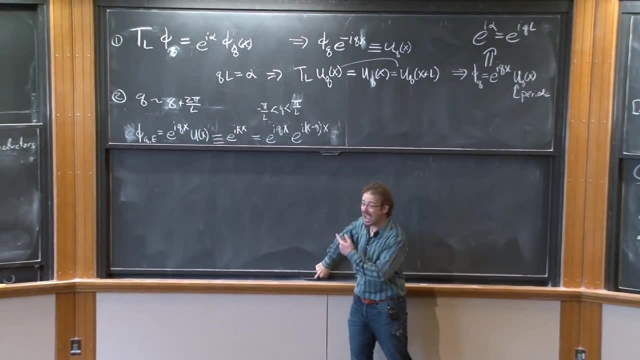 that even covers periodic potentials. it can be very confusing. Anyway, the reason that I had to go through all this is that, in order to answer the very, very good question that Professor Evans posed, I'm going to need to deal with this fact. 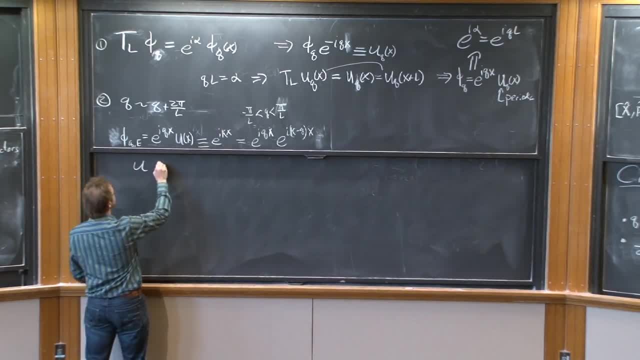 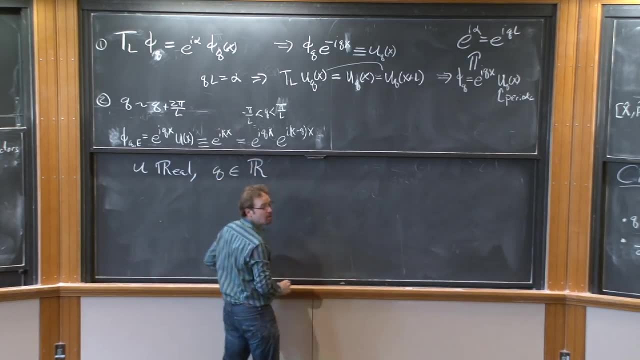 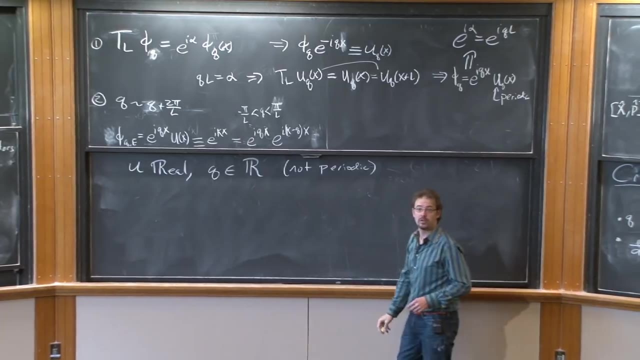 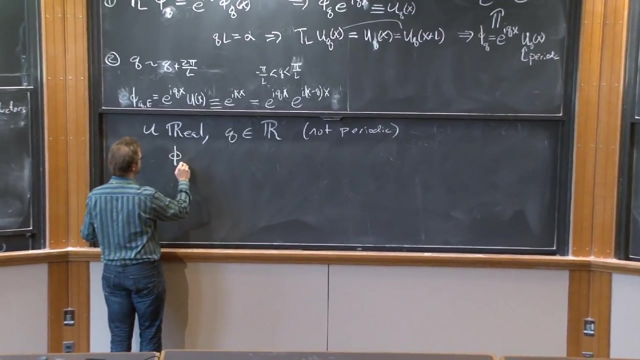 So for the moment, let's work with u- real, and q an unconstrained real number, so not periodic. Are we cool with that for the moment? OK, So if we do that, then notice the following nice property of our wave function: 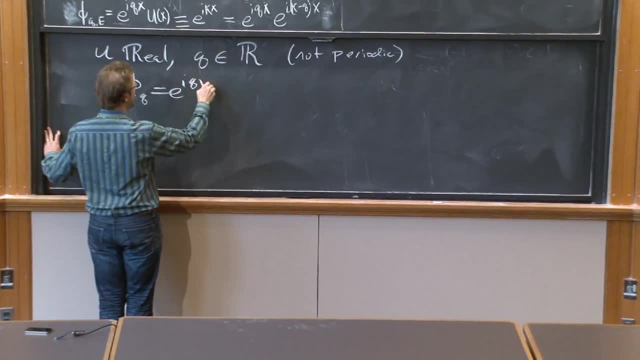 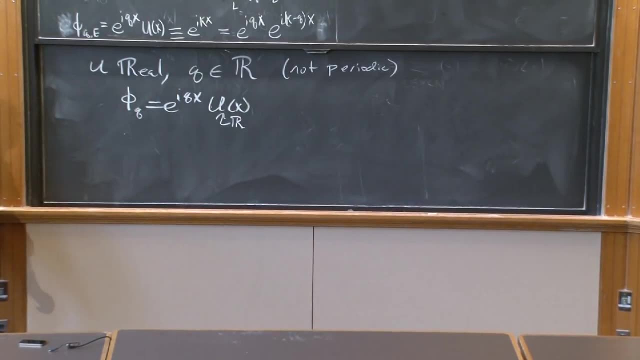 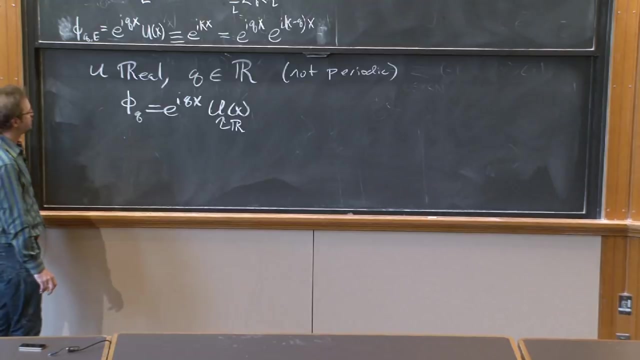 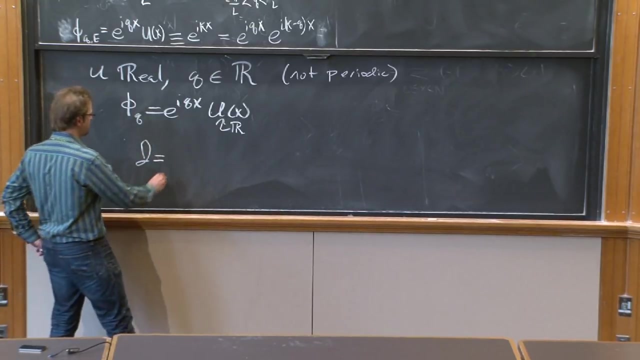 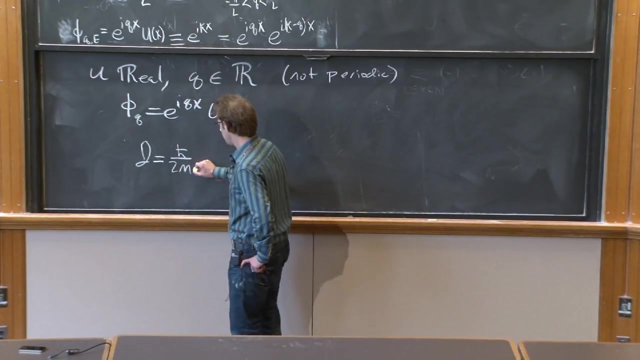 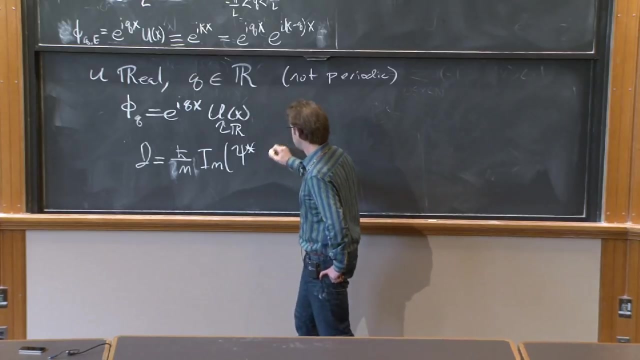 Our wave function, phi sub q is equal to e, to the iqx times u of q or u of x, which is real. So when we construct the current, remember that j boils down to the imaginary part h bar over 2m times the imaginary part of psi complex conjugate. 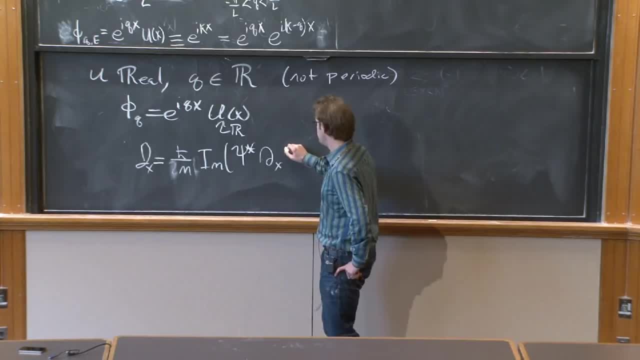 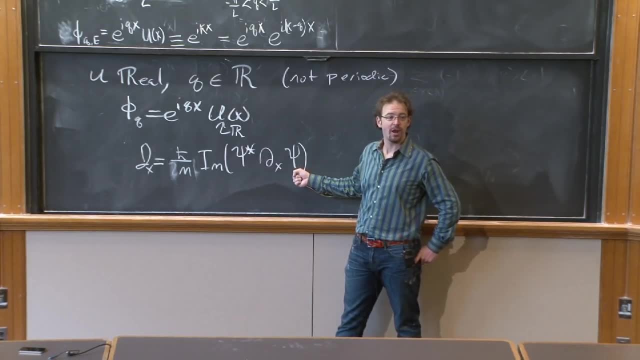 derivative with respect to x, which is the current in the x direction of psi, And we need this to be imaginary or we will get no current. You show this in a problem set If you have a pure, real wave function, for example. 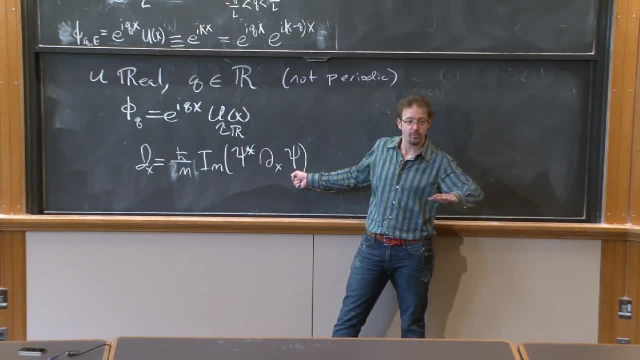 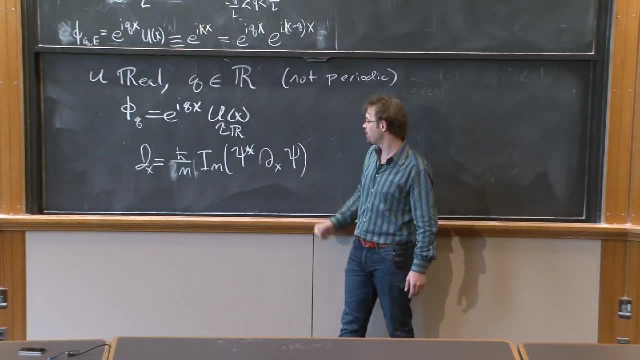 a single real exponential that's decaying, as on the wrong side of a barrier, then you get no current Nothing flows, And that makes sense. It's exponentially decaying. Nothing gets crossed, So we need the wave function to be real. 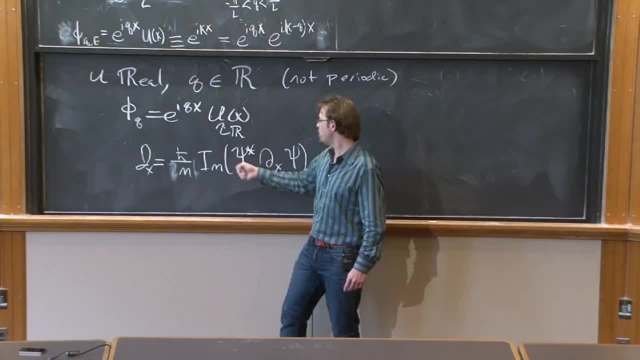 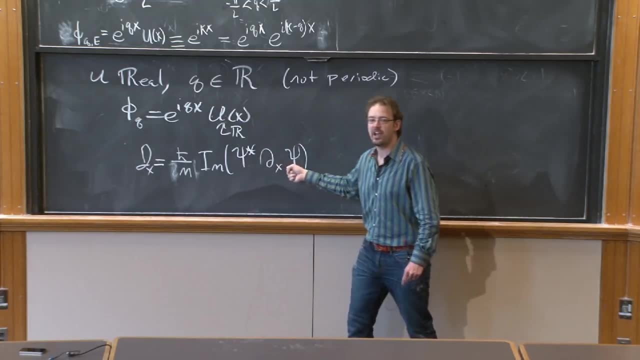 So if q were 0, we would get 0. And what you can immediately do from this compute, from this, is that if the derivative doesn't hit e to the iqx, if it hits u, then the phase e to the iqx cancels. 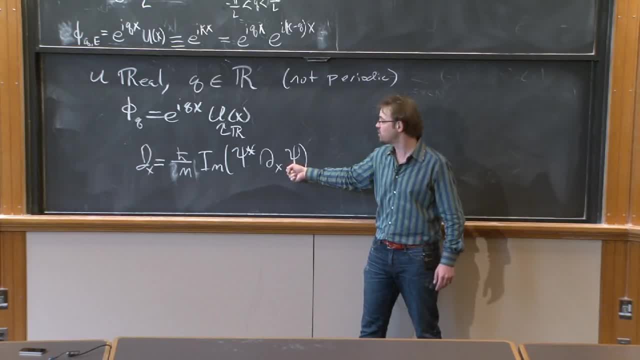 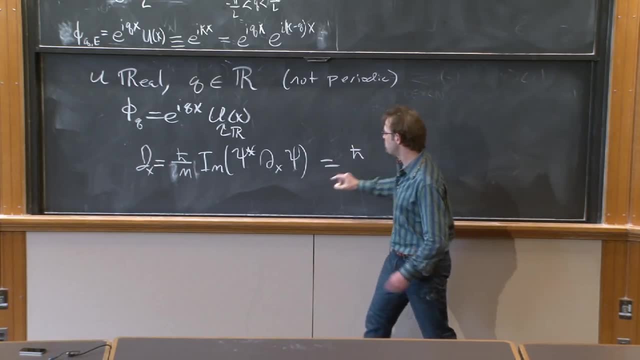 And so the contribution from that term vanishes. So the only term that's going to contribute in here is when the derivative hits the e to the iqx. But then this is going to be equal to h bar q, And we want the imaginary part, so that's going to eat the i. 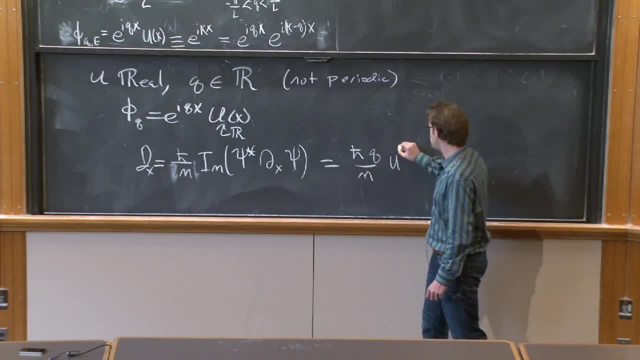 over m, And then we're left with u squared of x. So this is the current, But we had to take advantage. in order for this to be clean, we had to take advantage of u. We had to take advantage of u being real. 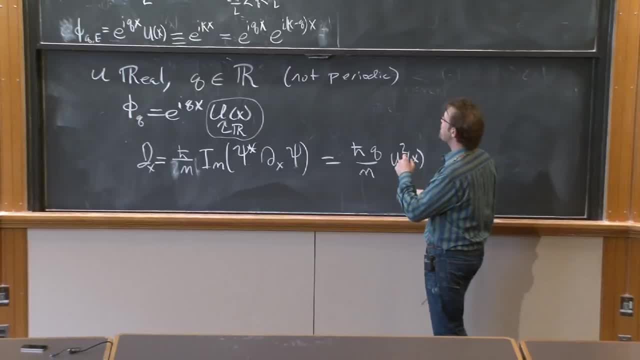 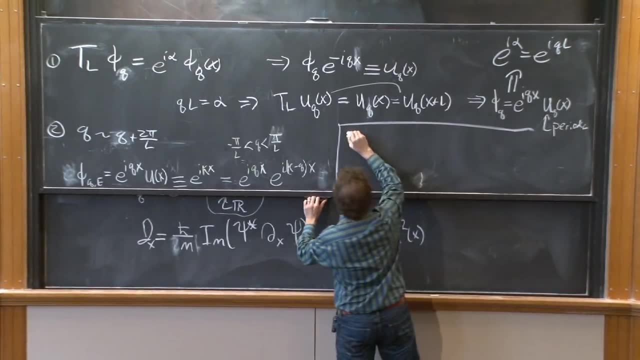 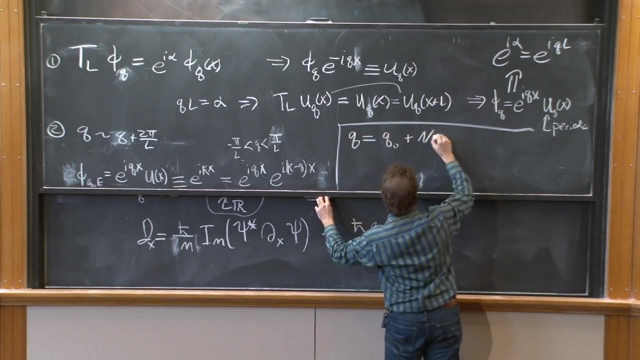 Everyone cool with that? Now there's one last twist on this, which is that if I have q- this is a side note going back up here to this logic- if I have q and I can always write it as some q0 plus n, pi over L. 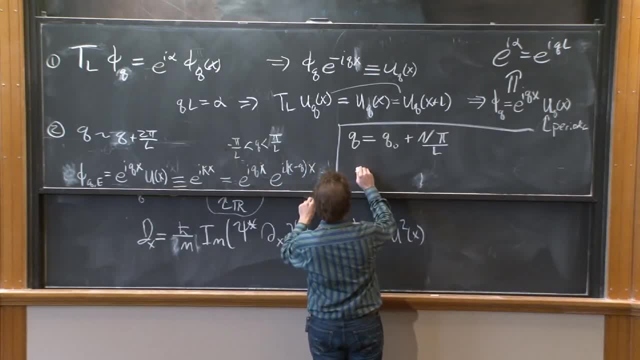 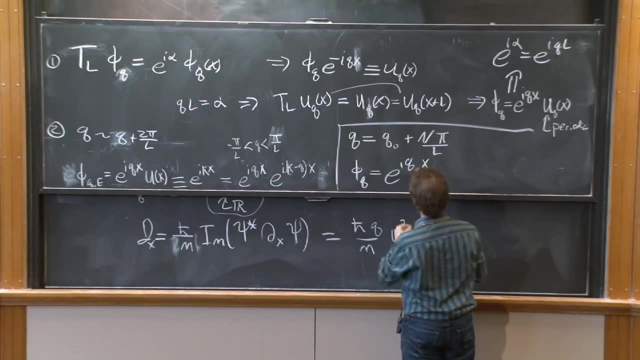 And so now what I want to do is I want to take sort of a hybrid of these two pictures And I want to say: phi sub q is going to be equal to e, to the i, q0, x, where this is the value that's. 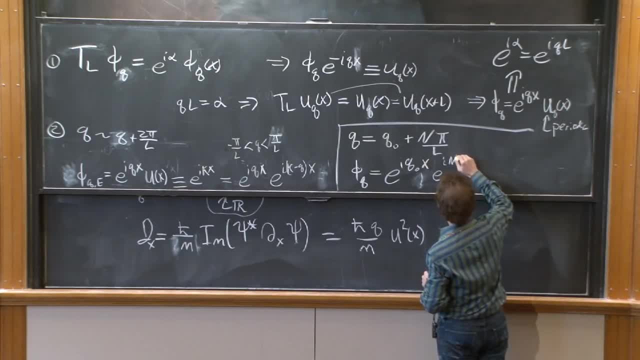 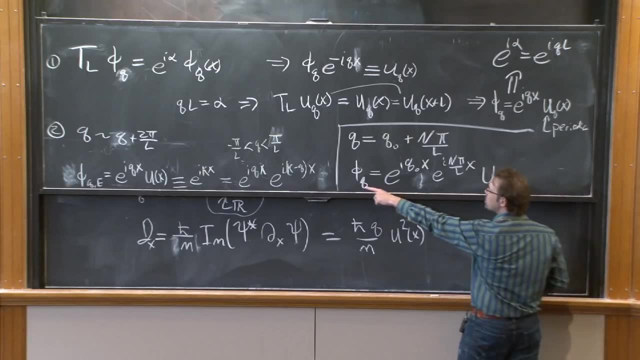 periodic by q, pi, e to the i n, pi, over L x, u. And so now, really, what I'm doing here is I'm labeling my wave function not by a single number, q, but by q0 and an integer n, comma n. 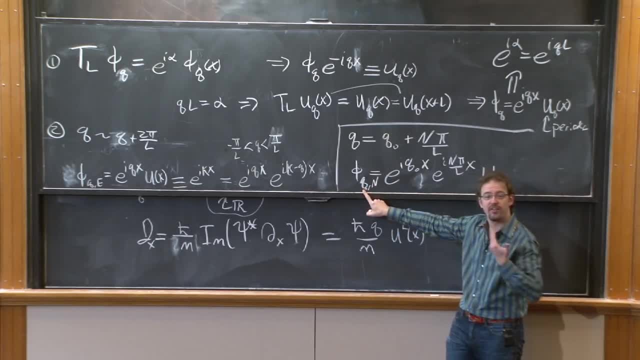 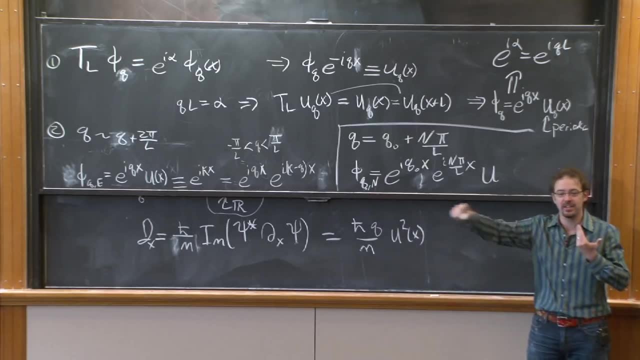 So q0 and n, And so now q0.. It's periodic, It's defined up to shifts by 2 pi. n is an additional integer And what it's telling you is: how many times did you have to shift back to get into that fundamental zone? 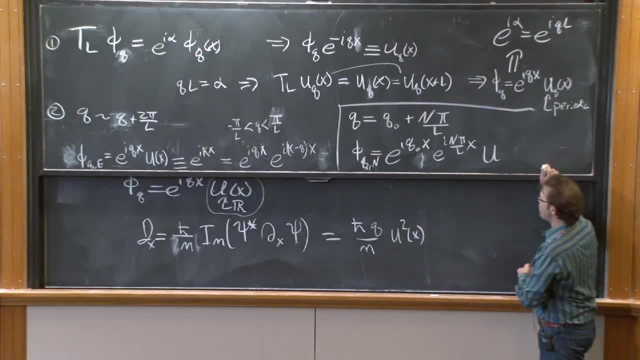 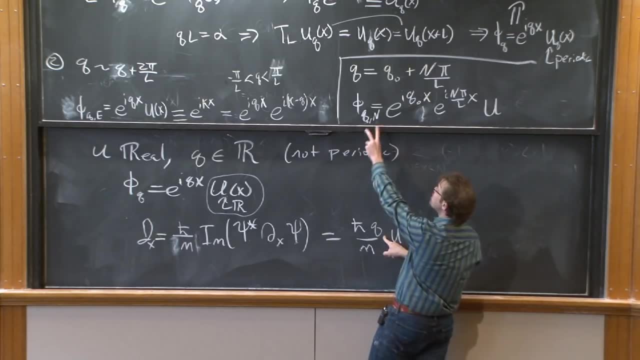 between pi and minus pi. And this fits nicely into this story, because now all we're going to get here is q, which is q0 plus n pi. So the current depends on both the part defined mod 2 pi over L, and the integer which tells you how many factors of 2. 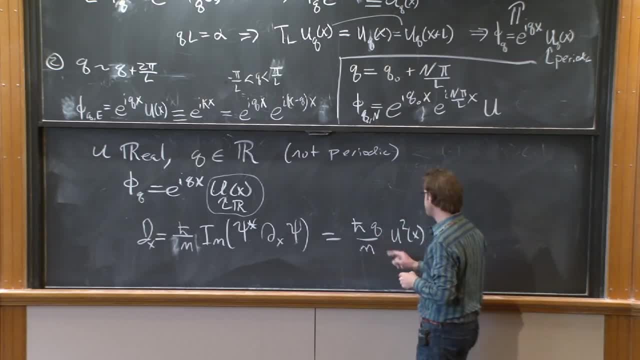 pi over L? did you have to subtract off to get into that fundamental zone? It's a little domain, But let's think back to our band structure. So what is this n quantity? Let's think back to our band structure. In our band structure we had something that looks like this: 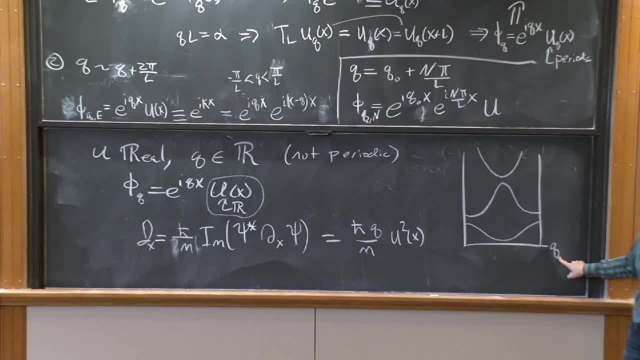 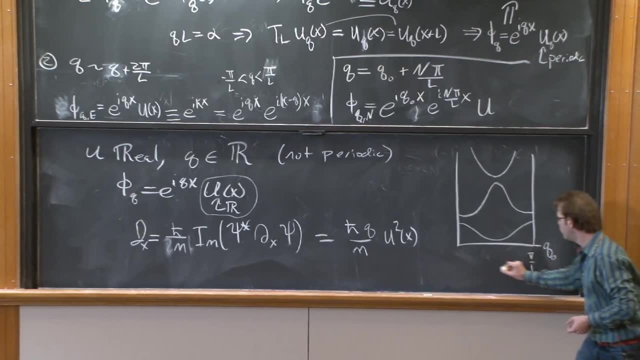 And here's a value of q. But am I plotting q? No, I'm plotting here q0.. I'm plotting the part that's periodically defined up to 2 pi over L. So this is pi over L. This is minus 2 pi. 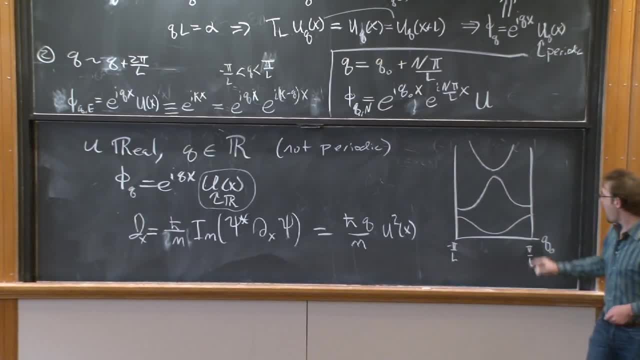 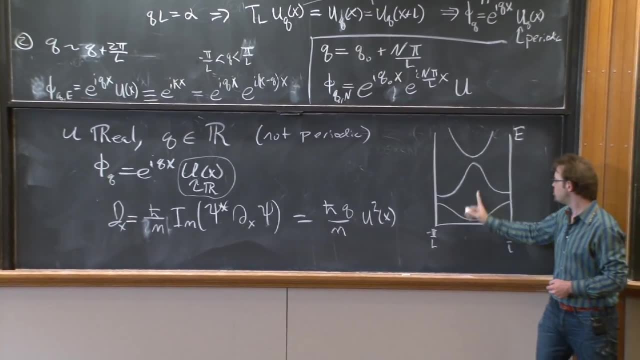 over L Or minus pi over L. OK, And what we see is that there isn't a single energy, because this is the energy in the vertical direction for these band pictures. There isn't a single energy for a given value of q. 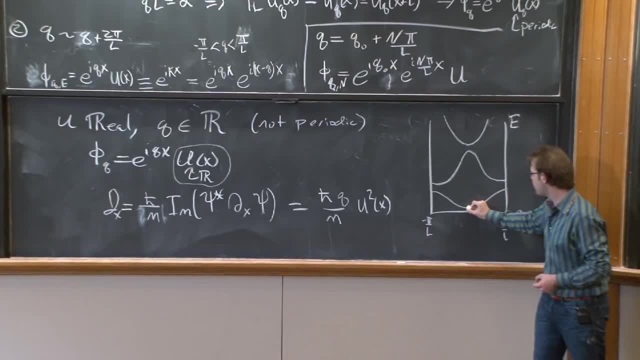 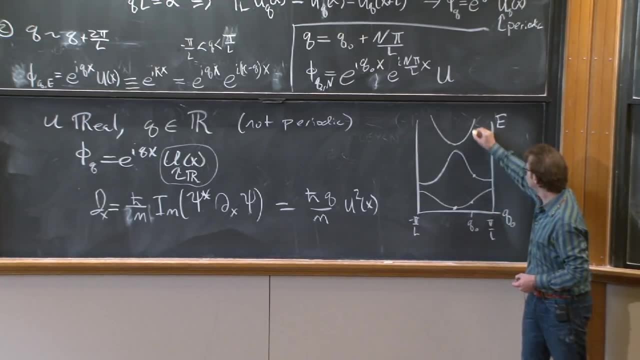 In fact the set of allowed states or energy eigenvalues for an allowed value of q, let's say this particular value of q0, how many of them are there? Well, there are as many as there are integers 1,, 2,, 3,, 4 count. 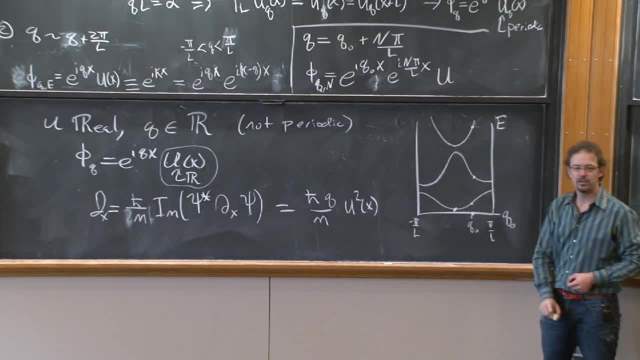 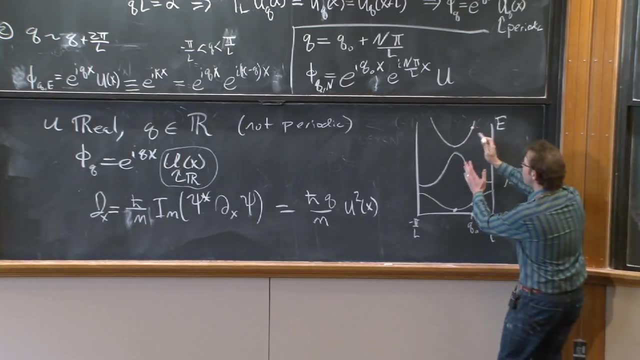 So to specify a state, I don't just have to specify q0.. I also have to specify n, Which one of these guys I'm hitting. And when you unfold this into the parabola picture, remember where these came from. These came from these curves came from shifting over. 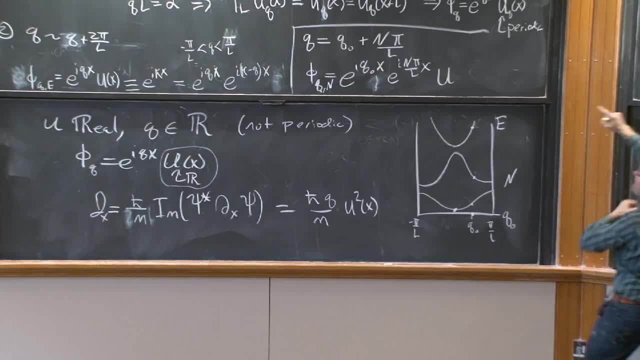 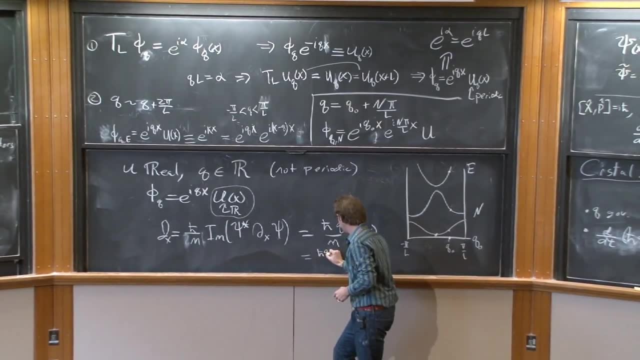 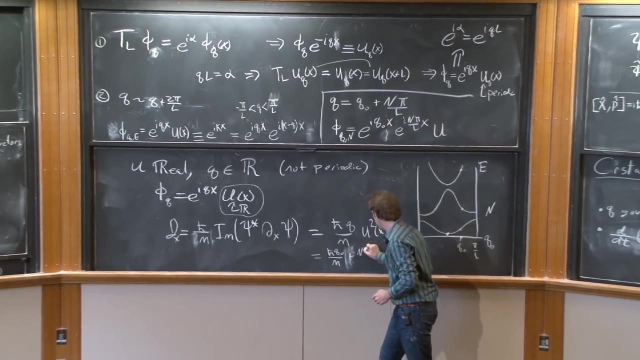 And the higher up you go, the more you had to shift over. And that's exactly the integer piece n pi over L, And so we can write the current now in terms of h bar q0 upon m u squared, oh sorry, h bar q0 upon m plus n pi h bar q0.. 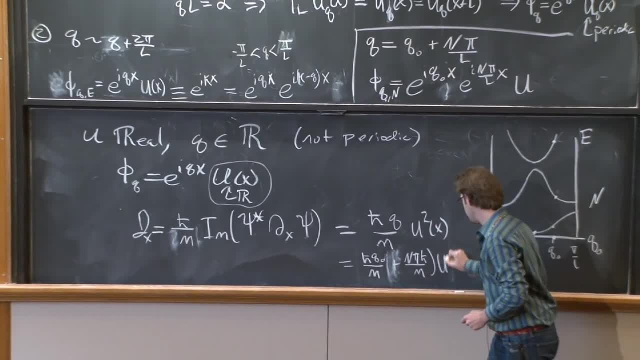 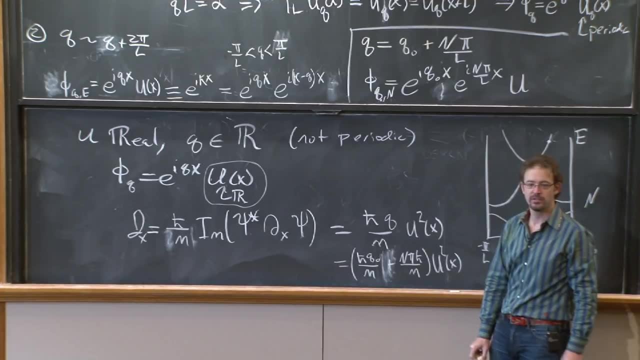 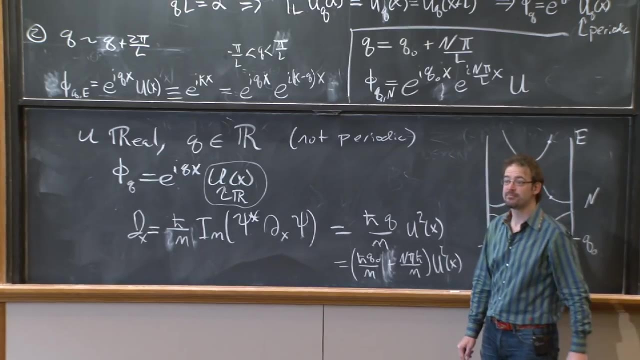 h bar upon m? u squared of x. So we get a contribution from the crystal momentum and from which band we're in. OK, So it's sort of an elaborate story to answer the phase question. Yeah, Why did we use the q squared? 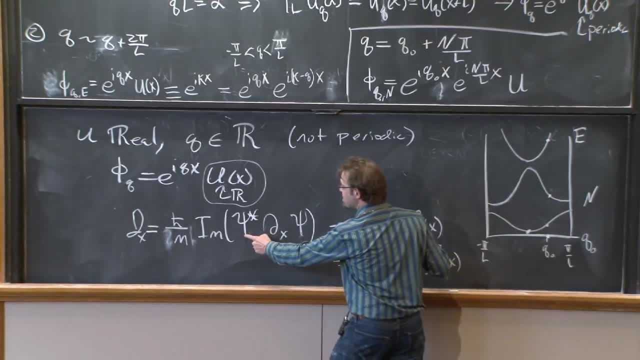 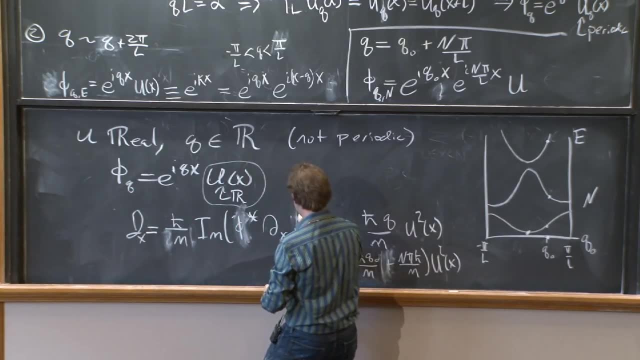 Why did we use the derivative of x? Good, So here we had psi. oh sorry, I should have done this for phi. I meant this wave function, Right, OK, So this is phi. this is phi. q, q. 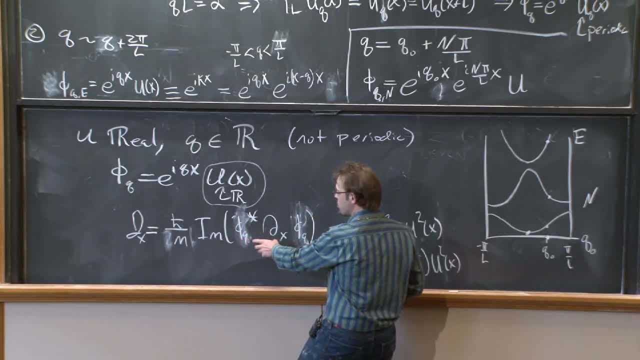 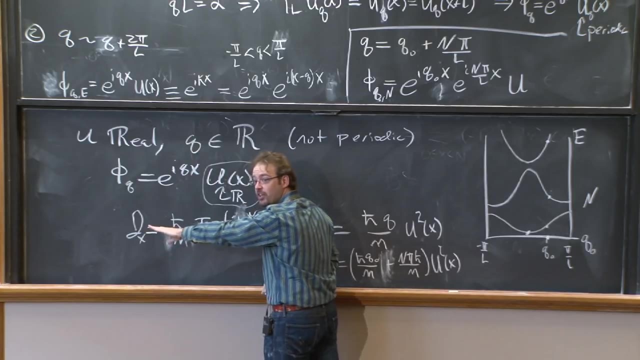 So from here we're going to get the imaginary part of this wave function, which is e to the minus iqx? u of x, derivative of e to the iqx? u of x. Now the term that contributes is when the derivative hits the e to the iq. x pulls down a factor of iq. 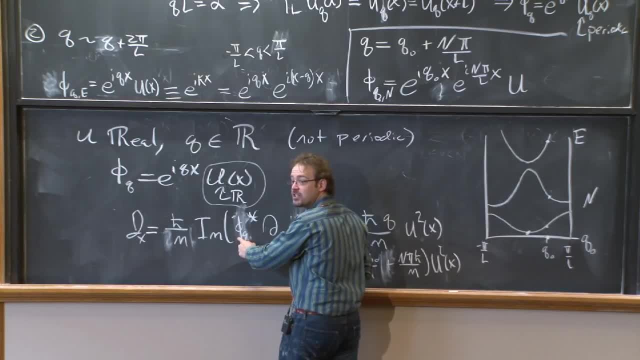 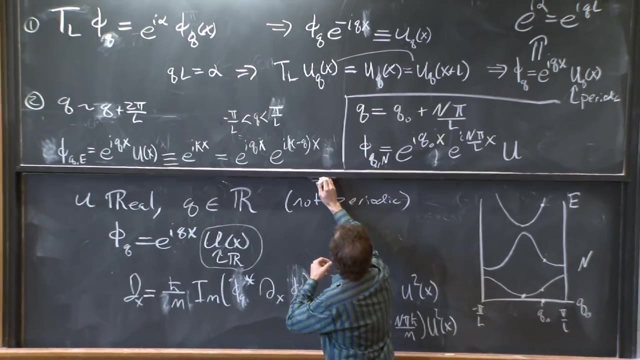 and the two phases cancel from these guys, leaving us with a u of x here and a u of x here. Oh sorry, this isn't the potential. Ah, good, That's the point. So this isn't the potential. So in the statement that when we have this translation by x. 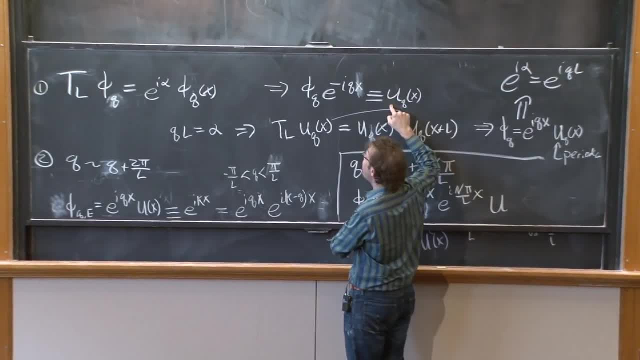 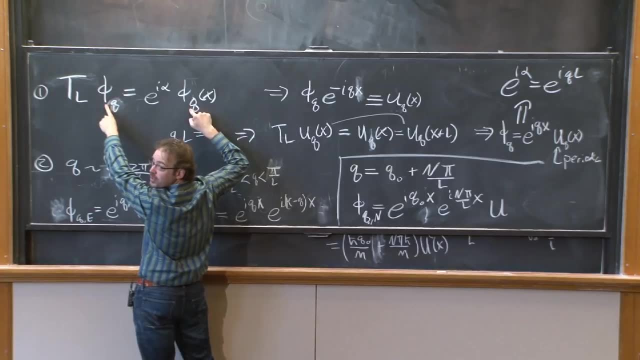 so this is just some function. It has nothing to do with the potential. It's defined in terms of the wave function, the eigenfunction of translate by l. So if we know, so the logic here goes: if we know, we have an eigenfunction of translate. 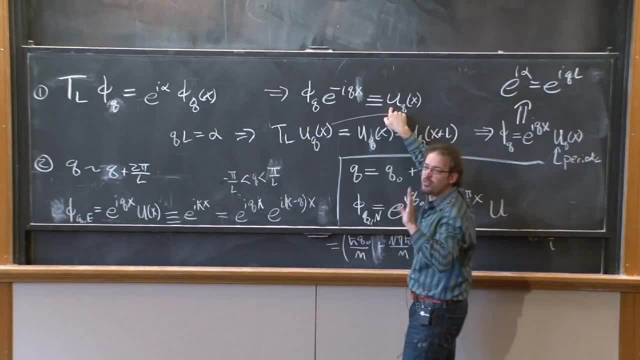 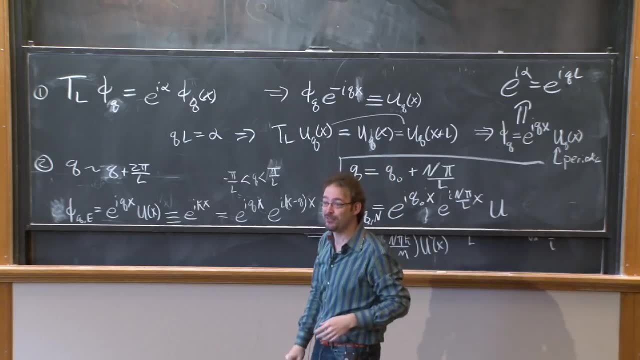 by l. then I construct a new function, u. nothing to do with the potential, just a new function which is e to the minus iqx times it. You can't stop me. You hand me a function, I will hand you a different function. 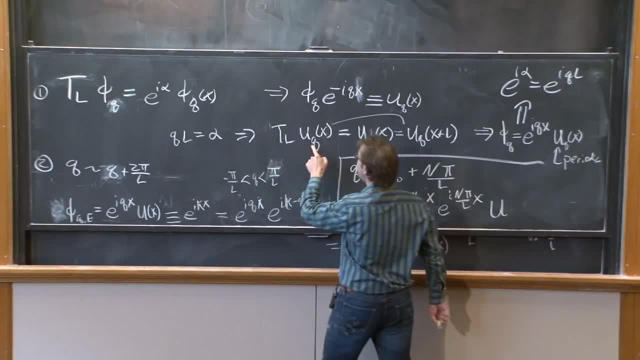 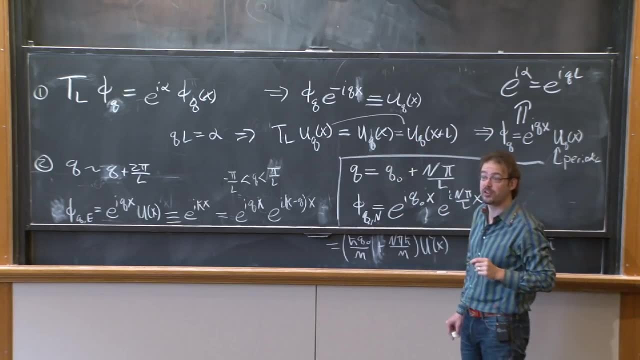 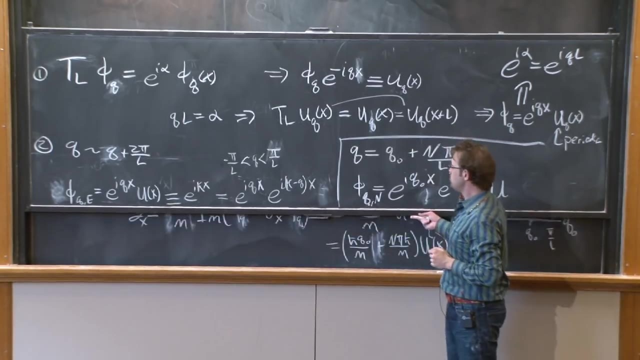 And then we pick q, felicitously, to show that u is periodic. So u is just some periodic function which is contained, which is defined from the wave function, from the eigenfunction of TL. Did that answer your question? OK, So here, it just came from the fact. 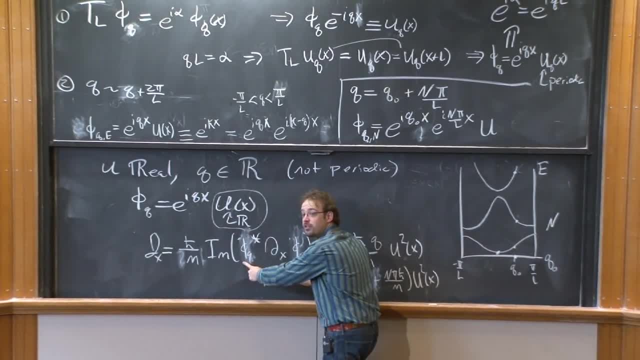 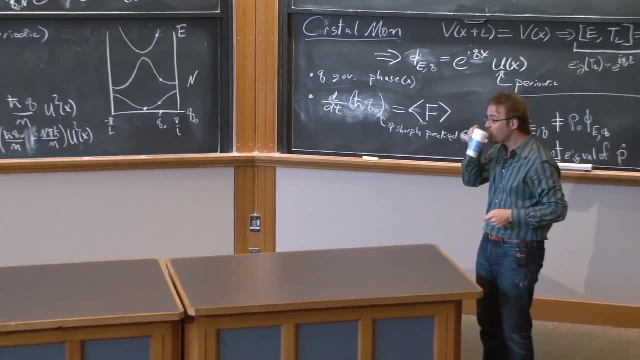 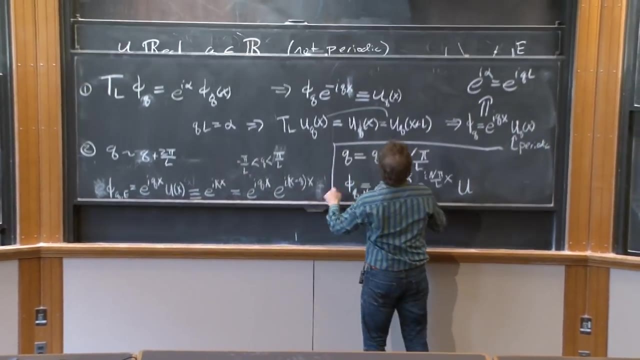 that u is phi, is e to the iqx u, and then there's a factor of u from each of these Other questions. Yeah, What does that picture actually look like when you unfold it? It's kind of awesome. So this picture when it's unfolded, first off. 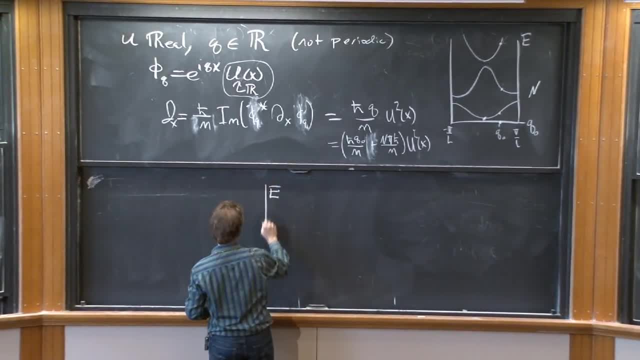 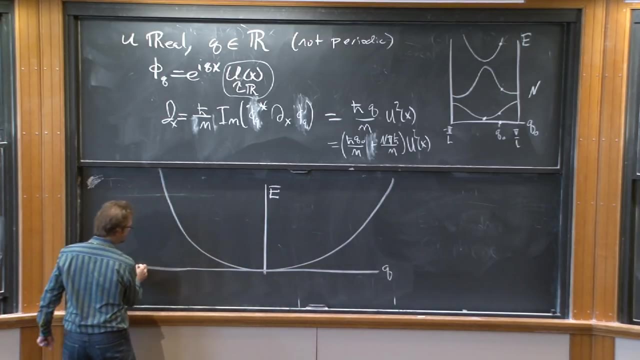 you know what it is for a free particle. So we want the energy as a function of q. So what is it for a free particle? Parabola, Parabola, Yeah, exactly. And now let's add in the, let's make this: 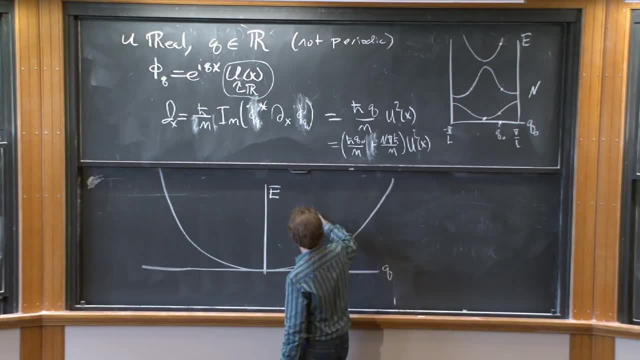 this is a function of q, not q0.. So here's pi over l, Here's 2 pi over l, Here's 3 pi over l, And I need to do this carefully because it's incredibly difficult to get this straight. 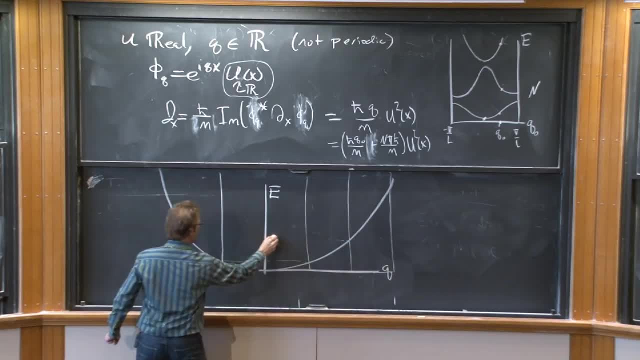 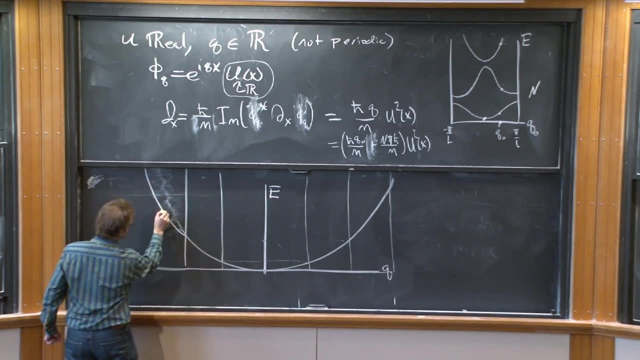 OK, Call that and then. OK, My artistic skills are not exactly the thing of legend. OK, So here's the parabola that would have been if we had not turned on a periodic potential. As we turn on the periodic potential, 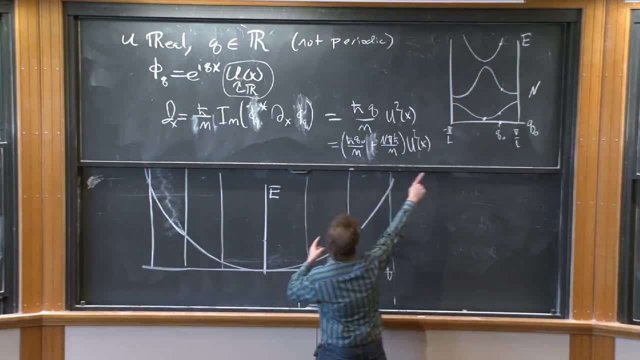 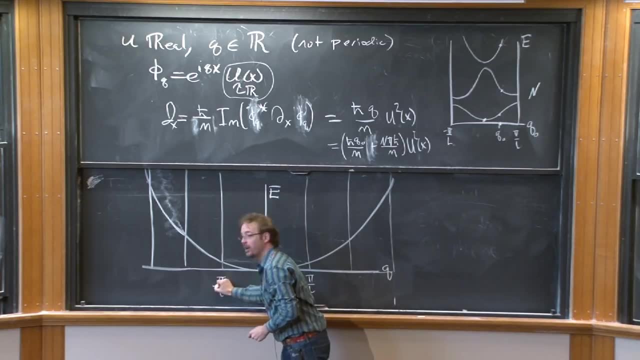 we know that the energies, the allowed energies, change, And so in the first band it's easy to see, because from minus pi over l to pi over l, we don't have to do anything. Pi over l minus. So it looks exactly the same as the lowest band here. 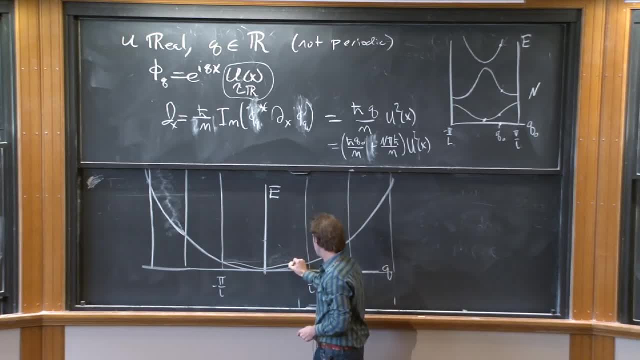 So in particular. OK, So what about the second band? Well, I want to know what's the other allowed energy at, say, plus pi over l. So at plus pi over l, it's going to be something greater than this value. 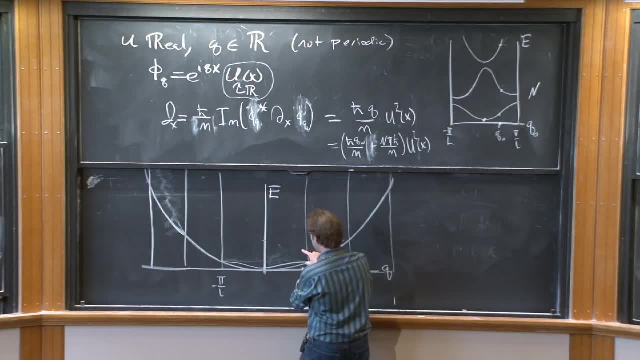 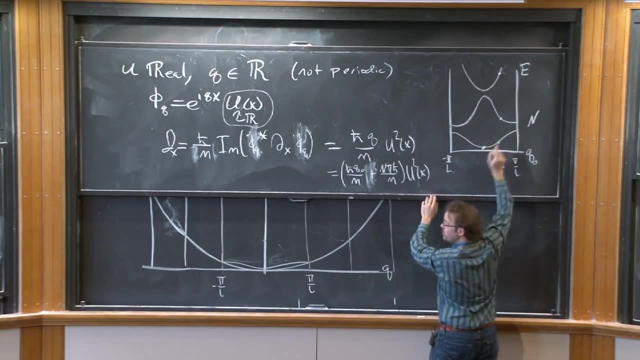 But plus pi over l? we already know the answer from that diagram, because plus pi over l is the same as minus pi over l. So what's the value over here? Well, the value over there for the second band is slightly above, and then it increases and decreases. 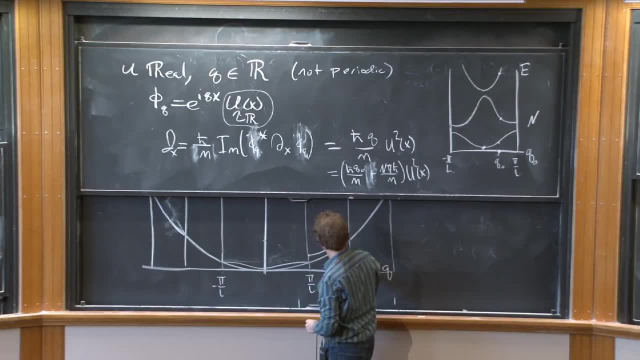 So slightly above. and then it increases. Shift by pi over l. Did I shift by pi over l, this guy? That's one, two. Yes, I did, Good, OK, And it goes the other way. So just noting that it goes the other way from the top. 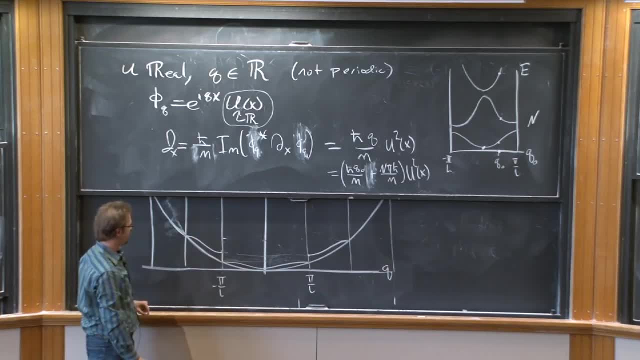 I have a hard time drawing these things. OK, So for every value of q there's an allowed energy, But it's different than it would have been for the free particle. And then we do the same thing. for the next thing, We do the same state. 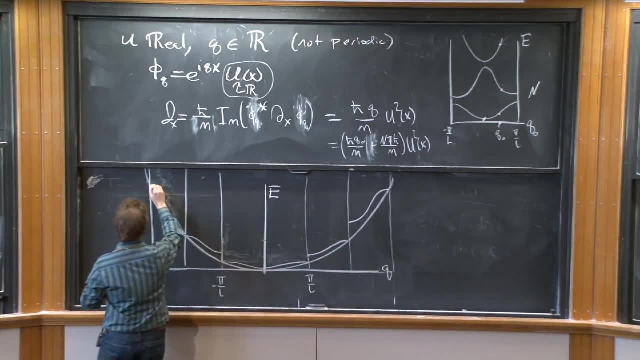 And it looks like this. So now imagine what happens. We take this and we fold it over One, two. What we get is a band that should look like this. That's what the second band should look like, And indeed, when we put it in the fundamental domain, 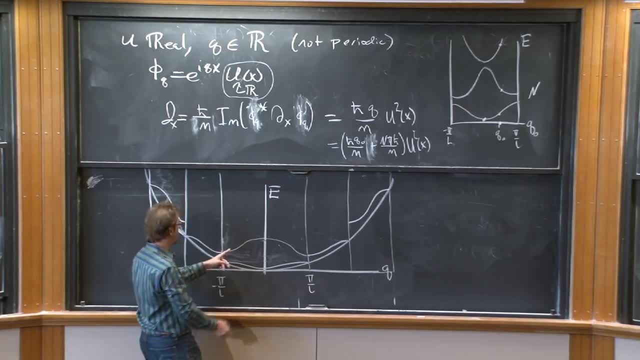 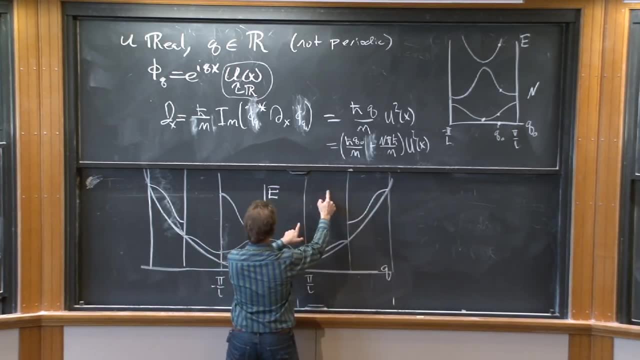 this is what we get. This is what the first band and the second band together look like, And then the third band. we'll move this over once and then twice. It's going to look like this: And this guy move it over once, twice. 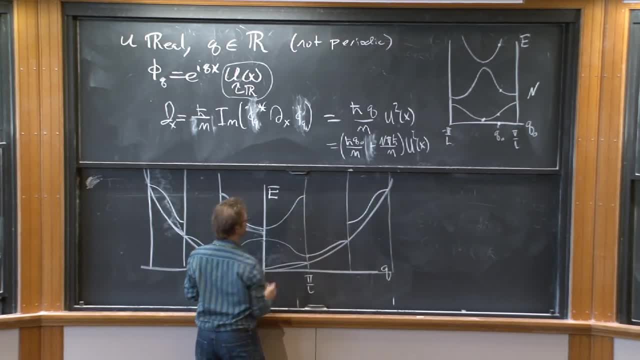 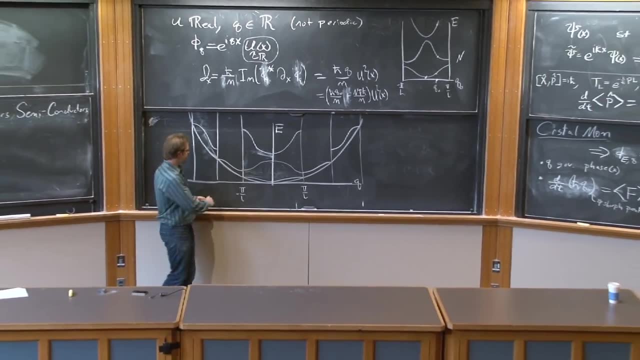 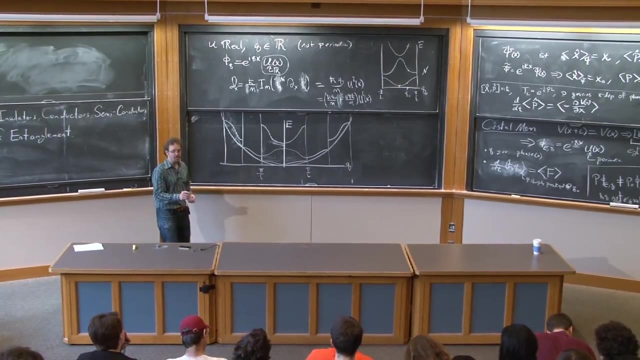 Looks like whoops, Good Yeah. So if we wanted to plot v with respect to k instead, would that just be a parabola with dotted lines? And if so, why do we not ever like If we just wanted to plot? sorry, say again. 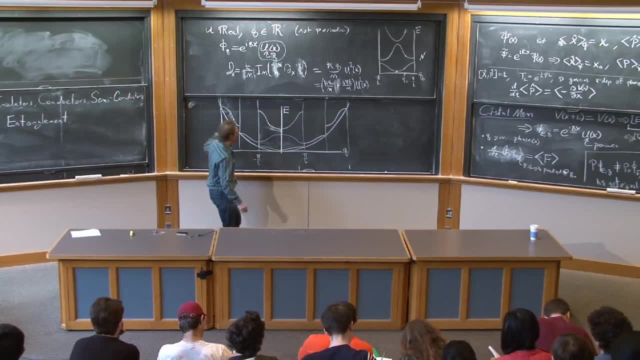 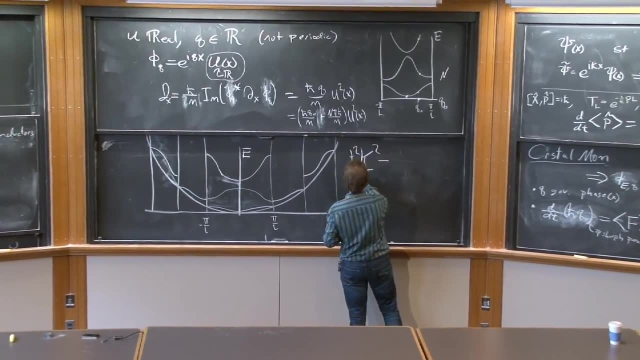 e as a function of k instead of q. Oh yeah, e as a function of k is always going to look like that, But k is not a. well, so what is k? k is just defined as h bar squared. k squared upon 2m is equal to e. 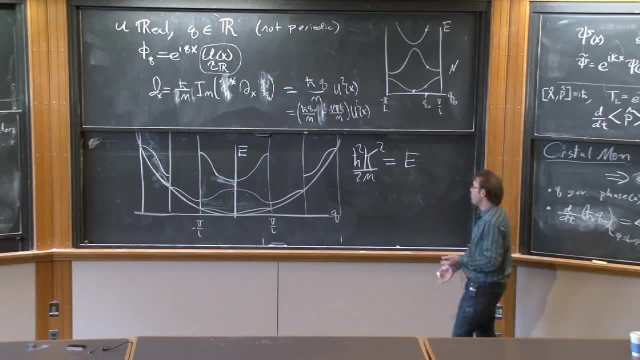 So this doesn't tell you anything, right? Because any allowed k- OK, sure, any allowed k- is some valid value of e, but this doesn't tell you which values of e are allowed. Only some values of e are allowed, right. 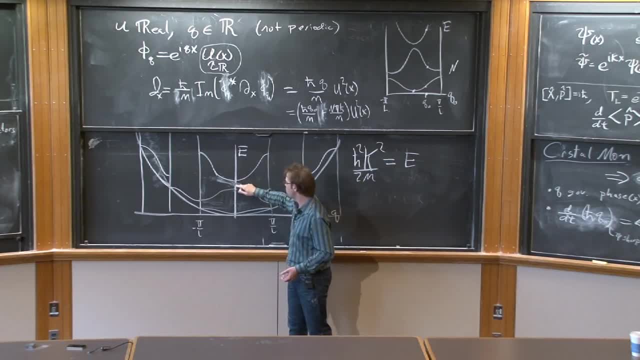 There are no values of e, there are no energy eigenstates with energy in between here and here, right. And so that tells you there are no allowed k's, because k is just defined, It's just completely defined by e. So this doesn't tell you anything. 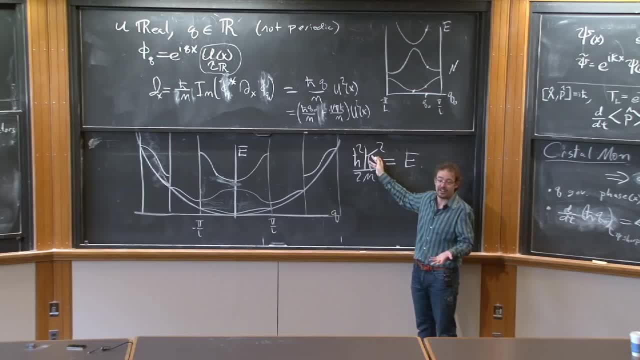 about which states are allowed. It just tells you that, given an e, there's some, you know some quantity. I could define k. This is a definition of k in terms of e. What this diagram is telling you is which e's are allowed. 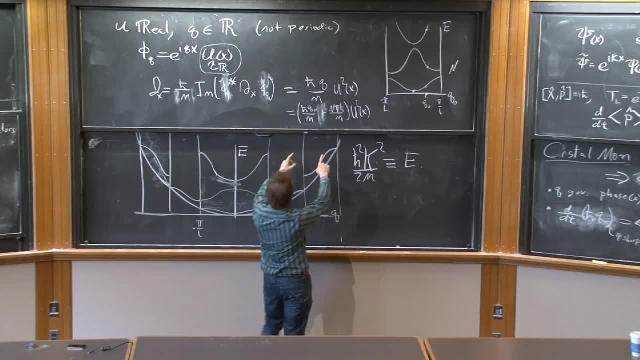 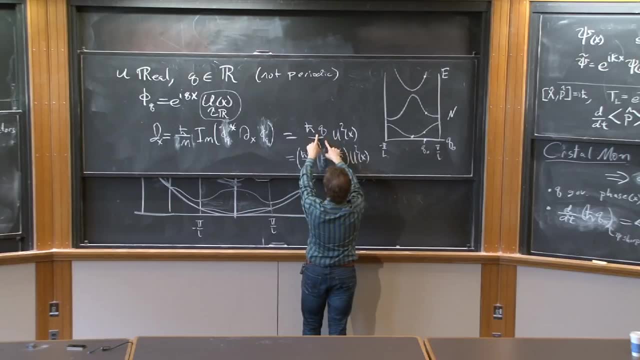 Sorry, say again, If you see an l in the second term of your current, that's where you're at. An l Yeah Or q Yes. yes, there should be a yes, Let's see, let's q. sorry, oh, here, yes. 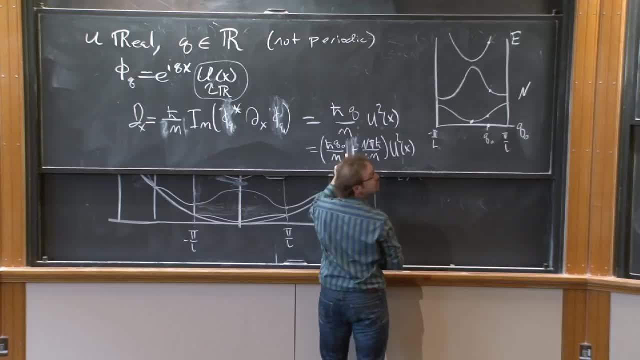 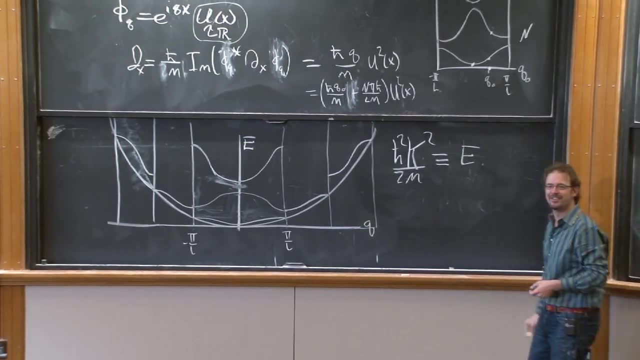 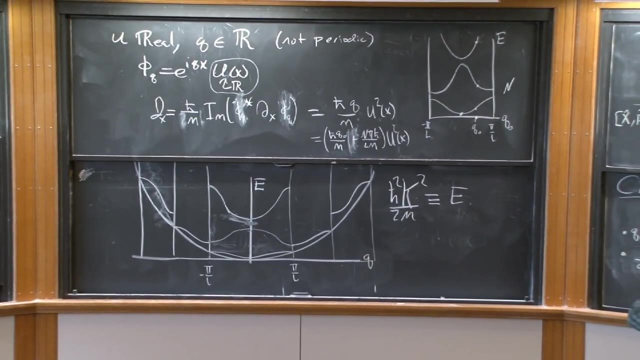 Yeah, you're absolutely right Over l Over l. thank you Excellent, that's exactly right. yeah, Oh man, I made a dimensional mistake. thank you, Jesus, OK, good, yeah, Another question. could you re-explain? 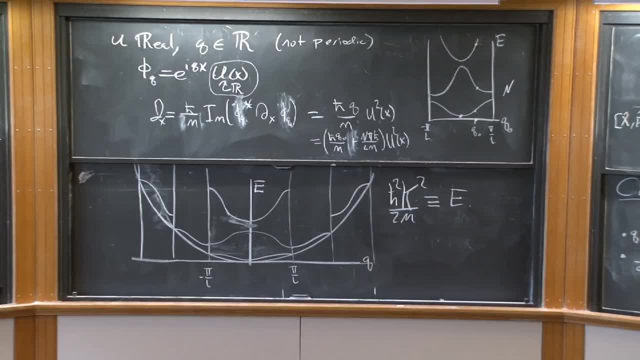 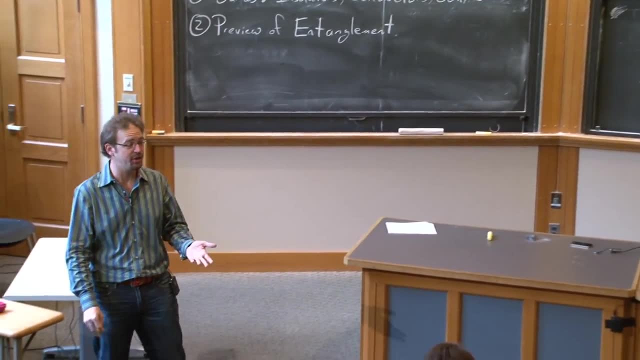 how imperfections in a lattice actually contribute to the conduction process. Yeah, I'm going to do that, So that's an excellent question. So the question is: could you explain again how imperfections in a lattice lead to actual conduction? 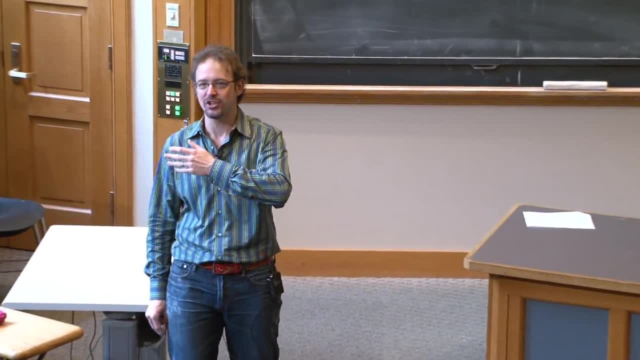 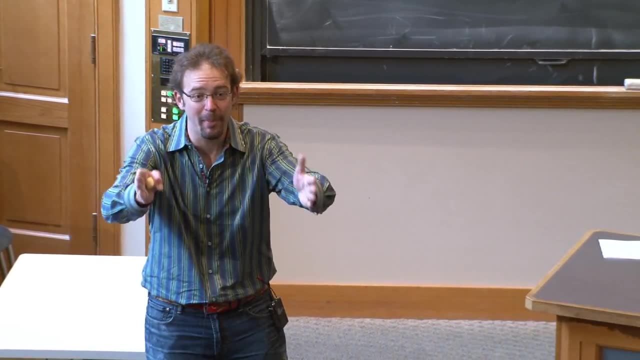 As we talked about last time, when you have a perfect lattice, there is actually no current flowing in response to an applied electromagnetic field. If you put on a capacitor plate across your perfect lattice, you don't get any current, The particle, the charged particle- in your lattice. 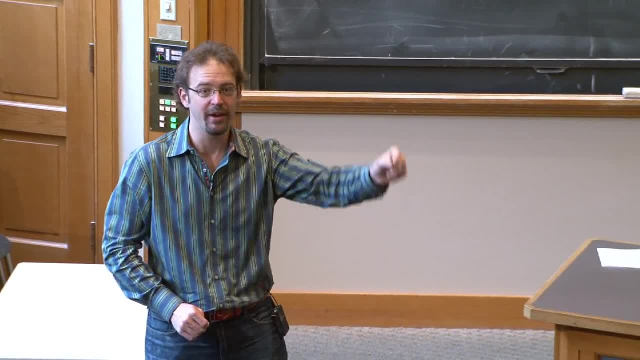 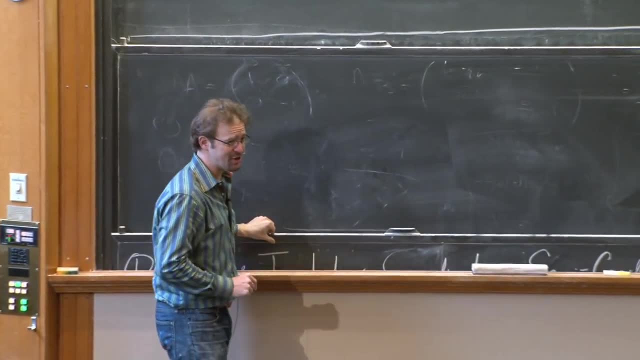 just oscillates back and forth in a block oscillation, running up the band and down the band, up the band and down the band. So how does that? so let me slightly change your question and turn it into two other questions. The first question is, given that, that's obviously not. 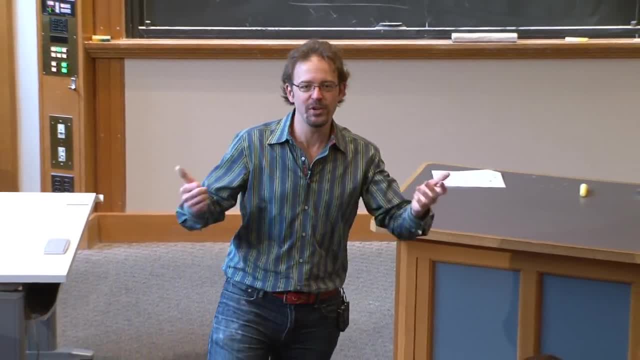 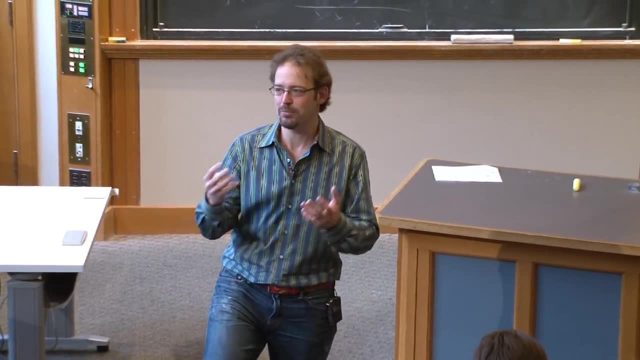 what happens in real materials? why don't we just give up on quantum mechanics and say it totally failed? And so this is a totally reasonable question, and I want to emphasize something important to you, which is the following: That model led to a prediction which 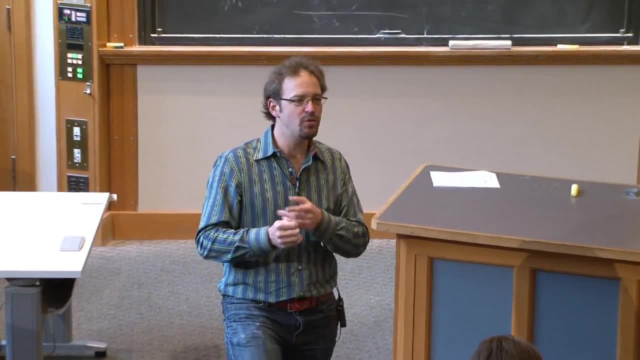 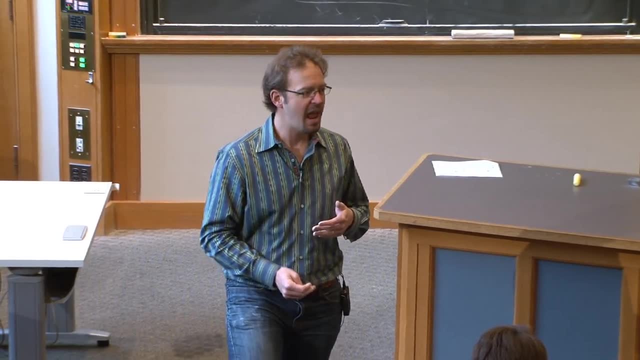 is that if you put a capacitor plate across a perfect crystal, then you would get no current flowing across. you would just see that the electron wave packets oscillate, a la block oscillations, as discussed last time, And that is manifestly not what happens with copper. 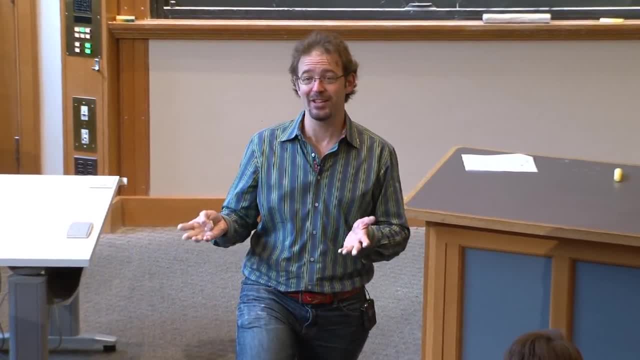 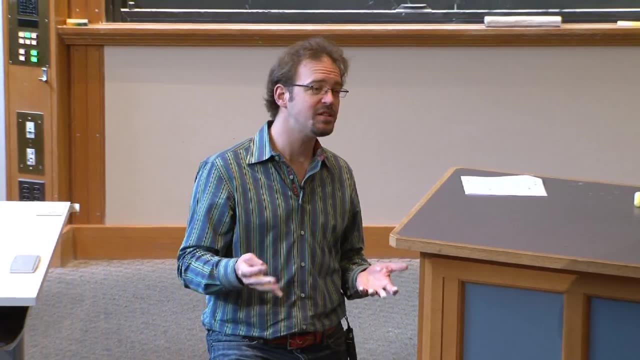 But the experimentalist comes back to you and says: look, dude, that is a ridiculous model, because the copper isn't in fact perfect, It's messy. So how do you test the model? Well, there are two ways to deal with the situation. 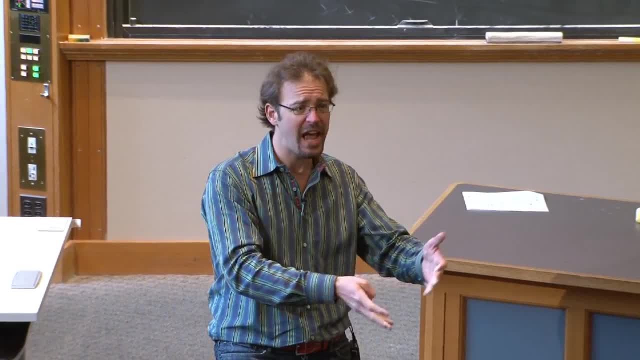 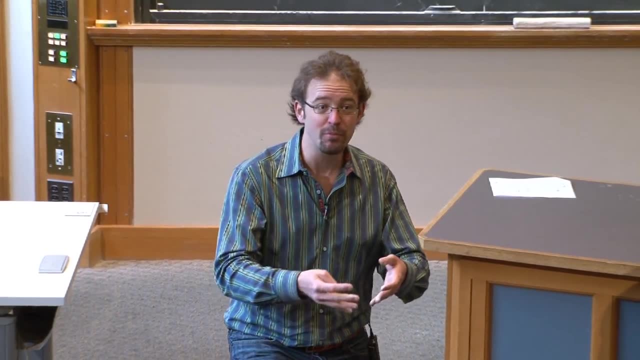 One is you improve the model to incorporate properties that copper actually has and see if you can actually get the same conductivity that you see. But the other is you could improve the material instead of improving the theory. So let's make a. can we actually build a perfect crystal? 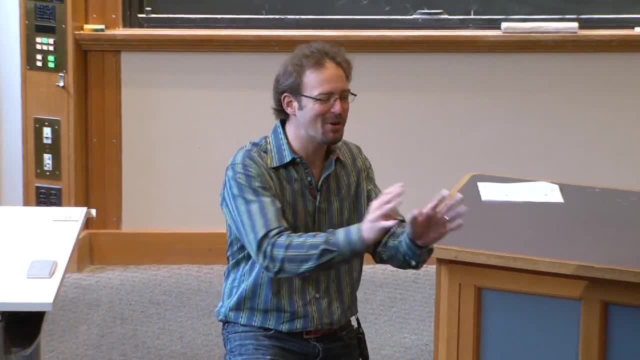 So this is actually something that's something that I'm doing research on right now, and not on the building side, but on the theory side, because I'm a theorist and you should not let me in a lab, But I collaborate with experimentalists. 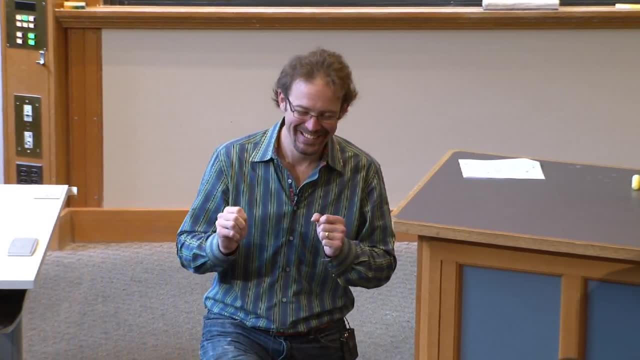 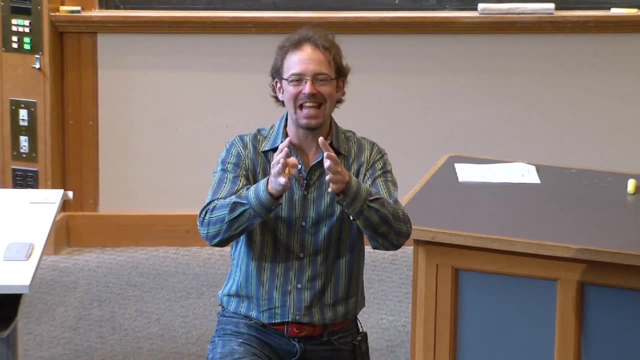 So they're nice people, Very good physicists. So here's something you can do. You can build a system that has exactly a periodic potential. It turns out it's very difficult to do this with quantum systems, but what you can do is you. 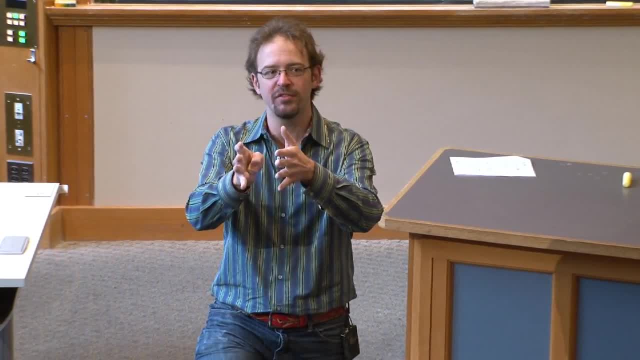 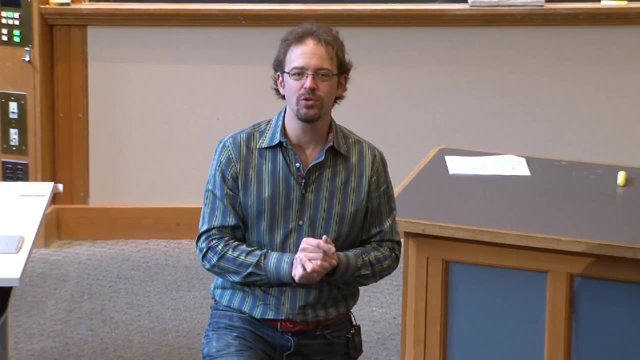 can do it with lattices not of Atoms, but lattices of dielectric. So the equation- here's a cool fact- the equation for light going through a dielectric, where the dielectric has different constant, like wave guides, you've got glass. 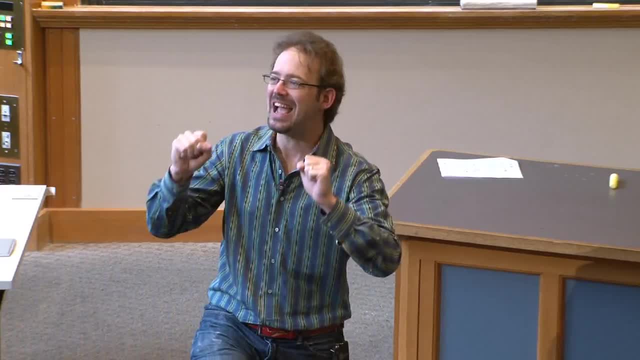 you've got air. you've got glass. you've got air. That equation can be put in exactly the same form as a Schrodinger equation for the time evolution of a wave function. They're both waves and so it's not so surprising. 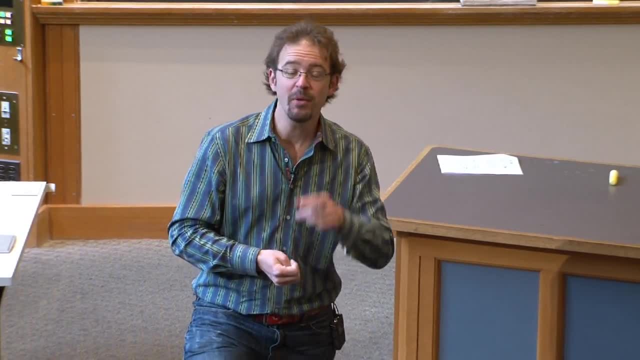 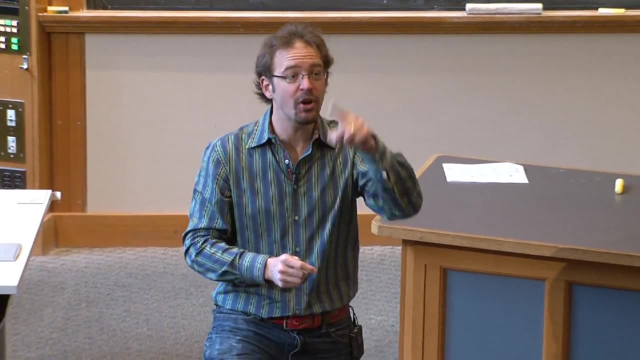 these two wave equations are related to each other in a nice way. Meanwhile, the index of the dielectric turns into is the potential for the quantum mechanical problem. So if you have a periodic potential, what do you want? You want a periodic dielectric constant. 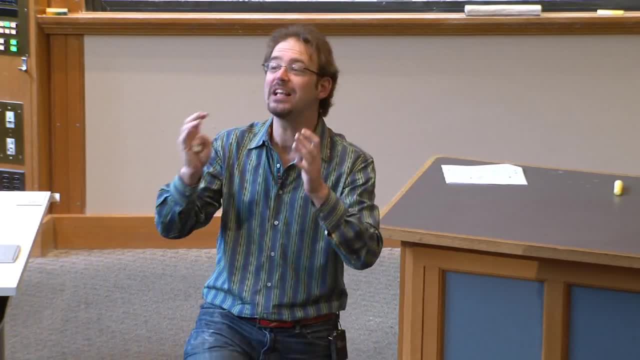 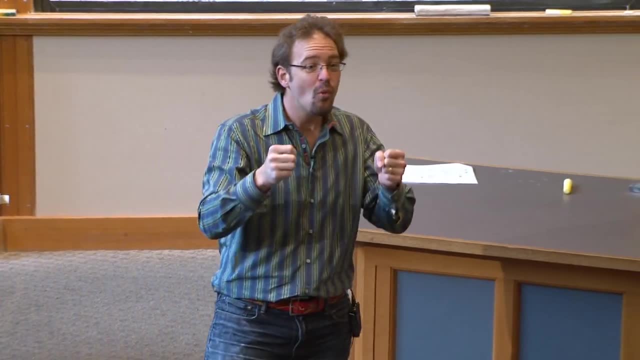 Yeah, And so you can build a system which incredibly cleanly has a periodic dielectric constant and no disorder, And then you can put light into the system and you can ask what happens to this system. So here's the idea. I take a system which is a periodic potential. 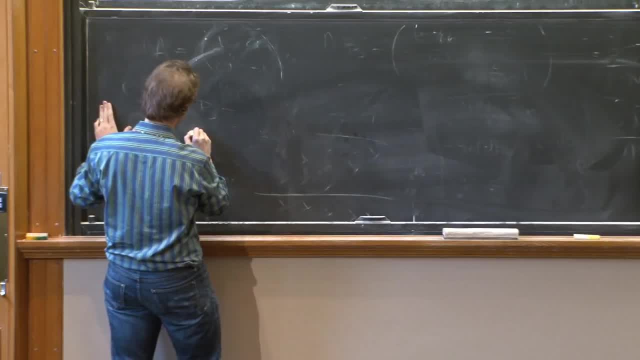 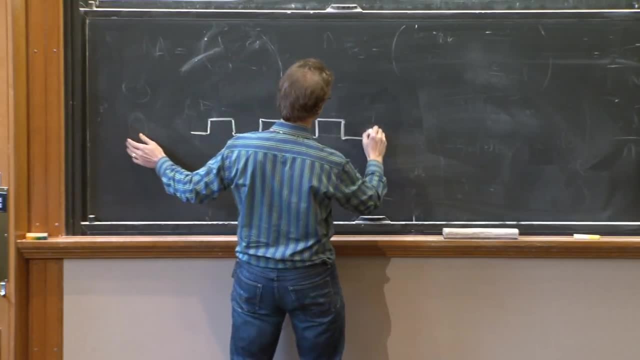 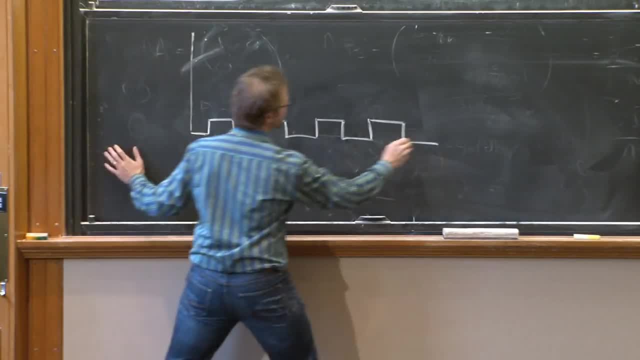 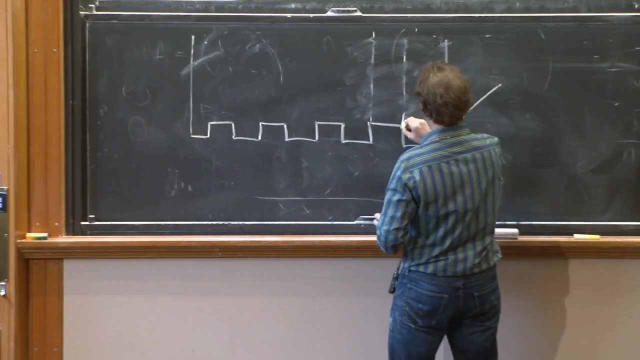 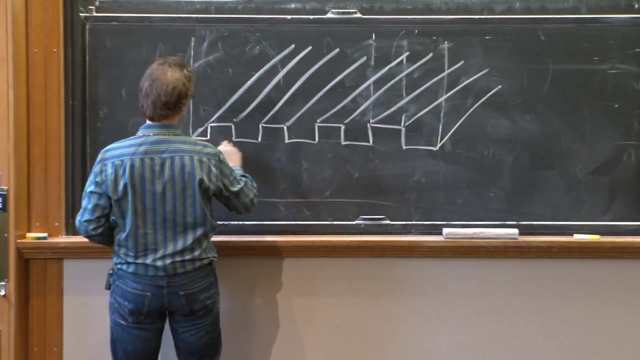 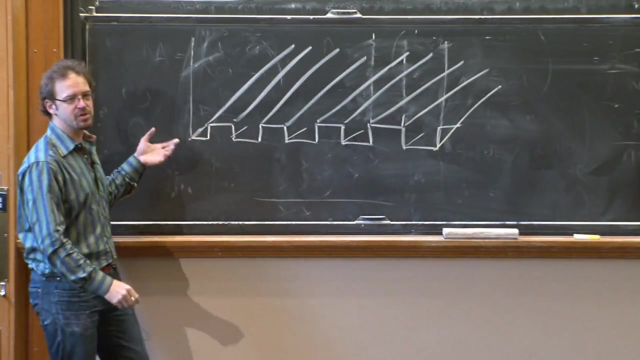 But instead of having it be a one-dimensional lattice, I'm going to make it a two-dimensional lattice. So now, basically, I've got a set of wave guides. Let me draw this slightly differently. So does everyone get the picture here? So literally what you have is you have glass, glass. 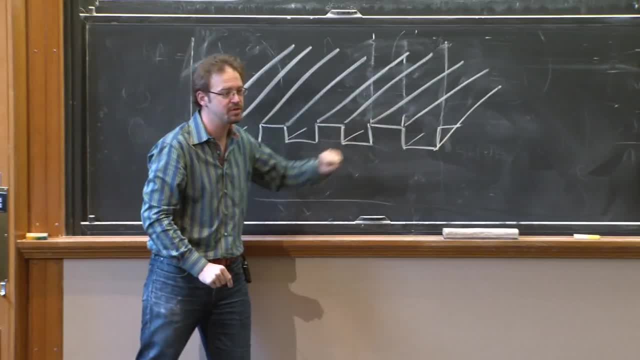 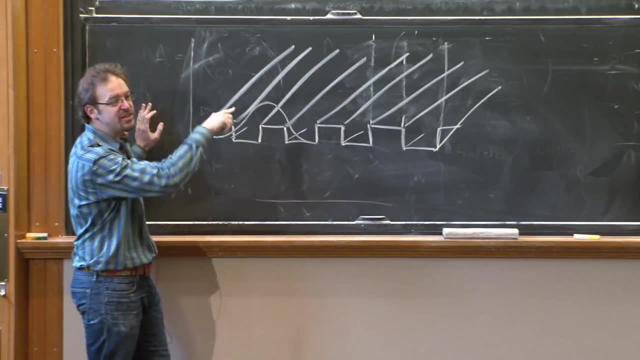 with a different index, glass glass with a different index. You can think of this as a line of glass fibers, of optical fibers, And you shine in light that's reasonably well localized in both position and in phase variation or crystal momentum. 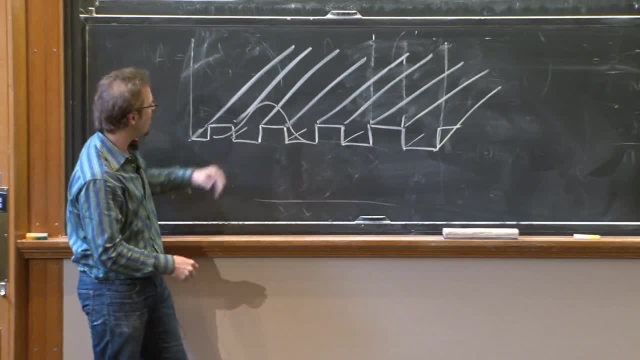 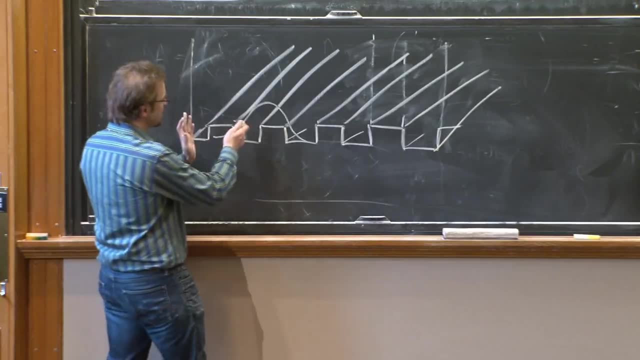 because you can control the phase of the light. So you send this wave packet and you ask: what happens? Well, not a whole lot happens. It's a wave packet, It's going through a wave guide, But we haven't implemented an electric field. 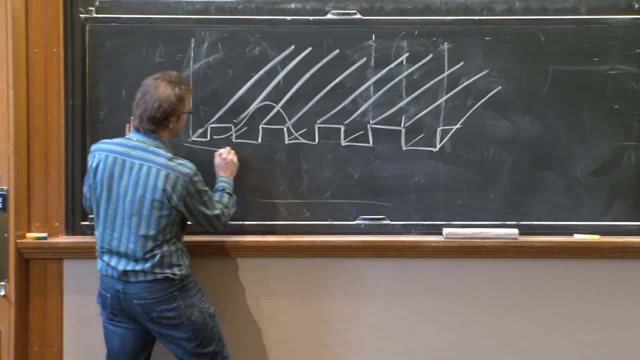 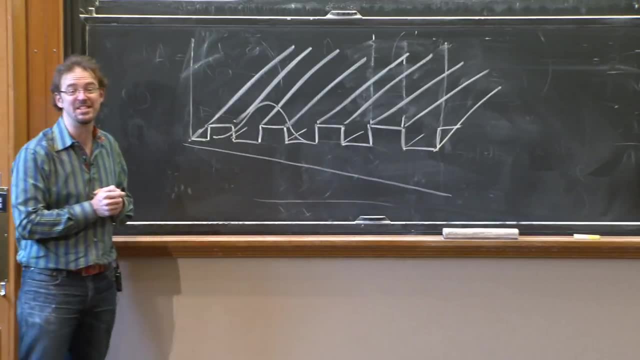 To implement an electric field, you need the potential to be constantly varying. So let's add a linear ramp into the potential Instead of making it just perfectly periodic. let's make the index ramp just a little bit, And this experiment has been done. 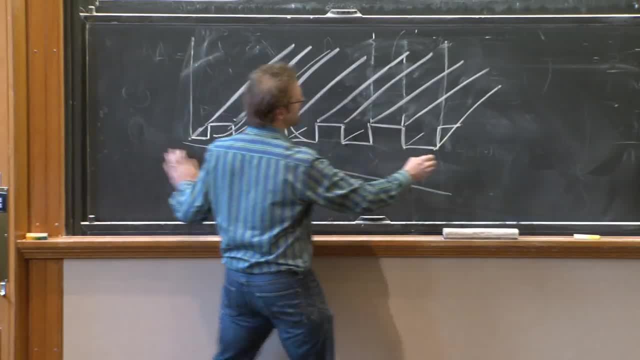 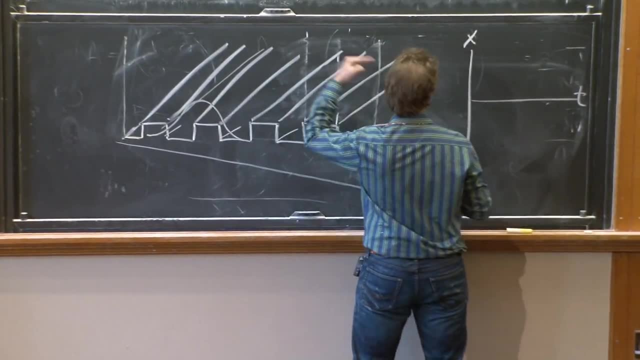 And this experiment, so as the wave packet moves along, what's discovered is that the position, if I draw the x as a function of t, so now the role of t is being played by the distance it's moved along the wave guide what you find. 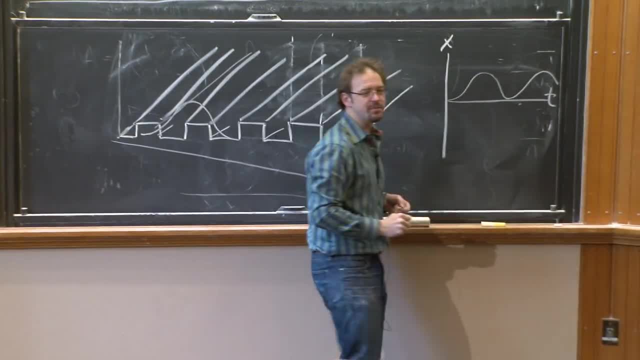 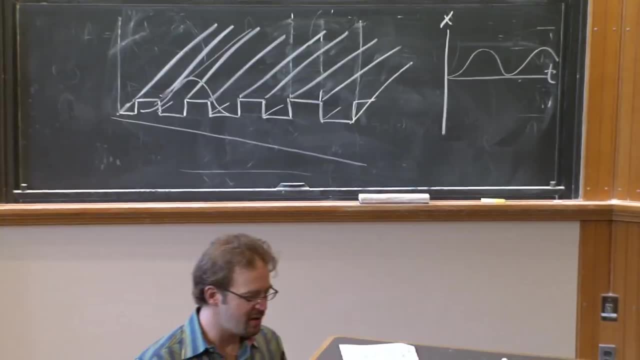 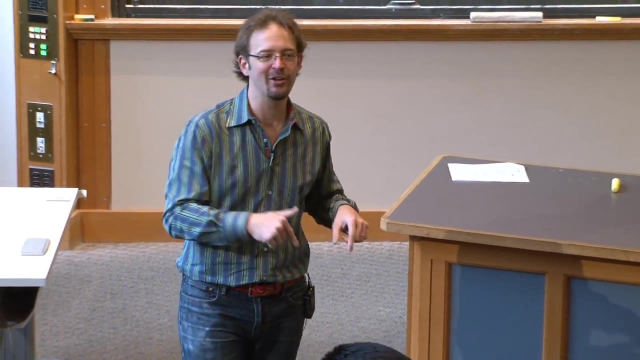 is. it does this: It exhibits beautiful block oscillations And this has been probed in a very small number of real, honest quantum mechanical systems. The most elegant experiment that I know of was done by Wolfgang Ketterle, who's here at MIT. 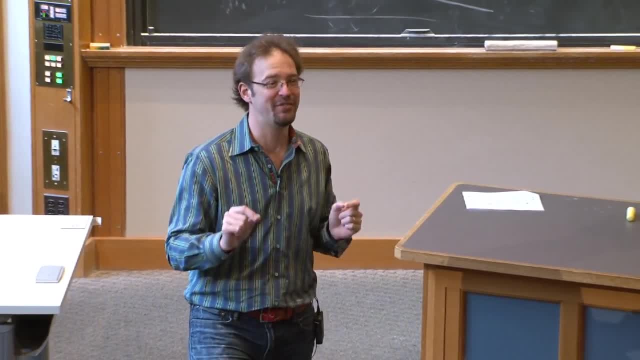 And he got three data points because it was preposterously difficult, and declared victory. So I talked to him about this in the hallway one day. He said, yes, this was ridiculous, But we got three data points. We got small, We got large. 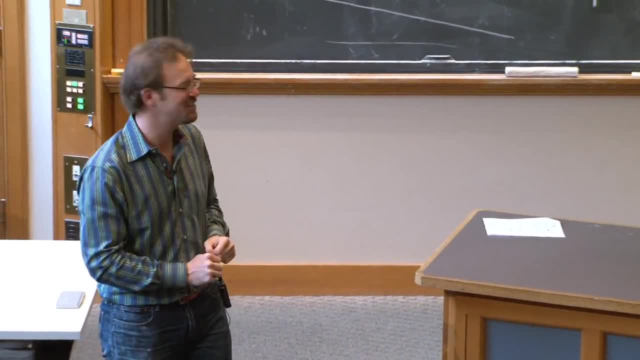 And victory. We declared victory, But it really needs to be done well. So one of the interesting questions in this part of the field right now is: we know that it's true, but we want to see it, We want to feel it. 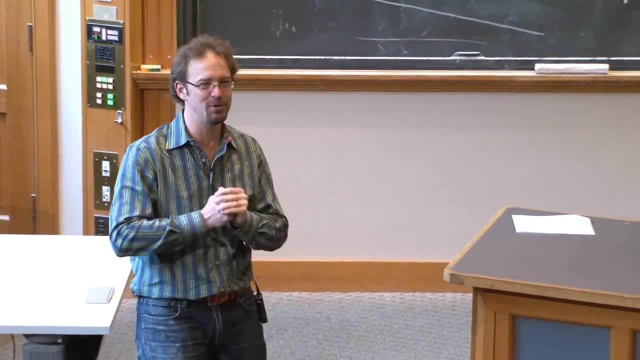 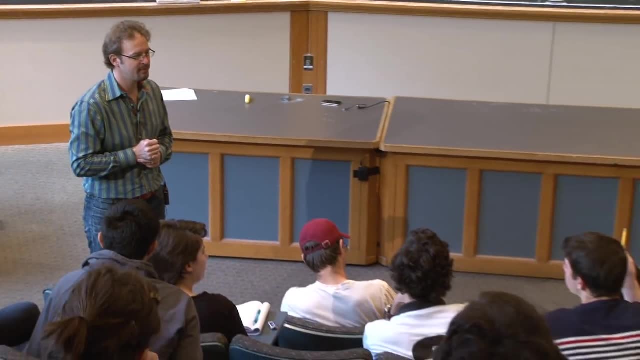 So various people around the world are working on making a truly beautiful demonstration of this bit of physics. Yeah, If you truly get these oscillations, is this or is this not like a wave doing quantum memory? Is it a- Oh, is it an impractical, impractical wave? 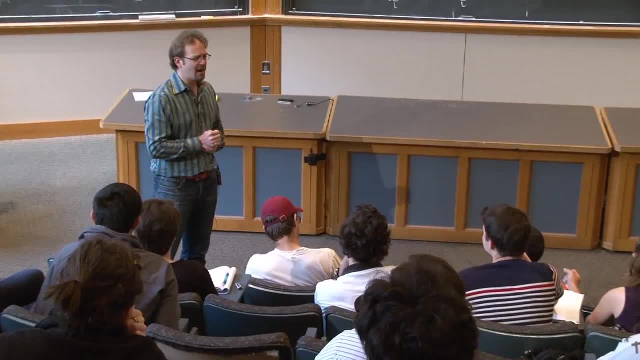 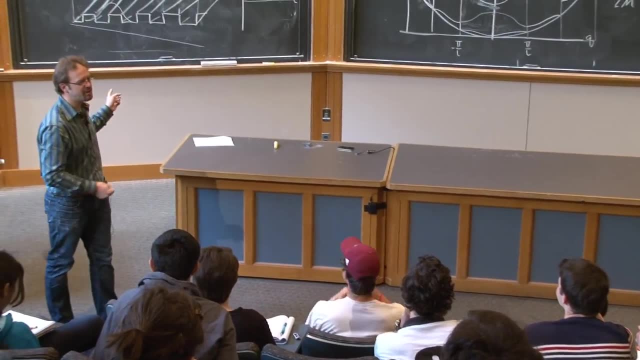 doing quantum memory Like if you want to. It's totally impractical because any interference is just going to kill you, unfortunately. So you have to work ridiculously hard to make systems clean. So the question is really a question about quantum computation, which we'll come to next week. 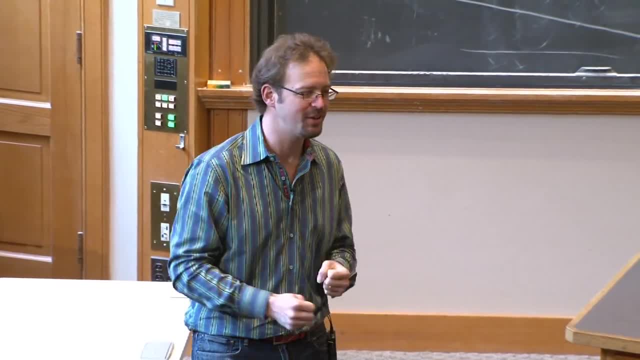 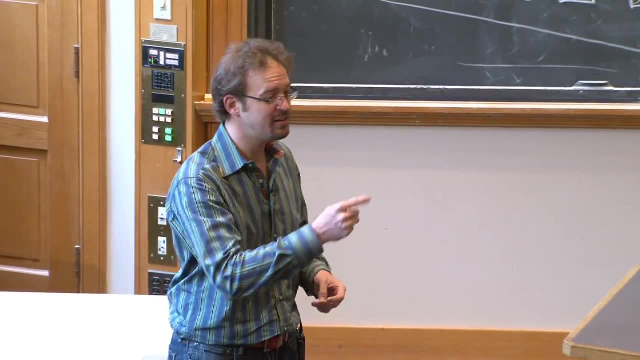 But the basic question is: how robust is this? And the answer is it's not robust at all, But which you can tell? because everything in the real world has enough impurity that it conducts or is an insulator. Yeah, What plays the larger role in the perfection? 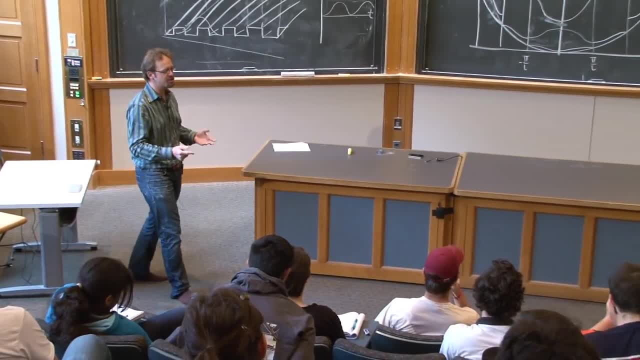 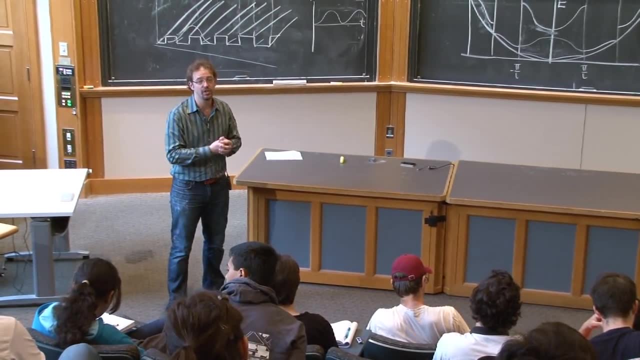 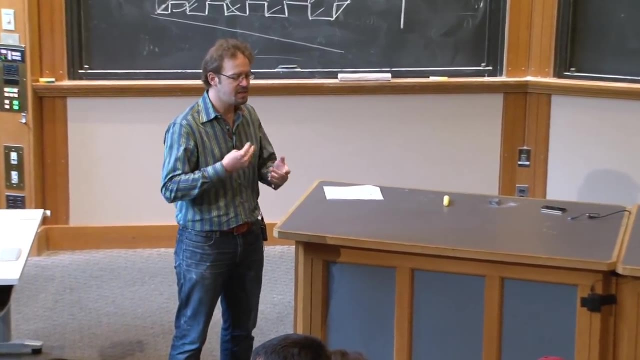 of a lattice, like temperature or impurity. That's a very good question. So the question is: what's the most important disordering property that leads to conduction And there's temperature fluctuations, There are impurities in the lattice, There are decohering effects, which 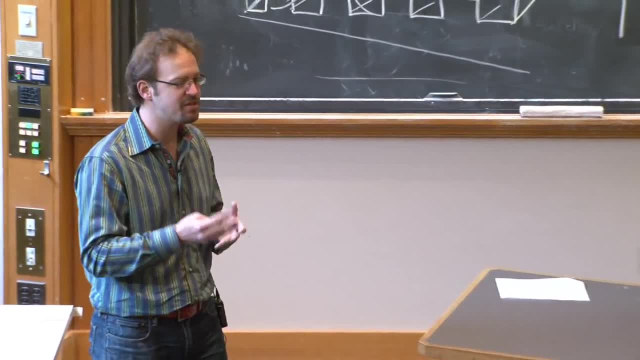 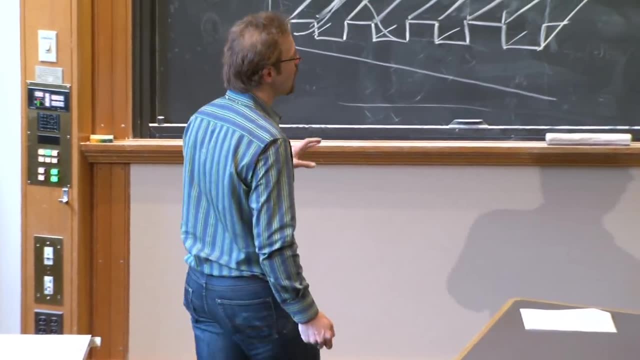 is a more complicated story, And it depends on the situation, depends on the system, And exactly how it depends is something that is an active area of research. Now, there are many, many ways to probe this physics, So we know that these block oscillations are true. 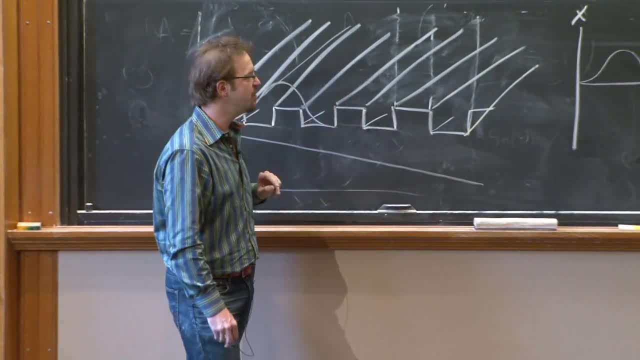 And we see them in all sorts of different systems. There are systems that are analogous, So there's lots of experiments. It's not like this is an ambiguous bit of physics, But it's one that turns out to be surprisingly difficult to tease apart. 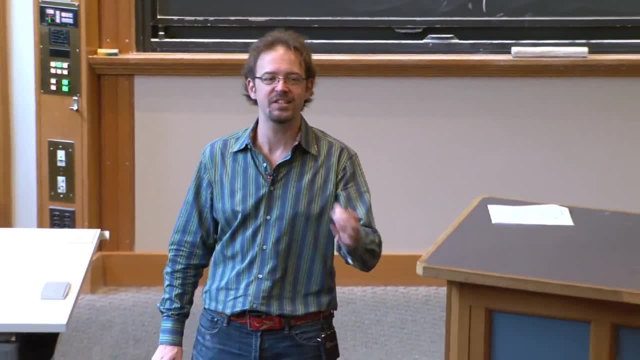 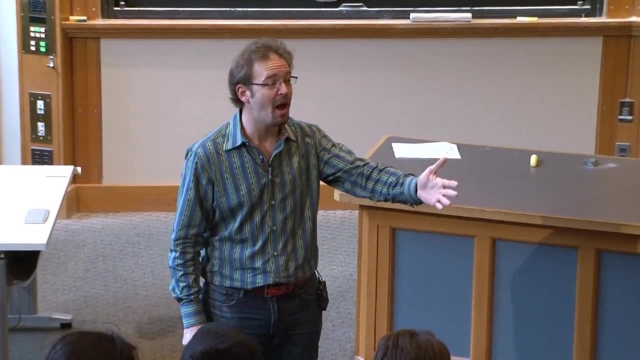 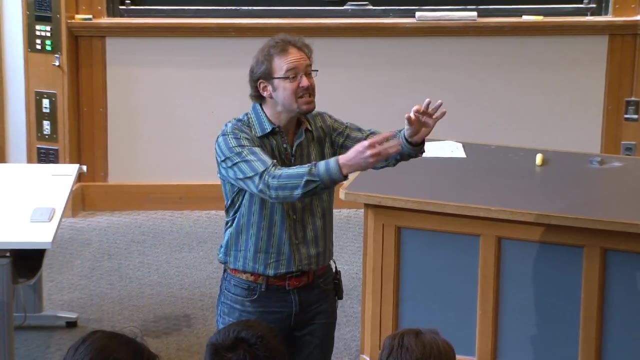 The reason I bring all this up is to emphasize the following: Our model made a prediction that disagreed explicitly with the conductivity property of copper and other materials. So don't throw away the model. Observe that you've modeled the wrong system If you find a system that shares the assumptions of your model. 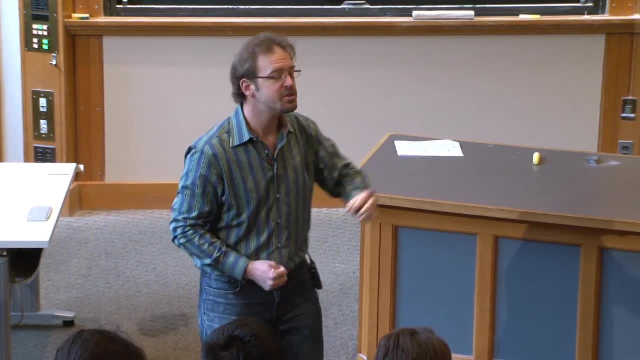 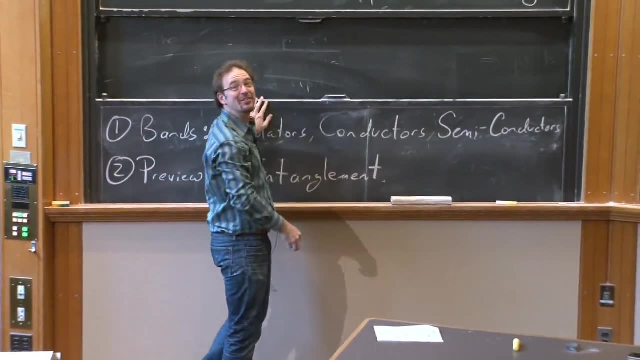 that's when you ask: did it work? And it worked like a champ. So now let's talk about real materials. This is going to close up our discussion of bands and solids, And this is actually what I wanted to get to at the beginning of the lecture. 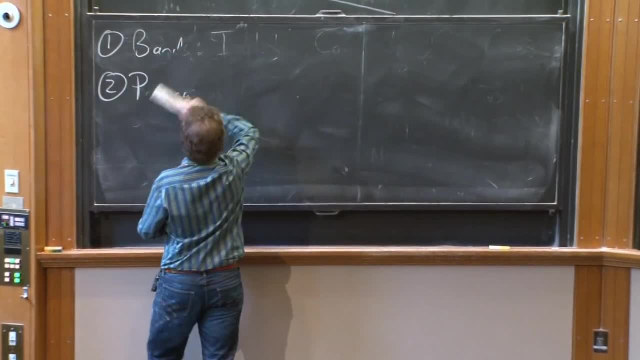 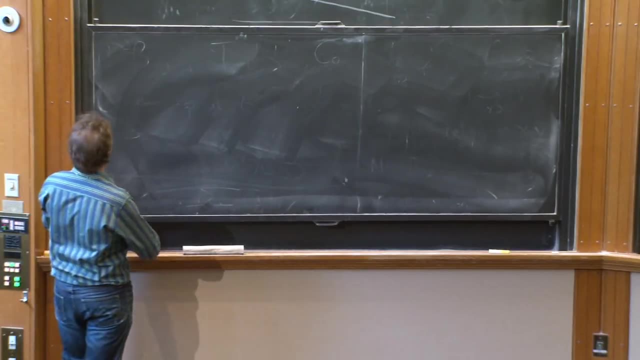 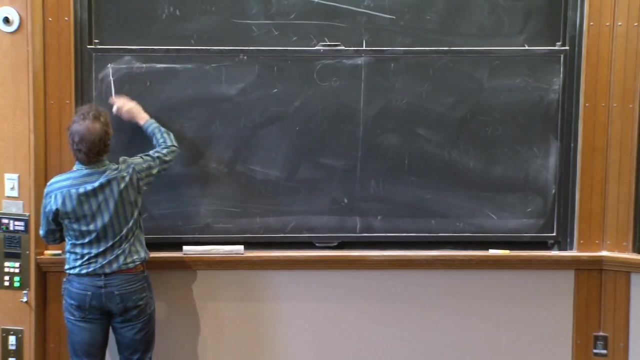 But that's OK. There are lots of questions and they were good questions, So this is going to be extremely brief. But I want to ask you the following question: What happens in the following three systems? So first, imagine we take a. let's. 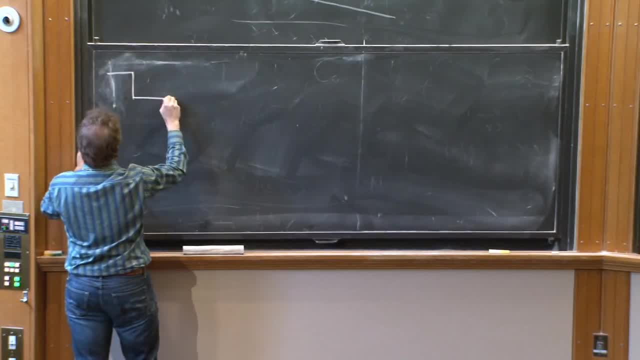 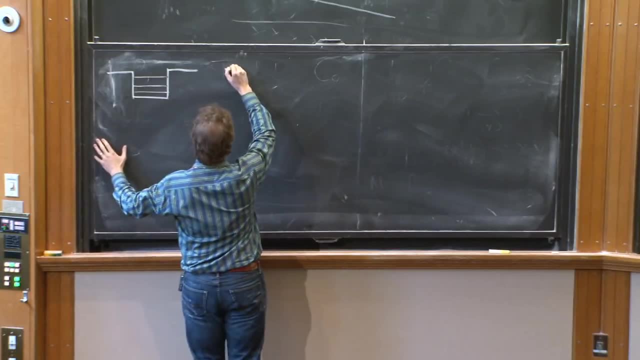 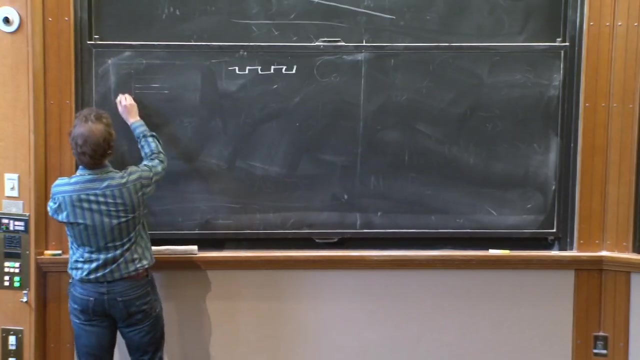 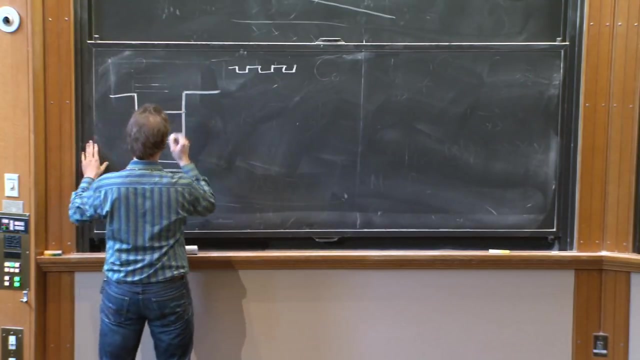 imagine we take a system built out of single wells which have some set of energy eigenstates, And then we build a periodic array out of them. What do we expect? And let me draw this bigger- What do we expect to see when we build a lattice? 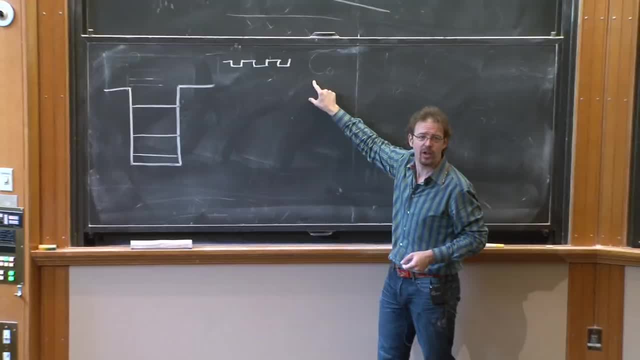 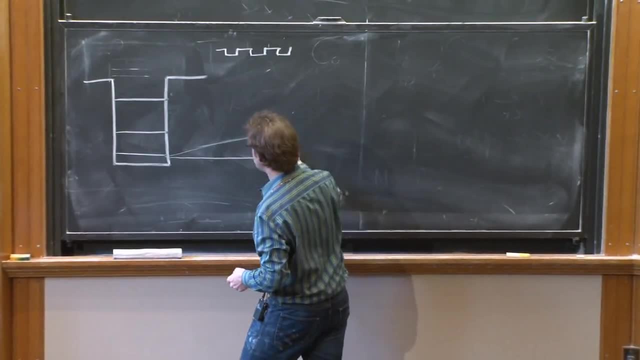 We expect that these states are going to spread out into bands. There's a finite width, And let's just talk about the 1D potential. So what we'll find is that this band turns into- or sorry, the state, the single state. 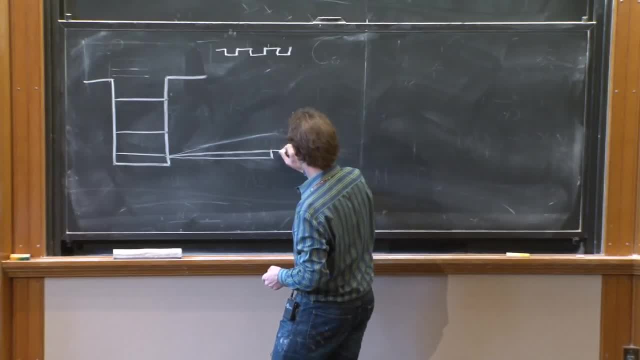 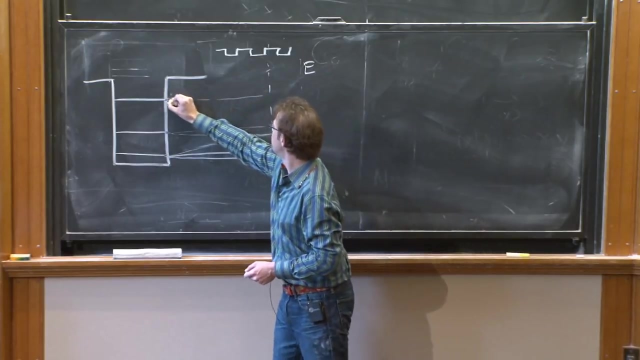 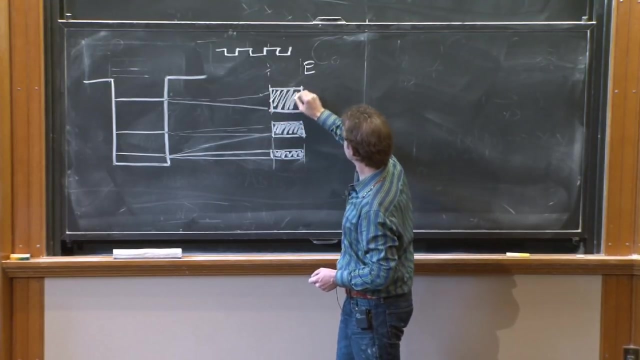 turns into a band of allowed energy eigenstates. This is now a plot of the energy And, similarly, this state is going to lead to another band with some width, And this state is going to lead to another band which is even wider. 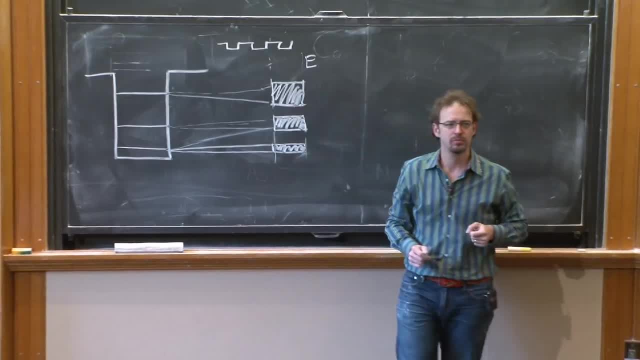 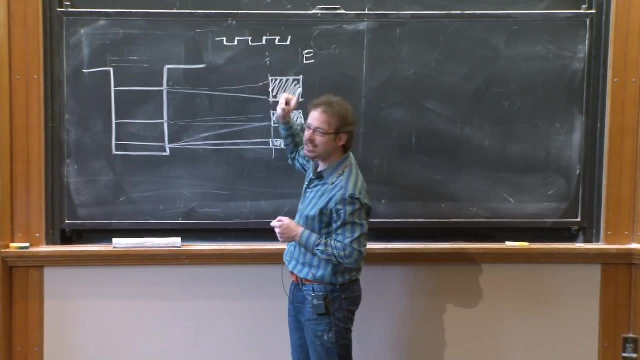 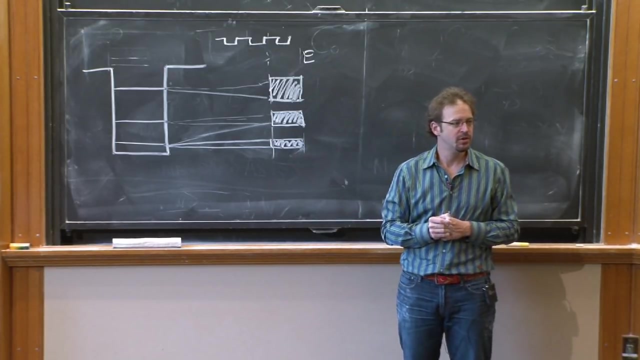 Everybody cool with that Quick question In 1D, do these bands ever overlap? No, by the node theorem. Now let's take a single electron. Let's put it in the system. What will happen? single electron fall into 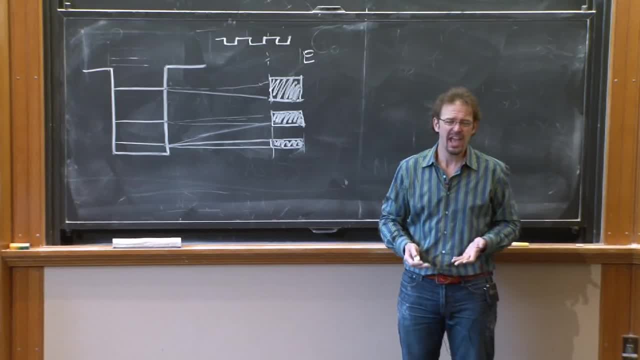 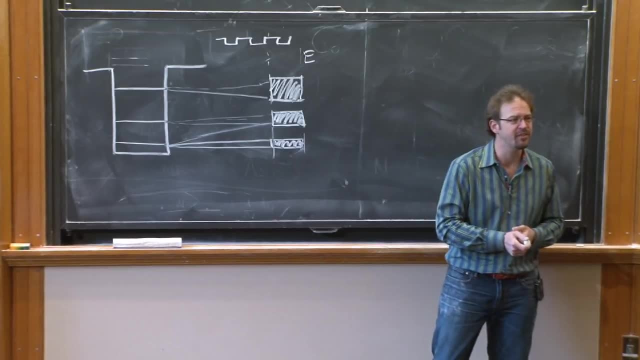 Yeah, one of the bands, but which state? Yeah, if you kick the system around you- let it relax a little bit- it's going to fall down into the ground state. You have to couple it to something else, like hydrogen has to be coupled to the electromagnetic field. 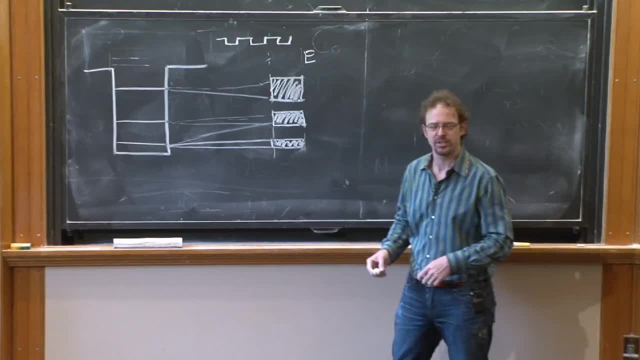 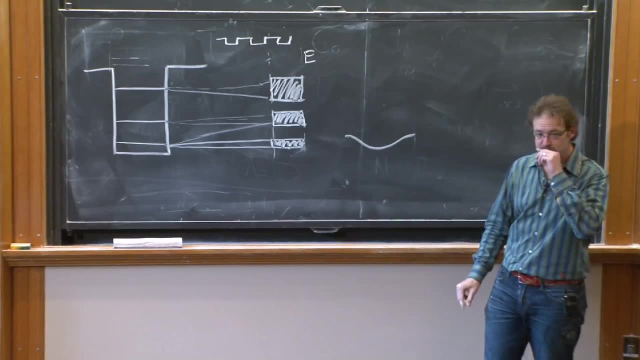 to decay, but couple it, kick it and let it decay And it'll settle down to its ground state. So you get an electron down here in the ground state And looking back at that band, we know that the band for that ground state looks like this: 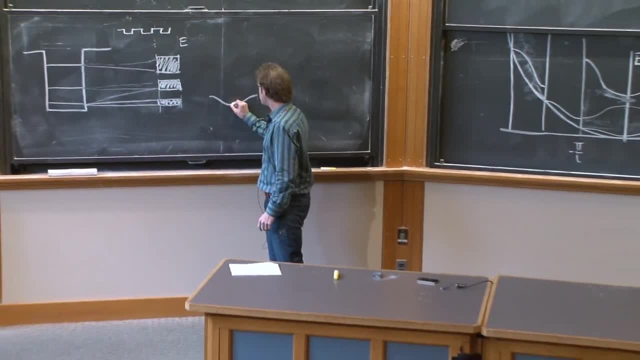 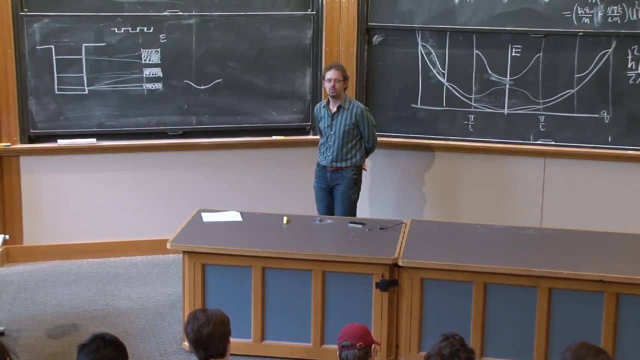 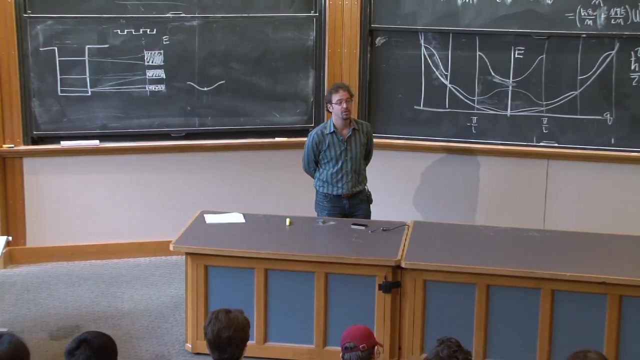 This guy. So here it is. There's our electron. It's sitting in the lowest energy eigenstate. Is it moving? Well, it's in a stationary state. It's the expectation value of the position changing in time? No, the expectation values don't change in time. 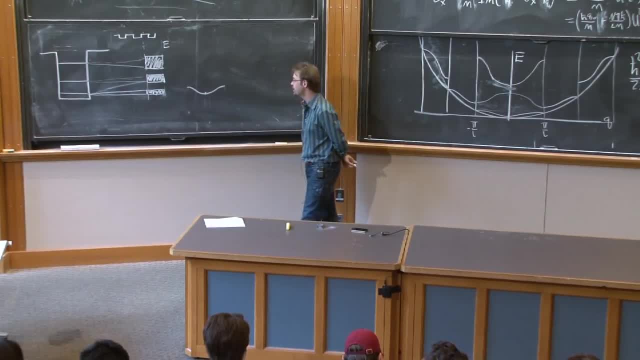 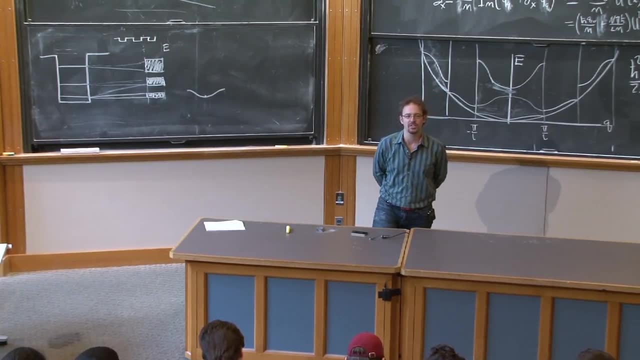 in the stationary state. That's part of what it is to be a stationary state, to be an energy eigenstate. OK, great, It's not moving. Now, in order to make it move, what do you have to do? What kind of state corresponds to the position changing? 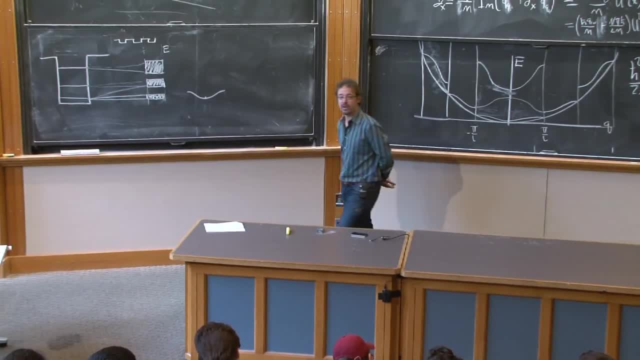 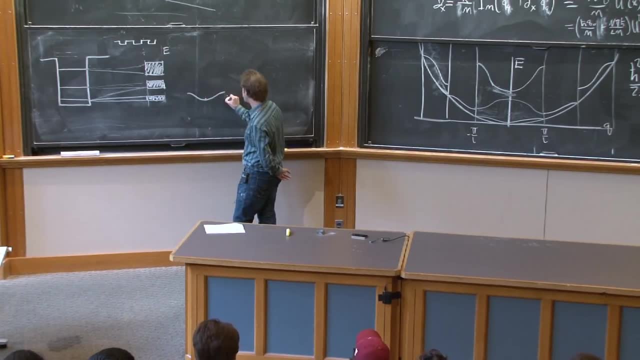 in time. Yeah, superposition, From the superpositions we'll get interference terms. So if we put in a superposition of, say, this state and this state, which corresponds to different energies, if we put it in a superposition of these guys, 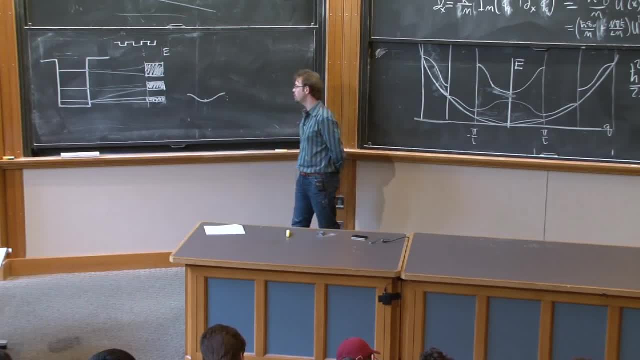 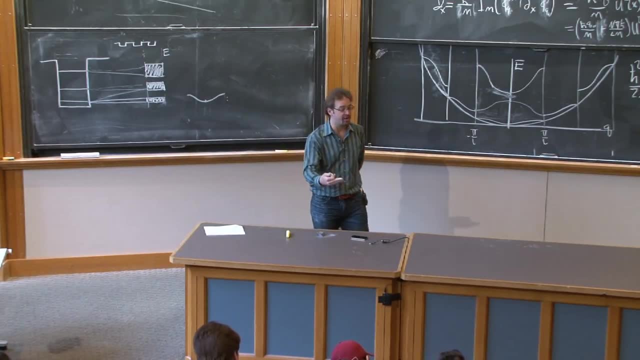 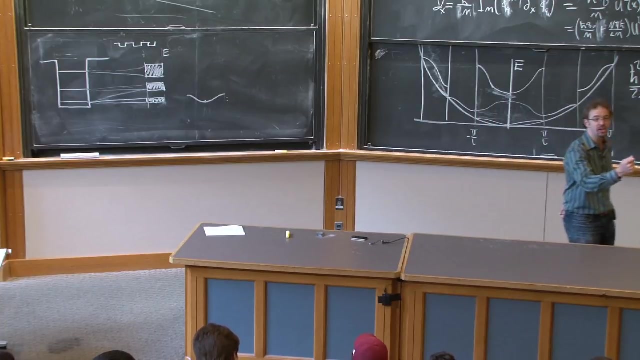 then it's meaningfully moving. It has a meaningful, well-defined time variation of its position, expectation value. So, in order to induce a current of this system where the electron wave packet carries a little bit of momentum, is changing in time its position. 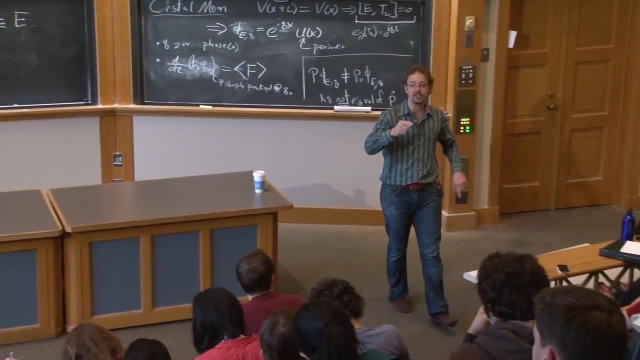 what do I have to do to the electron in the ground state? I have to excite it so that it's in a superposition of the ground state and some excited state or more generally, into a superposition of other states. Yes, 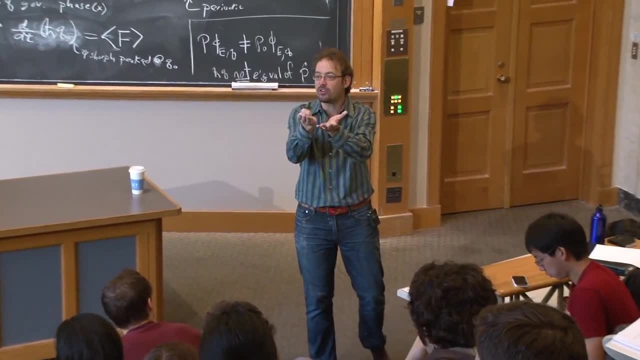 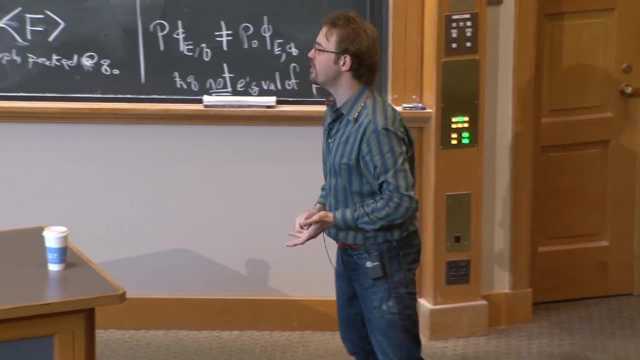 In order to induce a current, I must put the electron into a higher energy state and a particular superposition of higher energy states. Everyone down with that. Here's why this is so important. Imagine each one of these wells is actually not some square well. 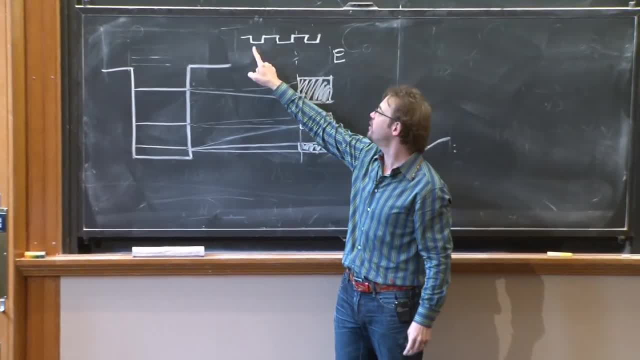 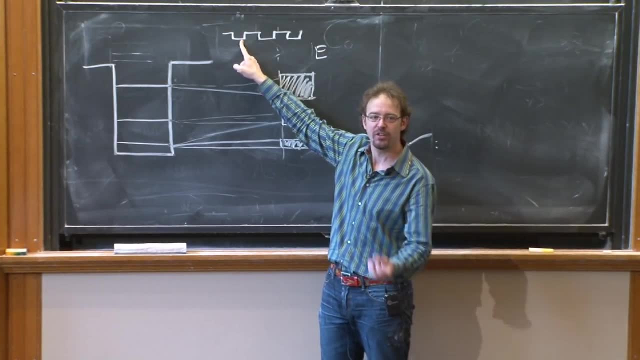 but it's an atom, And let's say the atom is hydrogen. just for you know, this doesn't actually happen, but just imagine In particular. what I mean is it has the ion. the nucleus is charged plus 1.. 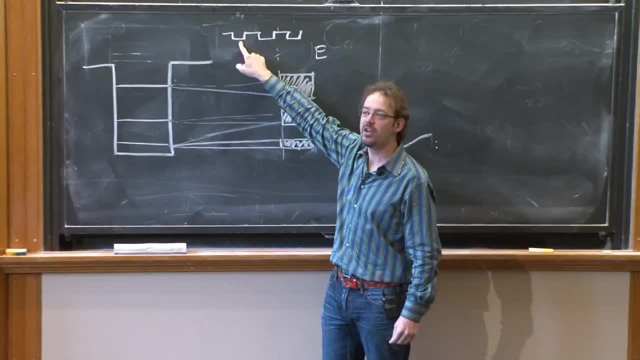 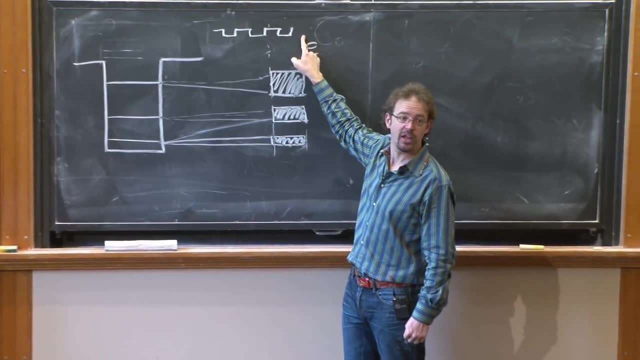 And so in order for the system to be neutral, I must have one electron for every well. So if I have n wells I must have n electrons in the system- Everyone agree with that- In order to be neutral, Otherwise the thing's charged and all sorts of terrible things. 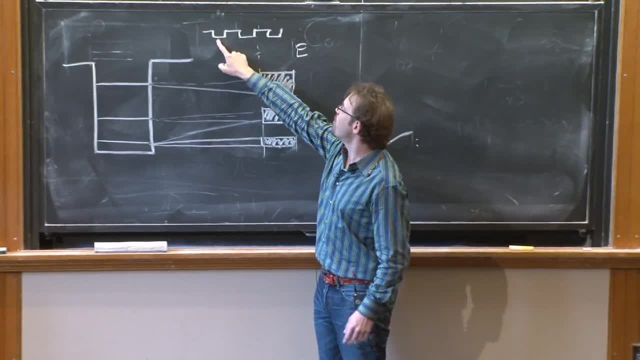 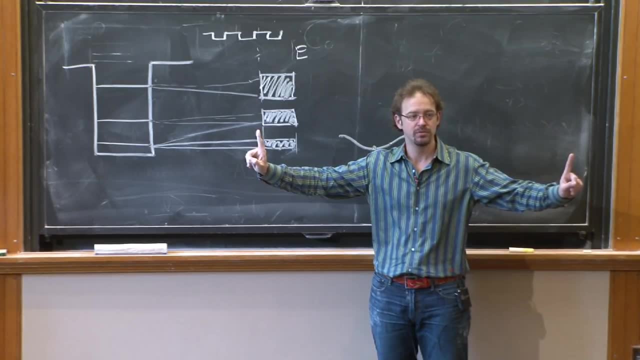 You know electrons will get ripped off of nearby CAD, So we must have an electron per well. How many states are in this band for n wells n Right? So if I put in the n electrons I need to neutralize the system. 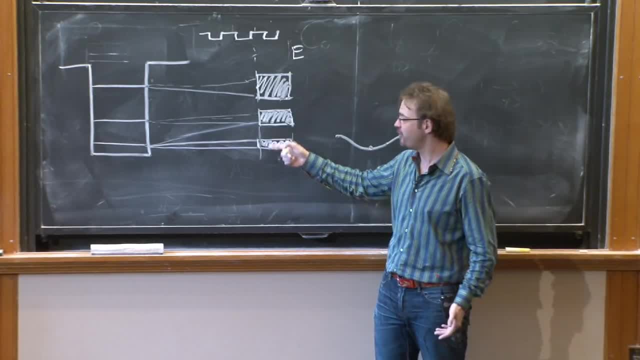 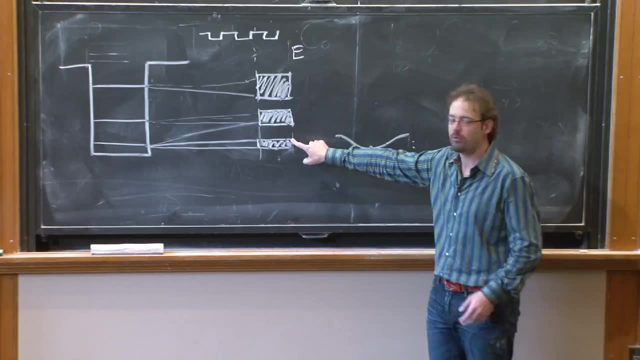 where do those n electrons go? Yeah, they fill up the first band And if we let the system relax with lowest energy configuration, every state in this lowest band will be filled and none of these states will be filled. Everyone down with that. 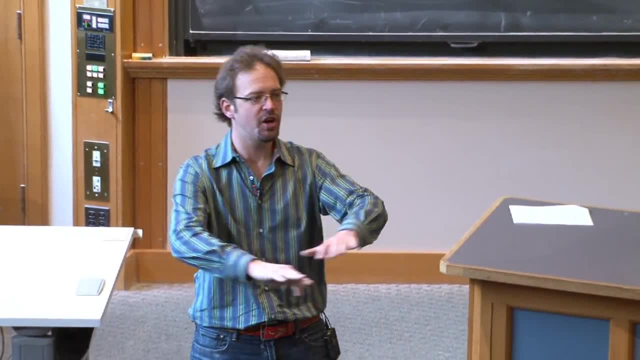 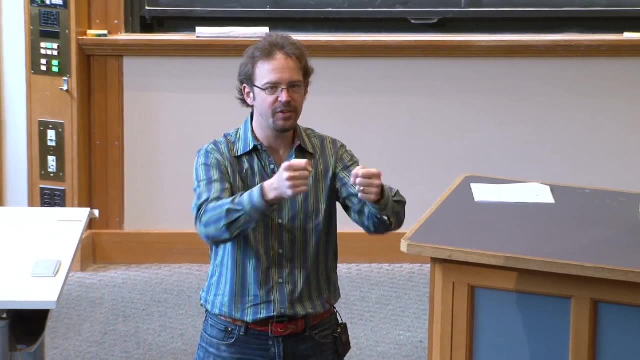 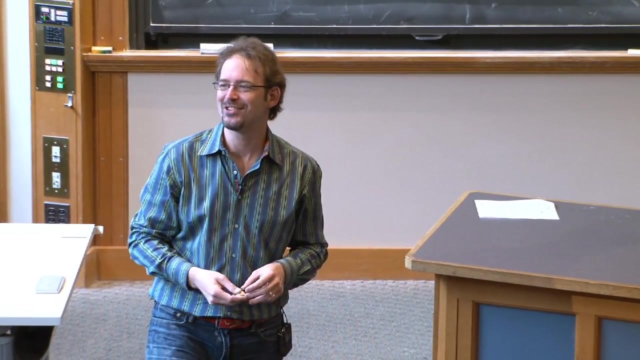 So here's my question: When I've got that ground state configuration of this lattice of atoms with one electron per well in these distributed wave functions filling out these bands, is anything moving? Wow, you guys are so quiet today. Is anything moving? 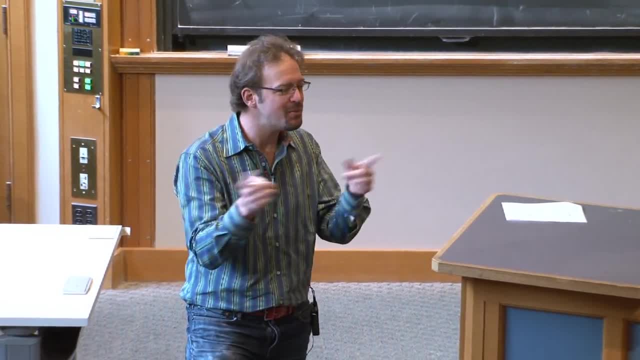 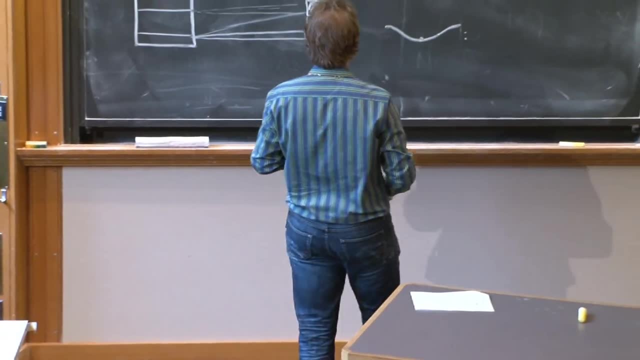 The system is in an energy eigenstate. In particular, it's in a completely anti-symmetrized configuration because they're identical fermions. So nothing is moving. OK, So nothing is moving. If we want to induce a current, what do we have to do? 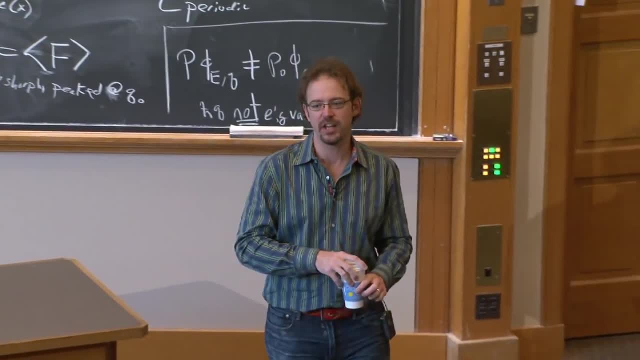 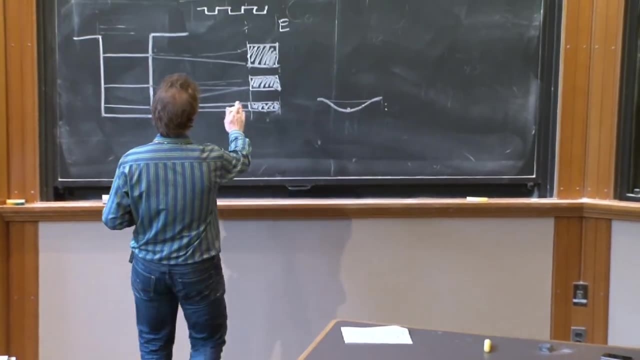 Yeah, we have to put them in a superposition, But where's the next allowed energy eigenstate, Next band? So it's in the next band. It's the next allowed energy eigenstate. So the configuration we have now is that these guys are all filled. 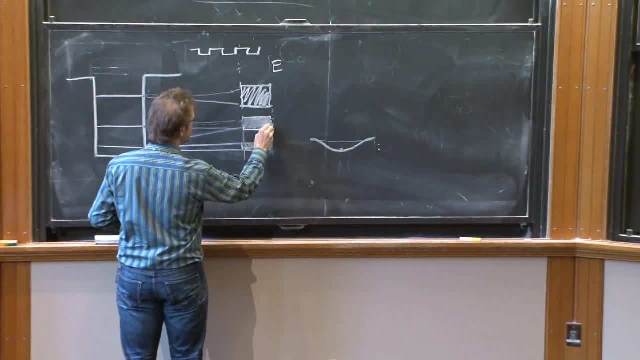 These guys are all empty, But in order to take an electron from here and put it into this excited state, we have to put in a minimum amount of energy which is the gap between those two. OK, So we have to put in a minimum amount of energy which is the gap between those two. 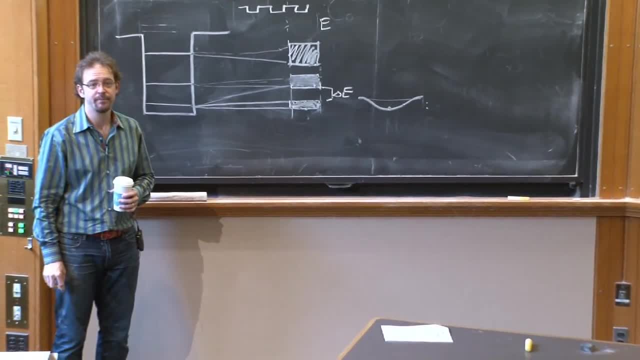 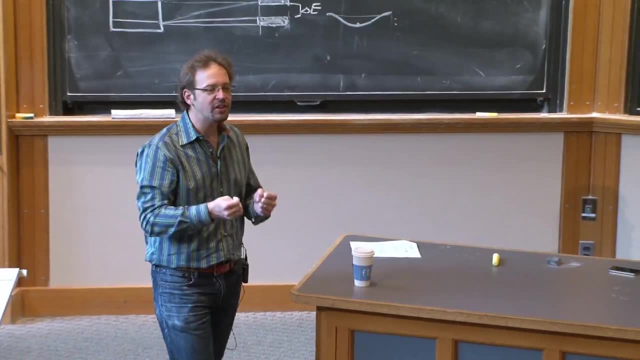 OK, So we have to put in a minimum amount of energy, which is the gap between those two bands, Right? So now think about it this way: Suppose I take light and I send my light at this crystal, In order for the light to scatter off the crystal. 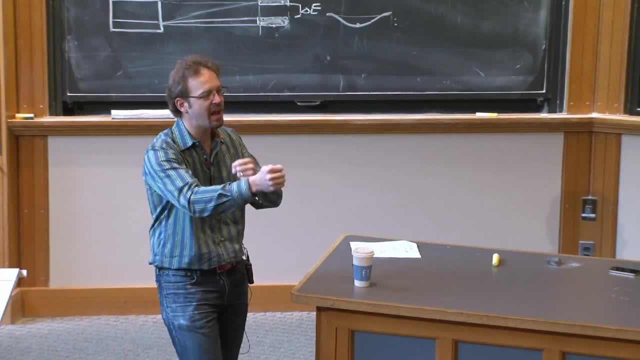 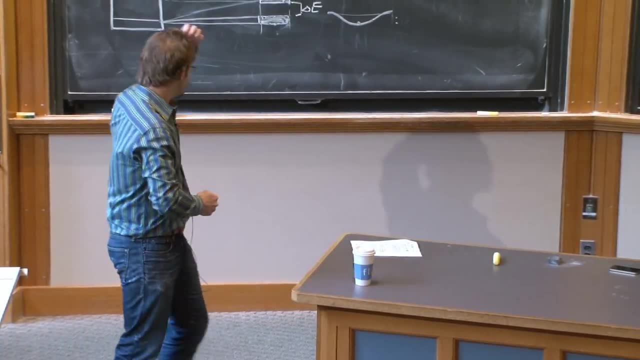 you must have electrons in superposition states so that they can have a dipole and absorb and radiate that energy. Yeah, But in order for that to happen, the light has to excite an electron across the gap. It has to give it some energy. 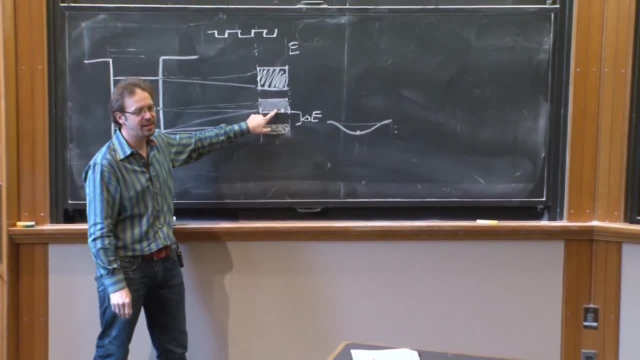 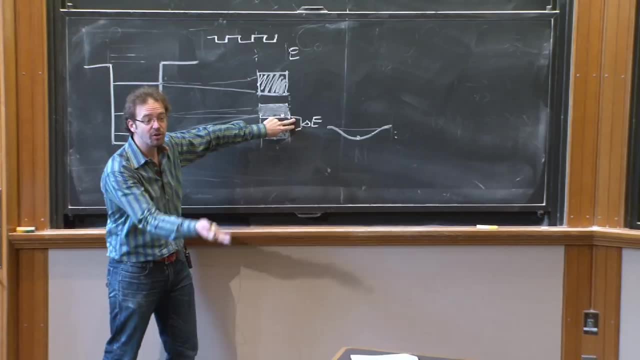 It has to give it this macroscopic amount of energy. Well, it's not macroscopic. it's large. It's not infinitesimally small. That means that there's a minimum amount of energy that that incident light must have in order. 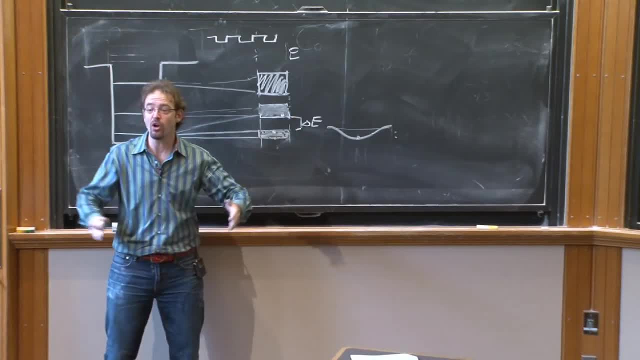 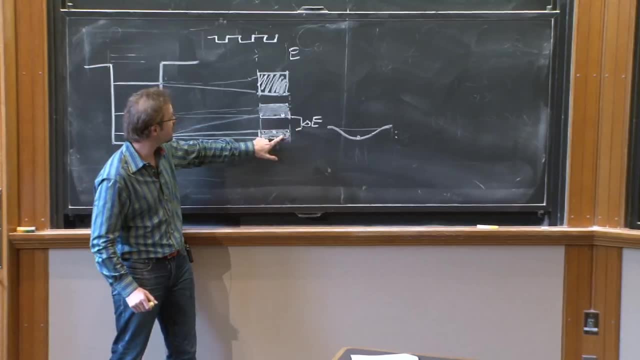 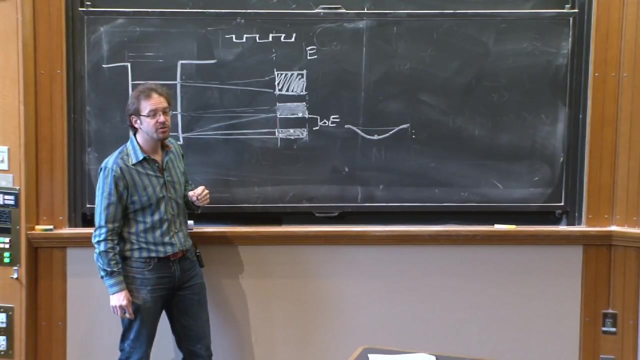 to excite the electron in the first place. So very long wavelength light will never do that. Light of long wavelength will not have enough energy to excite an electron across this gap into the next band to allow there to be a current which could oppose the electric field. 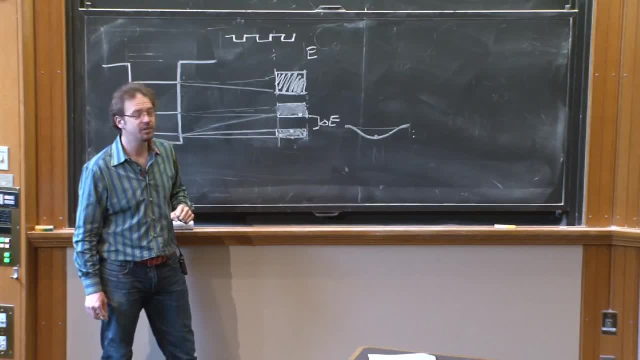 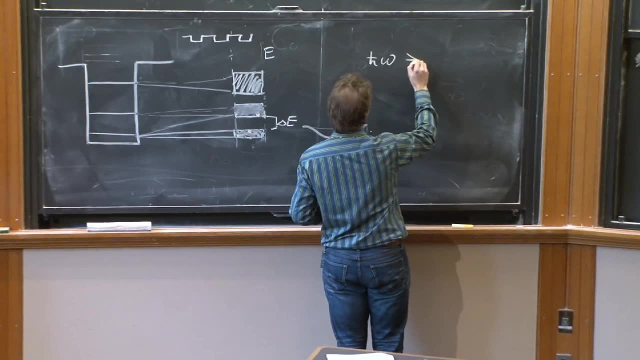 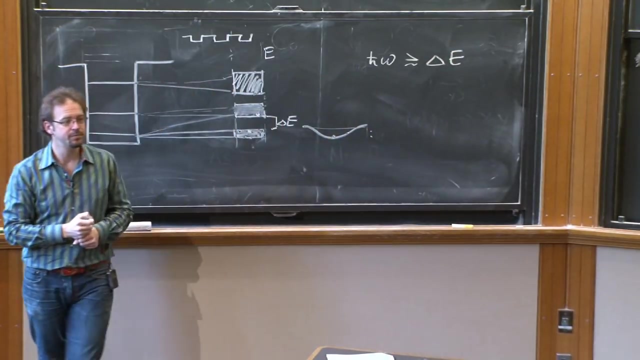 So the only way for light to scatter off of this crystal is if the energy h bar, omega of the light- is greater than or equal to. well, let's just say greater than or approximately the band gap delta E. Is that cool? 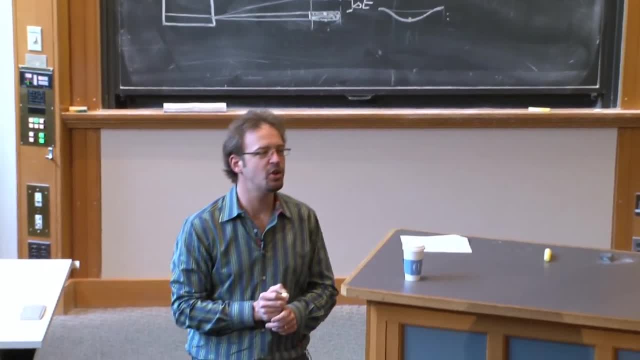 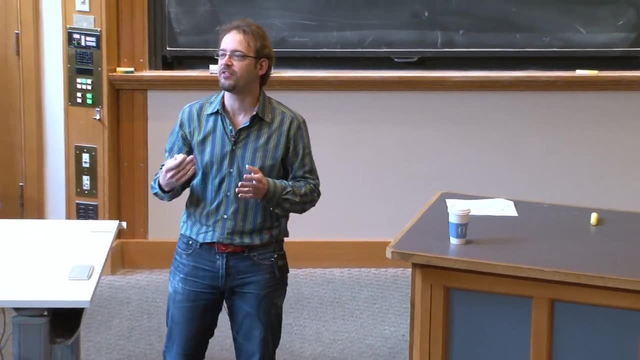 We've just discovered something: Crystals are transparent unless you look at sufficiently high frequencies. That's cool, right? A crystal is transparent unless you look at sufficiently high frequencies. If you look at low frequencies, there's no difference. Your crystal should be transparent. 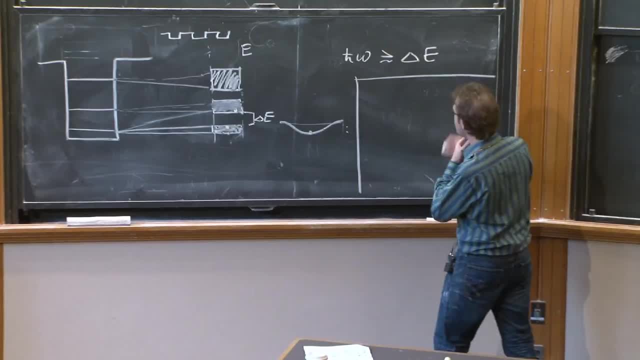 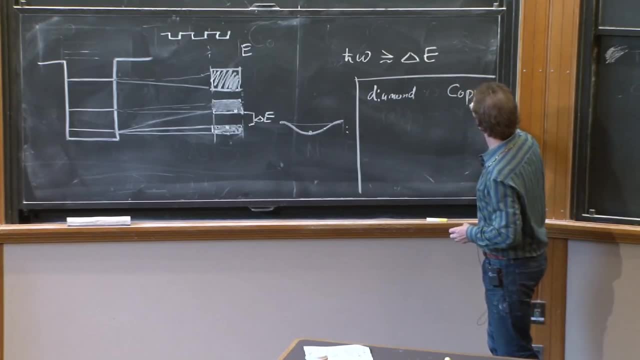 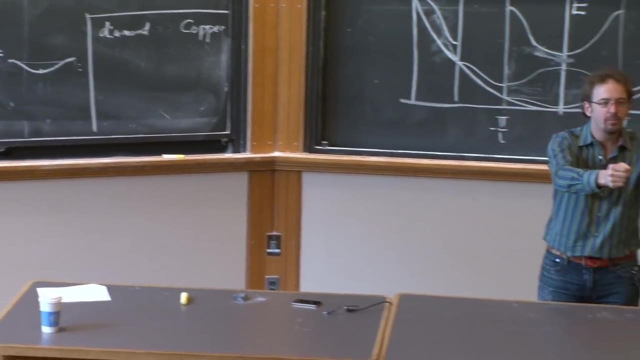 Well, that's really interesting. In particular, we immediately learned something cool about two different materials. Consider diamond and copper. These are both crystals. They're solids made out of a regular array- perhaps not perfect but extraordinarily good- regular array of atoms of the same kind arrayed. 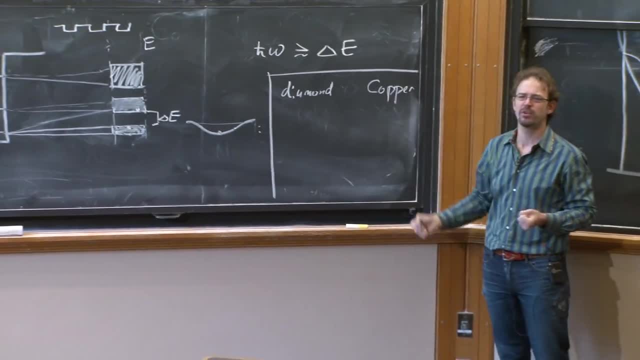 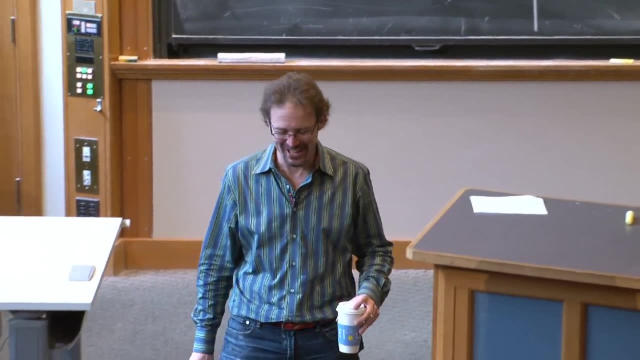 in a particular structure: diamond and, I think, face-centered cubic, I don't remember. I really should know that. Anyway, copper, it's a lattice, So that's embarrassing. I really should know that. So we have these two materials. 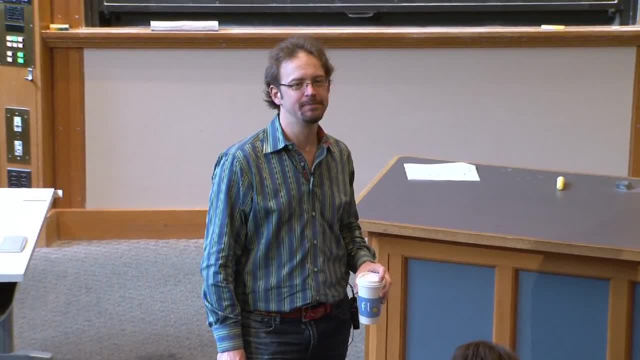 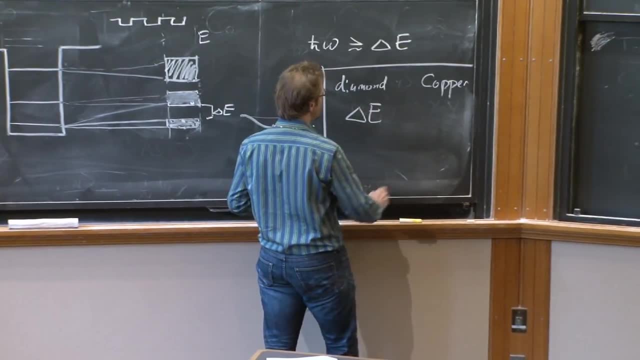 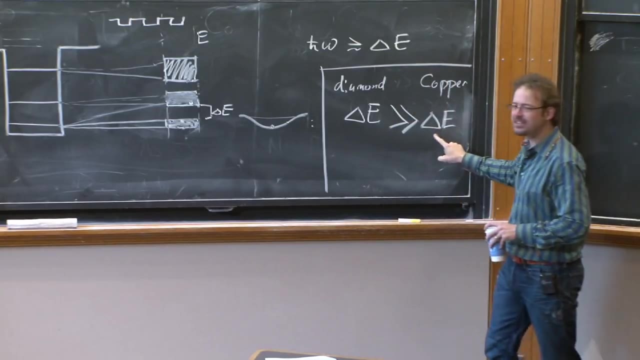 Which one has the larger band gap: Diamond, because it's transparent in the visible. So the band gap delta E of diamond is much larger than the band gap for a copper, But in fact This is a little more subtle because copper in fact 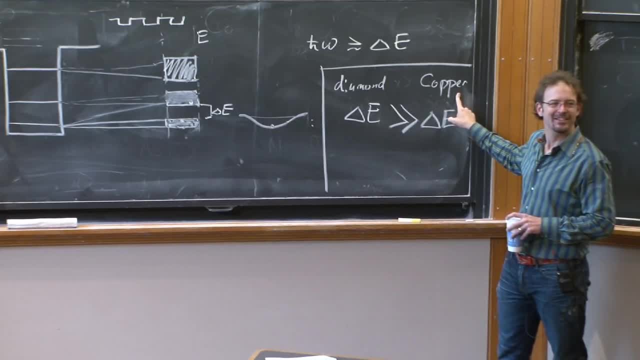 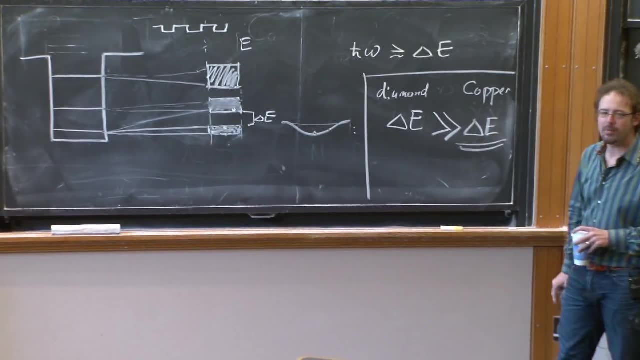 doesn't even have a band gap. Ah, we made an important assumption here, So I want to think about. we're going to come back to copper in a second, But I want to point out the nice thing here, which is that diamond has to have a band gap. 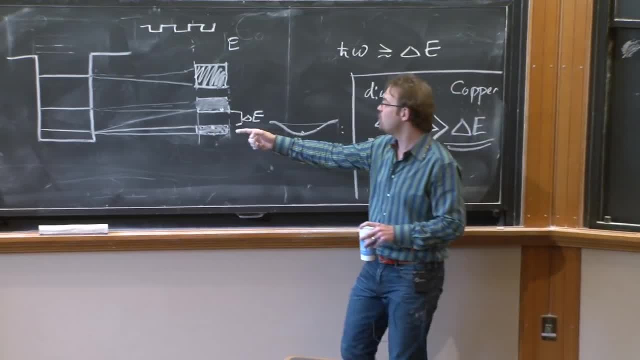 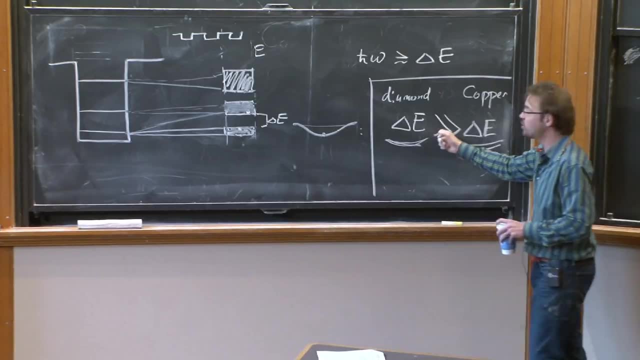 It's transparent, It must have a band gap. It must be such that when you fill up all the electrons you need for it to be neutral, there's a gap to the next energy states. And that gap must be larger. It must be larger than visible wavelengths of light. 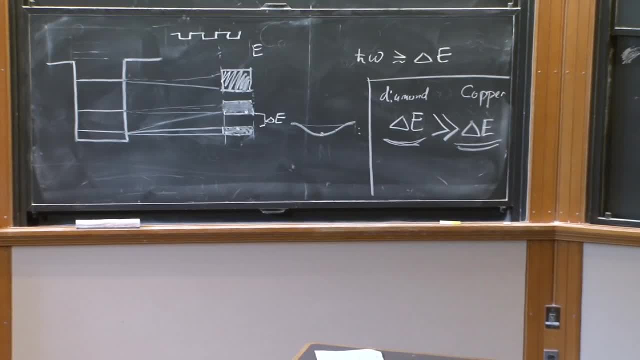 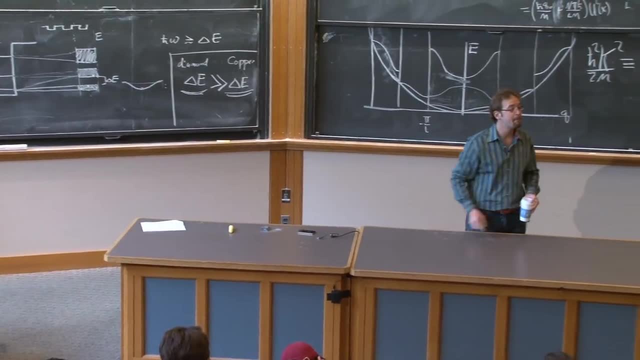 That's cool, And that must be true of all the transparent crystals that you see. Otherwise they wouldn't be transparent. They would respond by having free electrons that could respond like a metal. Yeah, So this means that the original diamond material should not be conductible to the sun. 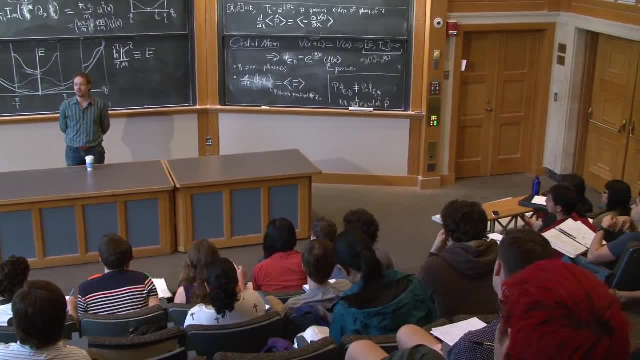 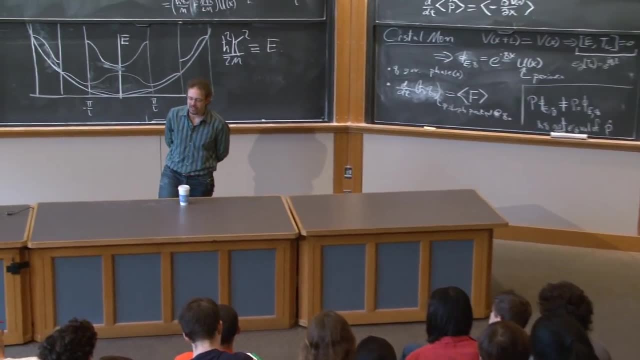 Yeah, Are diamonds good conductors? No, they're terrible conductors. In fact, they're preposterous Preposterously. If you compare the number of- well, OK, I'll get into this later, But yes, they're terrible. 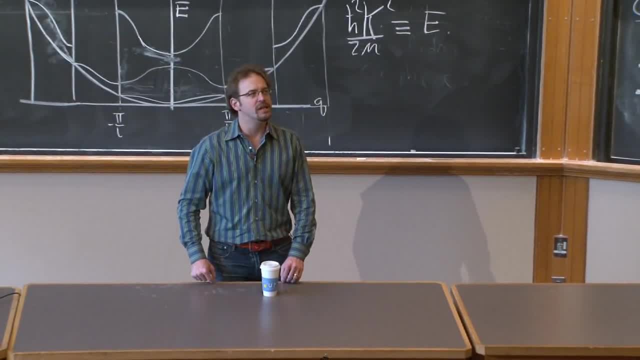 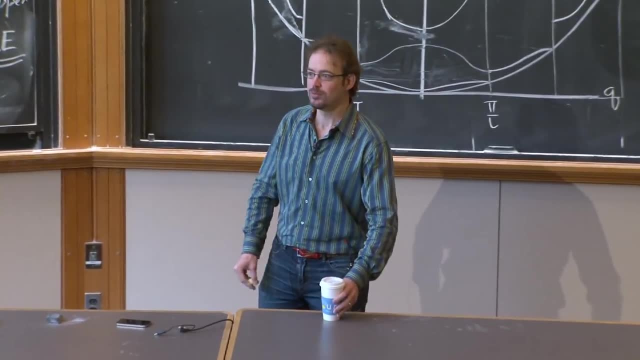 Also, why are those metals are gray? That's a slightly more complicated story which let me come back to Hold on to that, And if I don't answer it today, ask me after an office hours, because it's a little more. 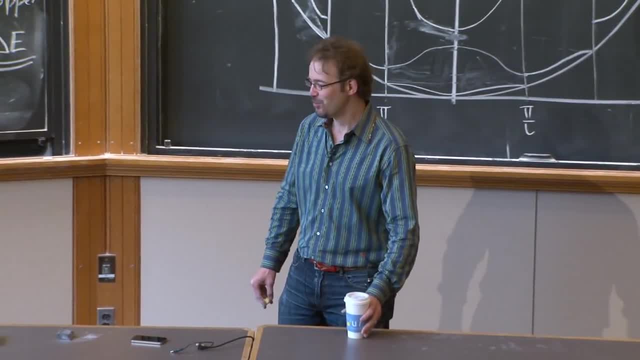 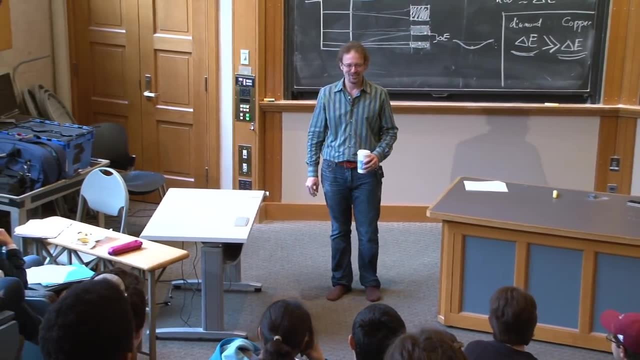 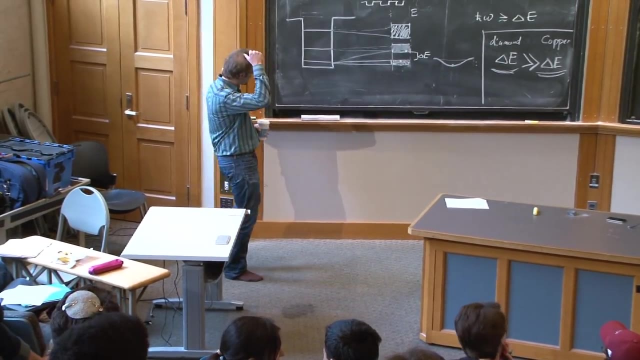 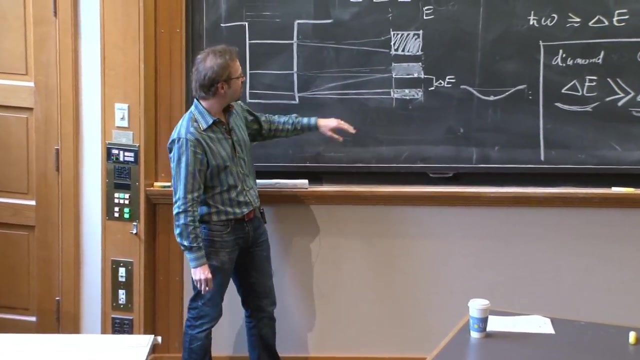 What Really Wow. Well, MIT, OK, It's all about the intellect And everything else has to wait. So this is pretty good. But here's the thing: In one-dimensional crystals, the only thing that can happen is: look, if you have, each band comes from an allowed energy.